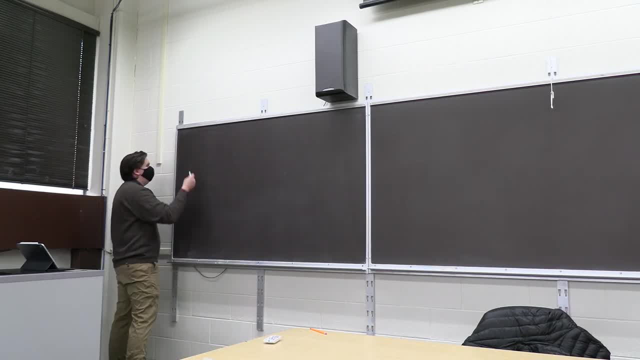 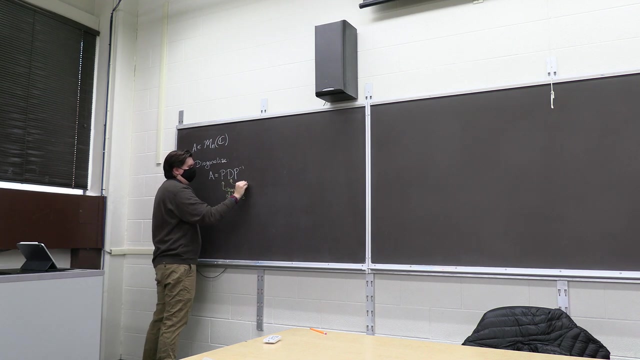 So last time we mentioned that if we have a matrix with complex entries- so let's say it's an n by n complex matrix- we can always diagonalize the matrix, That is, we can write it of the form: A equals PDP inverse, where P is our change of basis and D is a diagonal. 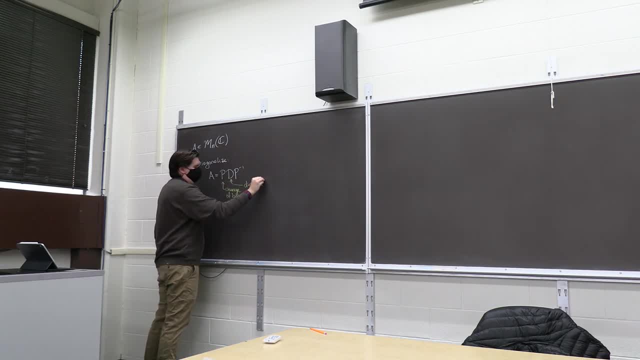 matrix with eigenvalues along the entries right. So the columns of P are eigenvectors and the eigenvalues along the entries right. So the columns of P are eigenvectors and the values of D are your eigenvalues And you have a little bit of freedom in which. 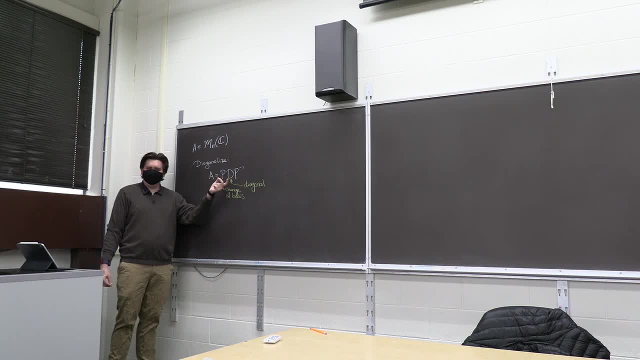 eigenvectors you pick right Because you may have some eigenvalue. you know there's a whole, you can scale by whatever, but you may have, like, some eigenvalue. you should have multiplicity two and you just want to pick any two vectors that span that two-dimensional. 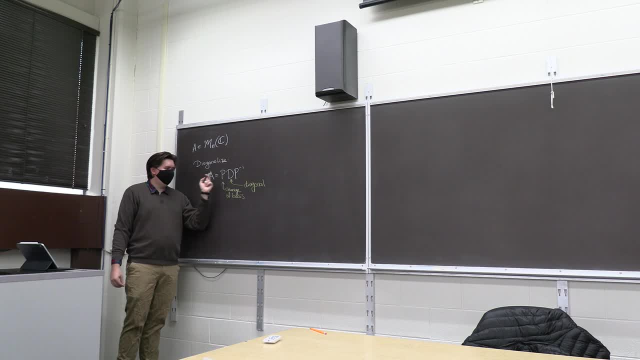 subspace, right. So there's some freedom in which P you pick here. but it gives us a way to rewrite A in terms of some diagonal matrix. And then we said, well, what if we want to insist that that P is a unitary matrix? right That eigenvectors? 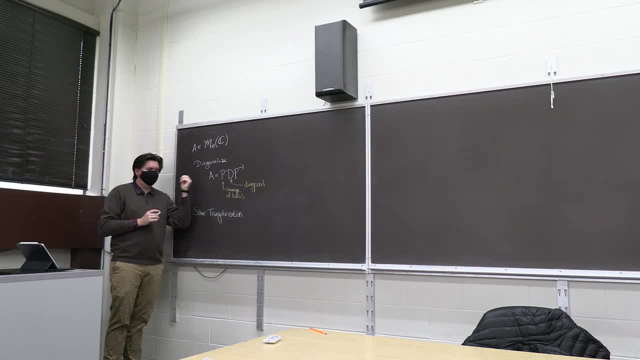 are chosen in such a way that they're an orthonormal basis. Well, you can try and do that, but you maybe won't always be able to find such a. In particular, your D may not remain a diagonal, but you can always find a unitary matrix U. 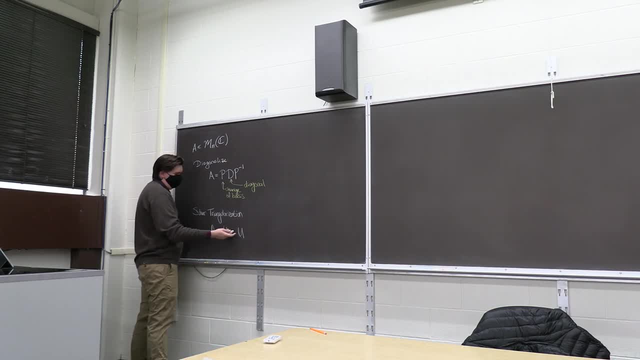 if you relax the condition on the center matrix to be an upper triangular matrix. So now U is unitary, so U inverse is just the conjugal Didier Francis formula, Inaugural and now transpose of U. So here U is some unitary matrix, and thus that explains why U 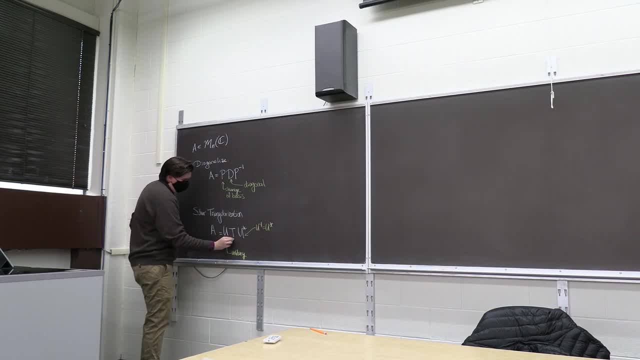 inverse is just U conjugate transpose and T is an upper triangular matrix. Okay, so now you have an orthonormal basis, an orthonormal change of basis. you can think of it as Aren't necessarily all eigenvectors, because T isn't just. 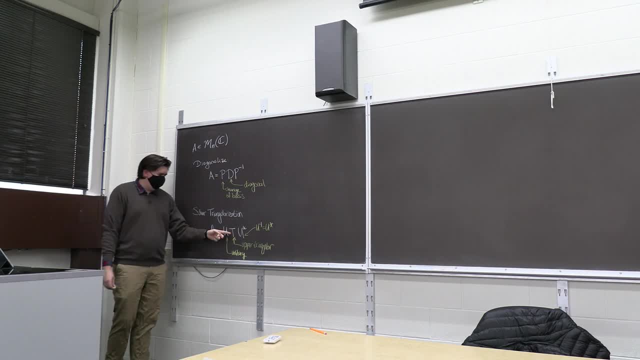 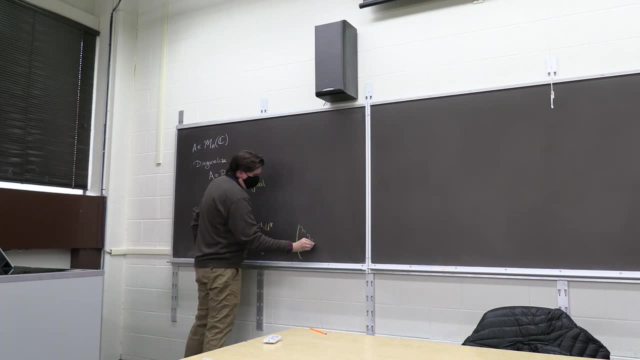 eigenvalues along the diagonal. It's a little more complicated than that. It is still eigenvalues along the diagonal, but you may have other stuff above it. You could have whatever up here and then you know zeros down here. So this is not necessarily just a collection of eigenvectors, It's just 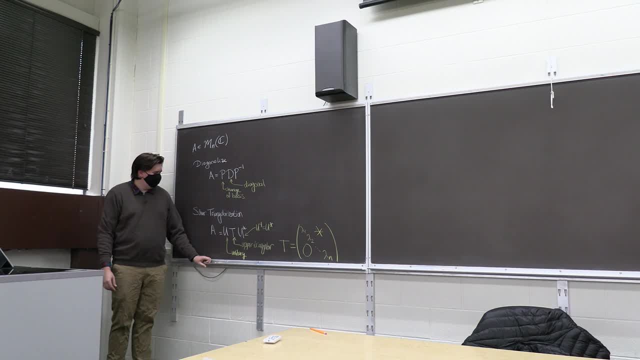 some orthonormal basis That's doing something kind of similar, but you have a different matrix in the middle. Okay, so why might we want to be able to? why might we want to be able to do this? Well, doing this, let us prove lots of nice properties right From this. 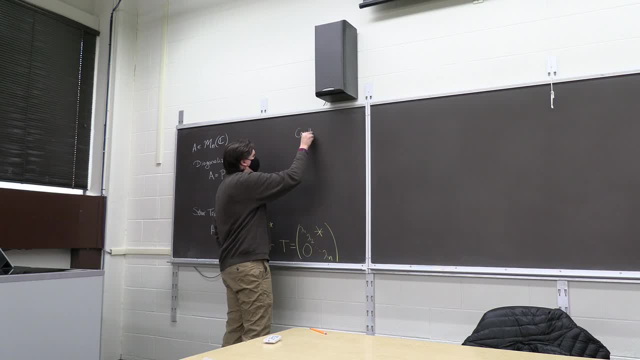 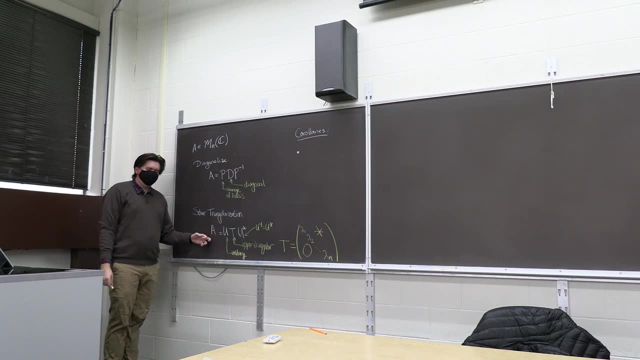 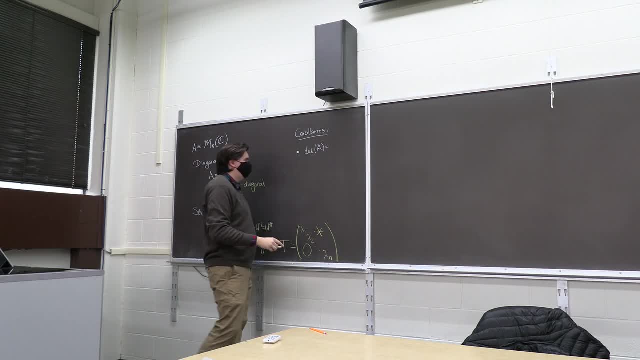 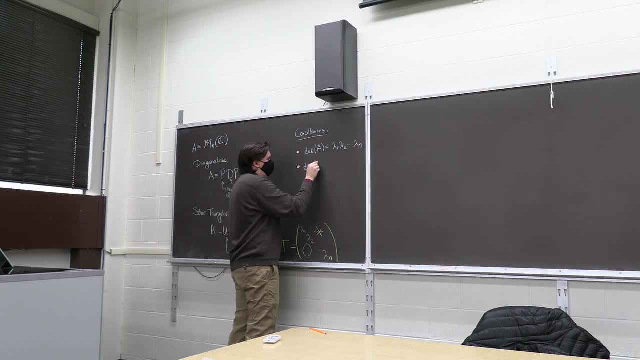 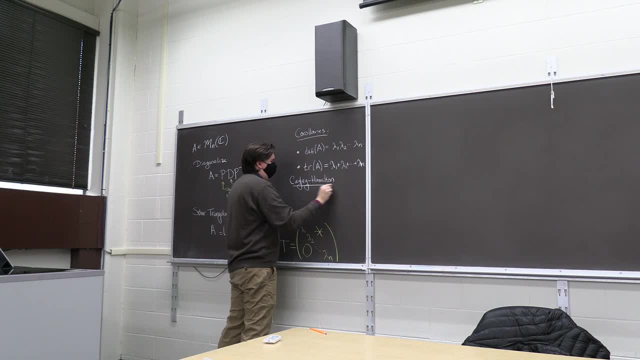 theorem which states that if we denote the characteristic polynomial of A as PA lambda, so if this is a characteristic polynomial, characteristic polynomial, then if you plug A into it you recover zero. You already know that if you plug an eigenvalue into here, you get zero. But now I'm saying, if you plug a matrix into the polynomial you get zero. 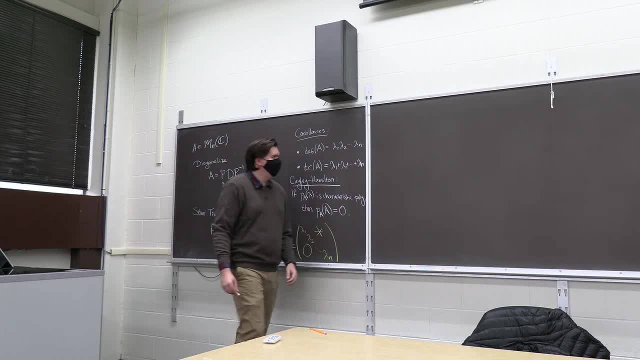 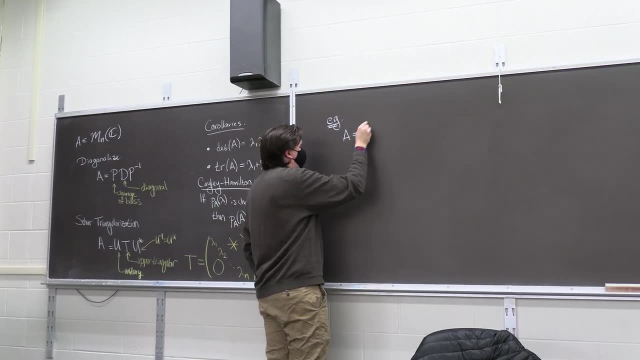 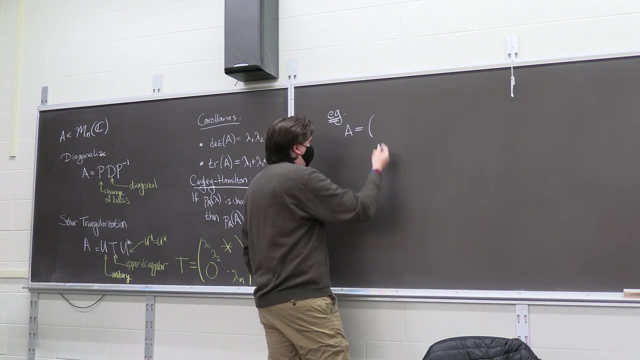 So what do I mean? plugging a matrix into a polynomial? What's going on here? Let's just look at a quick example. So let's take some matrix A, I don't know. Let's pick a nice one. You can pick whatever you want. Let's call it 1,, 2,, 3,, 4.. 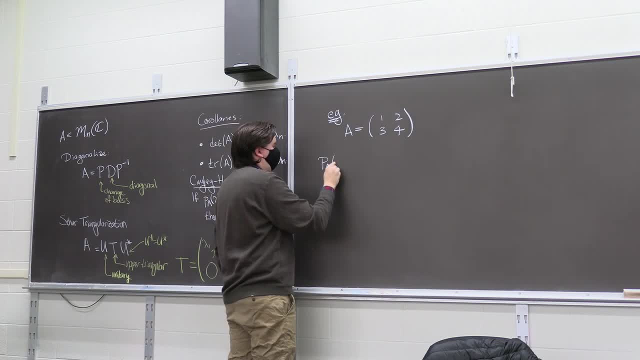 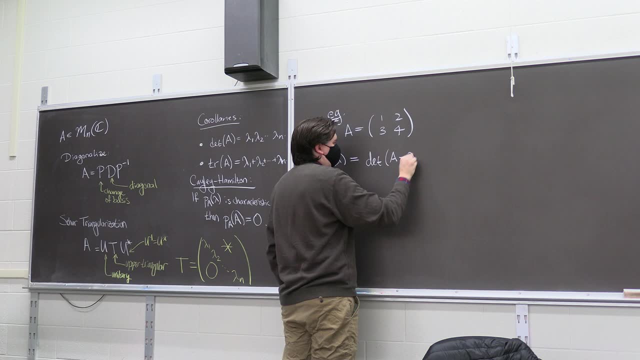 What is the characteristic polynomial of A? Well, recall that's just defined to be the determinant of A minus lambda. I So that's just the determinant of 1 minus lambda, 2,, 3,, 4 minus lambda, Which is just the product of these guys, which is lambda squared minus 5 lambdas plus 4.. 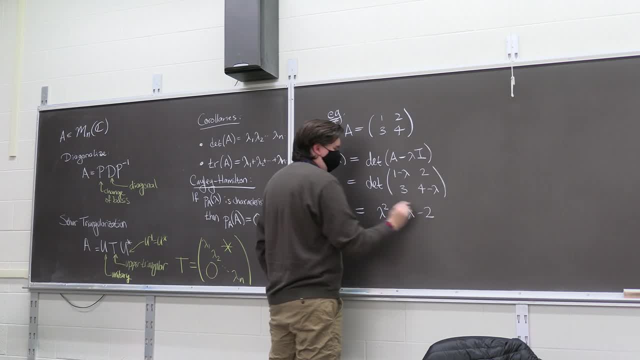 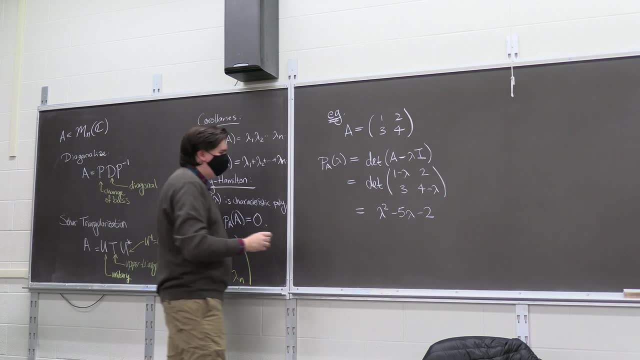 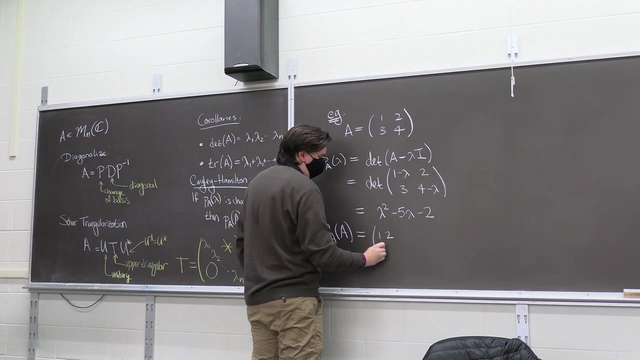 But then you're going to be subtracting 6,, so minus 2.. I think that's my characteristic polynomial. So what is the characteristic polynomial? plugging in A plugging in a matrix? Well, that would be plugging your matrix 1,, 2,, 3,, 4, squared. You know how to square a matrix. 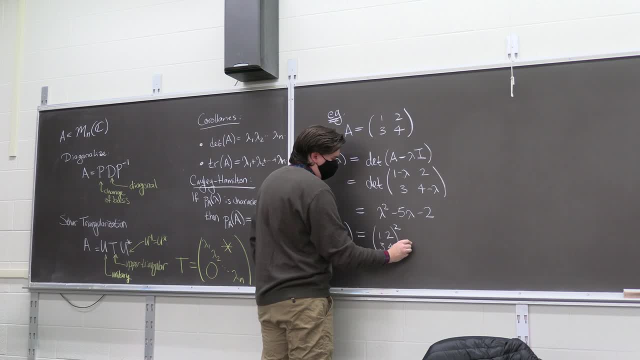 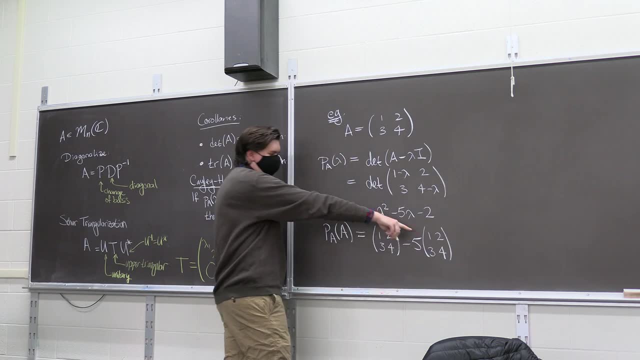 That's just multiplying the matrix by itself, Minus 5 times the matrix. We know how to scale a matrix by 5, so that's not a problem. And then minus 2.. And it's like: well, what does minus 2 mean? 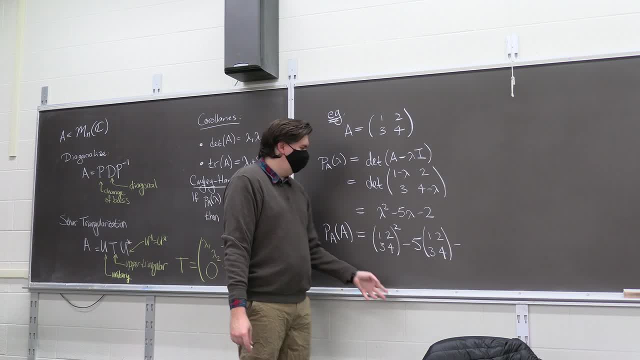 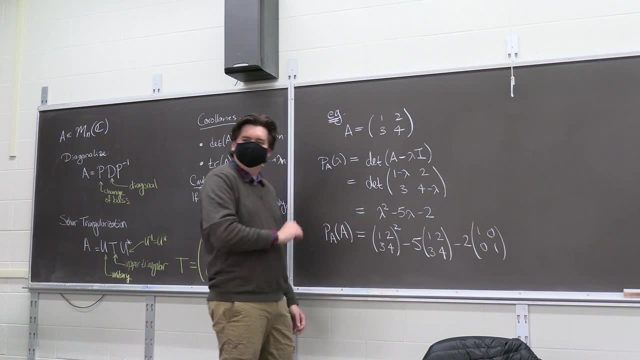 You can't just put a 2 here. Well, the analogous thing would be just to say 2 times the density, right? You think of this 2 as like 2 times 1, so in terms of matrices, that's 2 times the density. 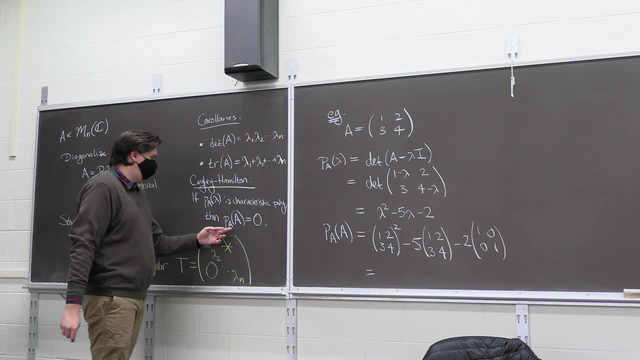 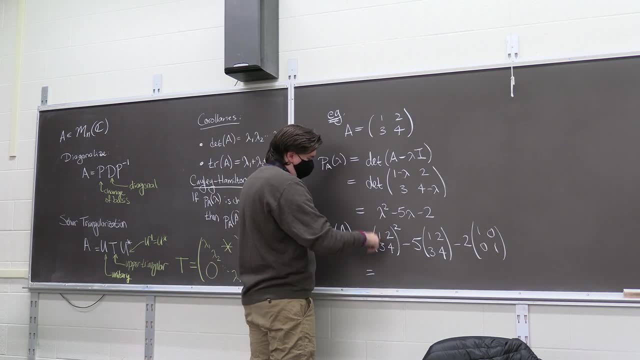 And let's just verify that indeed it does as it should. According to Cayley Hamilton, this should come out to be 0.. So let's check. So here we get, row times column. You guys can help me out? I think this is a 7 in the upper left-hand corner. 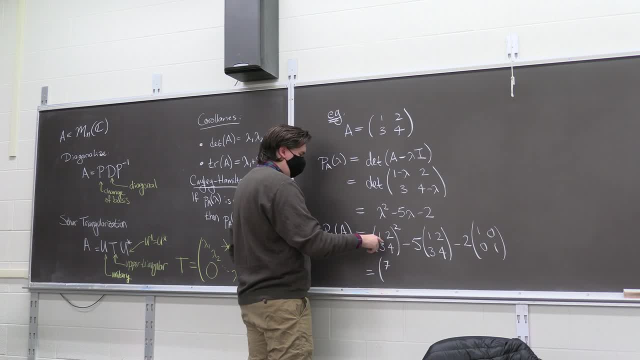 So here we get row times column. You guys can help me out. I think this is a 7 in the upper left-hand corner. Row times column is 8 and 2, so that's 10.. Row times column is 12 and 3, so that's 15.. 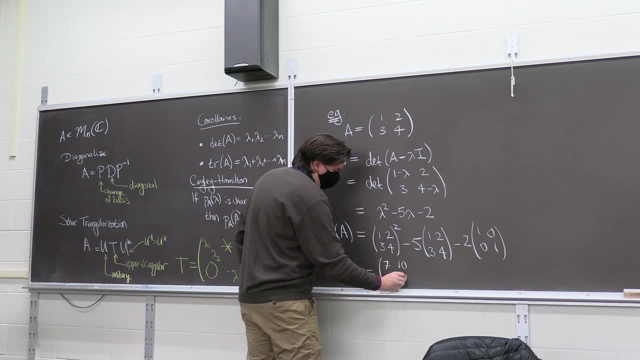 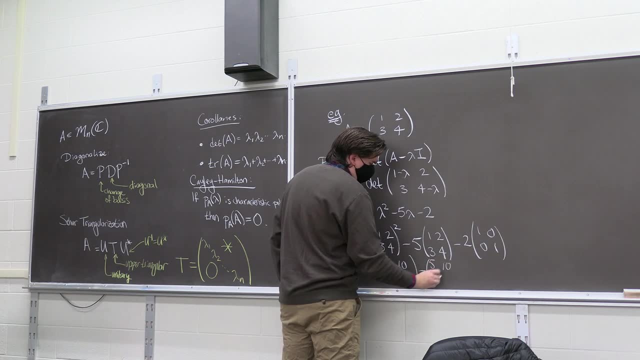 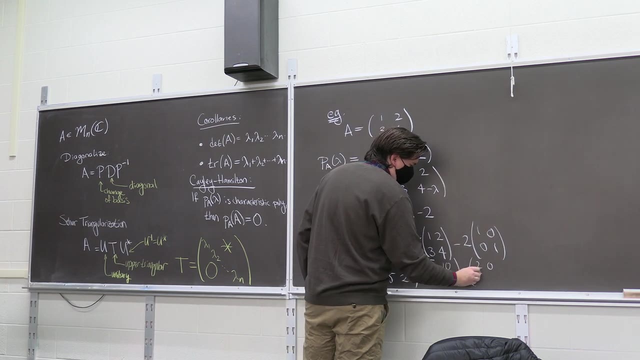 Row times column is 6 and 16,, so that's 22.. Does that look good? Minus 5,, 10,, 15, and 20.. And then minus 2,, 0,, 0,, 2.. 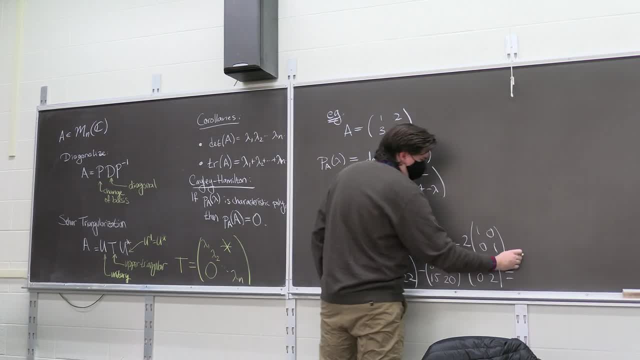 And let's just check really fast: 7 minus 5 minus 2 is 0.. 10 minus 10 minus 0 is 0.. 15 minus 15 minus 0 is 0. And 22 minus 20 minus 2 is 0.. So we recover the 0 matrix. 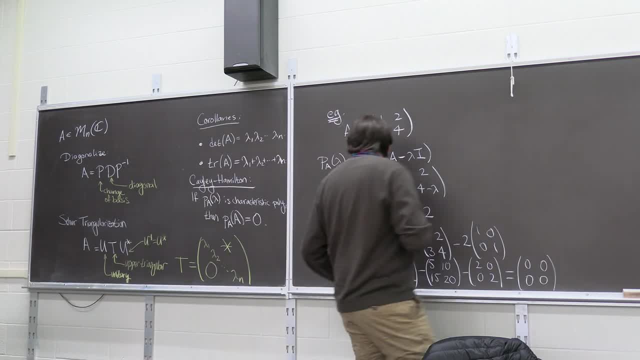 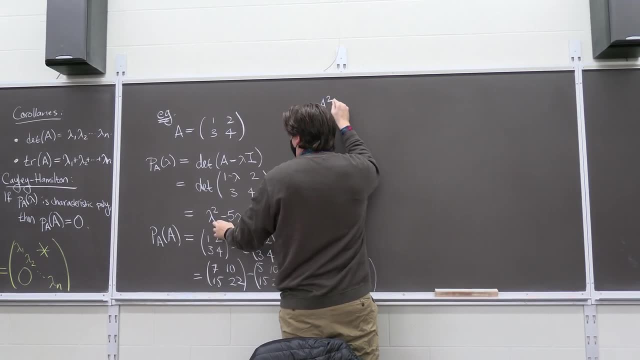 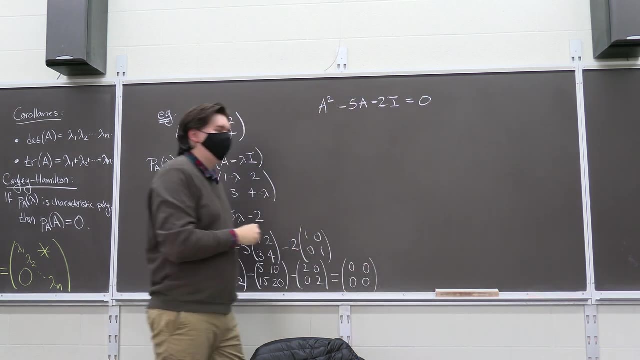 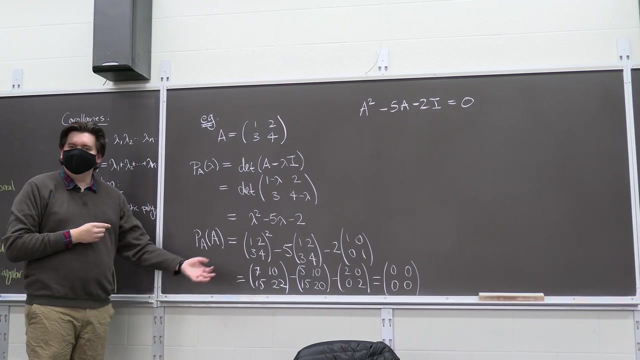 So that's what I mean when I say that this is 0.. That is, I'm saying that a squared minus 5a minus 2 times the density gives you the 0 matrix. Okay, this might just seem like a nice little trick, but there's actually some really nice applications of this right. 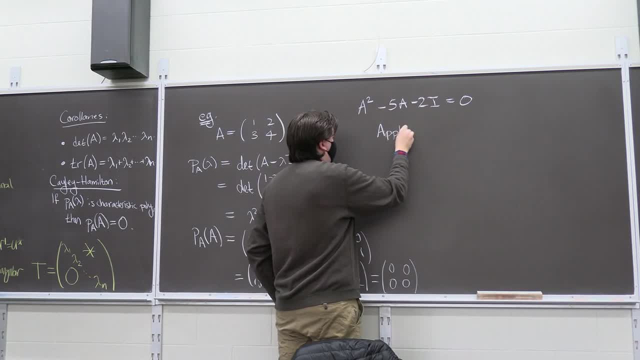 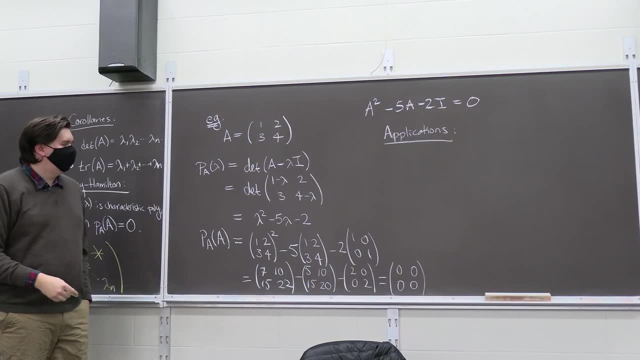 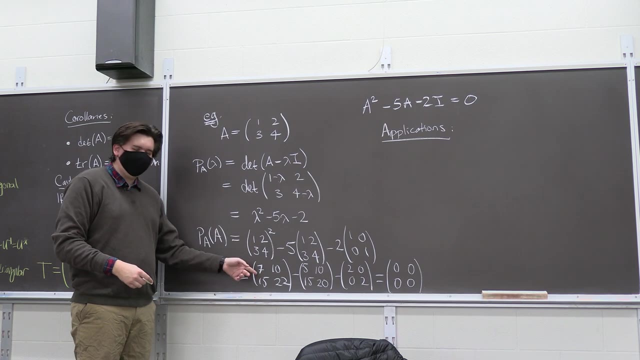 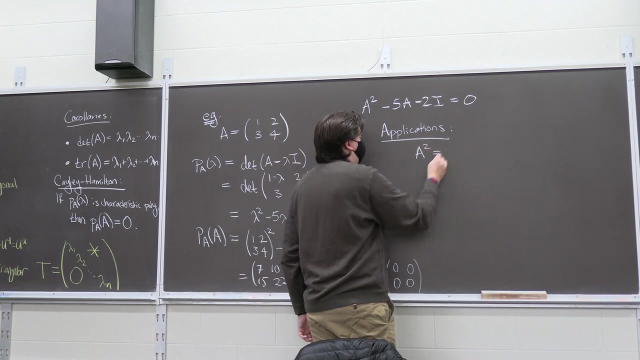 So let's look at two quick applications. One is suppose it's like: this was hard, I'm all playing the matrix by itself, Like that got kind of tricky and confusing. I didn't have to do this, I could have just noted that a squared is 5 times a plus 2 times i. 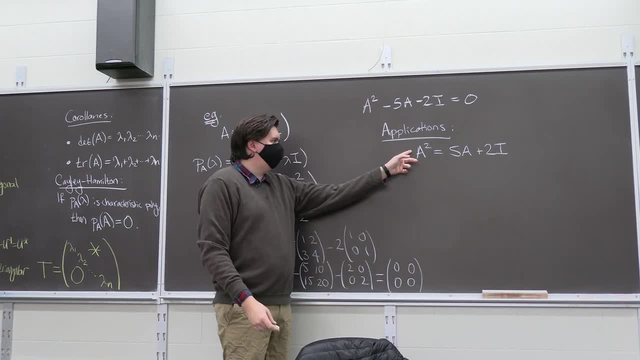 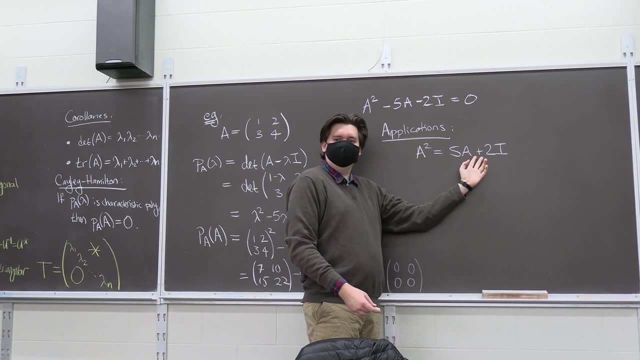 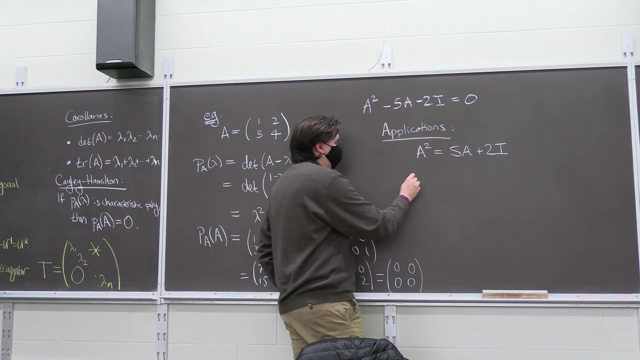 I've just changed the power of a matrix into simply taking a scalar of a matrix plus adding another matrix. These are very easy operations, right? So I've turned power into a very simple expression. You can do higher powers too. What would a cubed be? 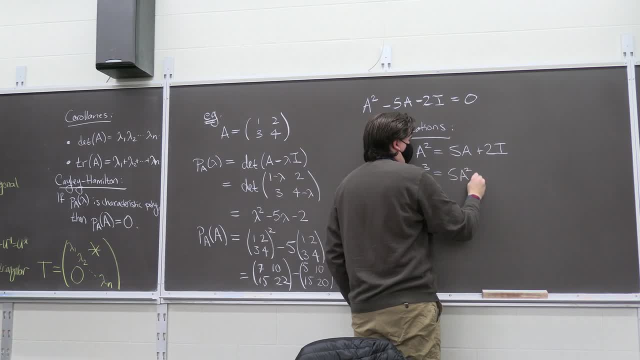 Well, I'll just multiply the whole thing by a, So it's 5a squared plus 2a. And it's like: well, what's 5a squared? I know what a squared is. a squared is 5a plus 2i. So now we just have 25a plus 2a, so that's 27a plus 10i. 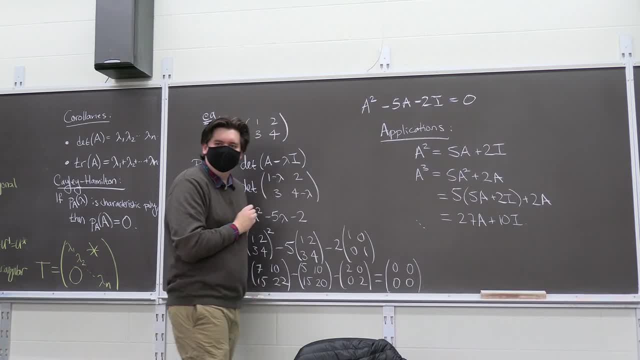 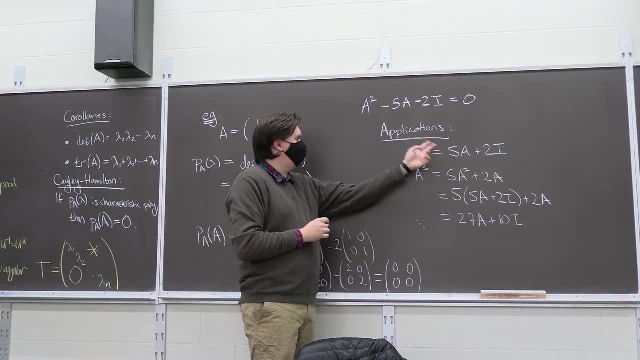 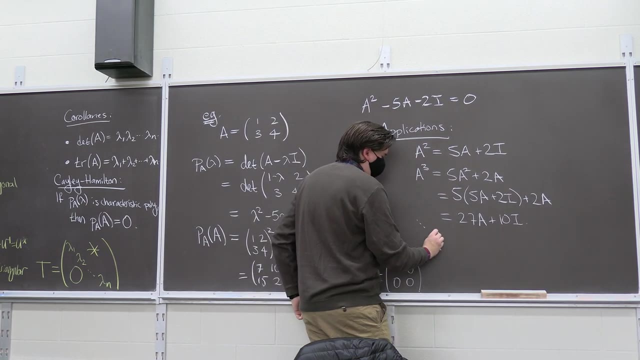 And you can continue in this manner and calculate higher and higher powers. right, Because you can just keep lowering the power by 1, using this relationship, until you have a to any power. in general, you have a to any power. it's just some number of copies. 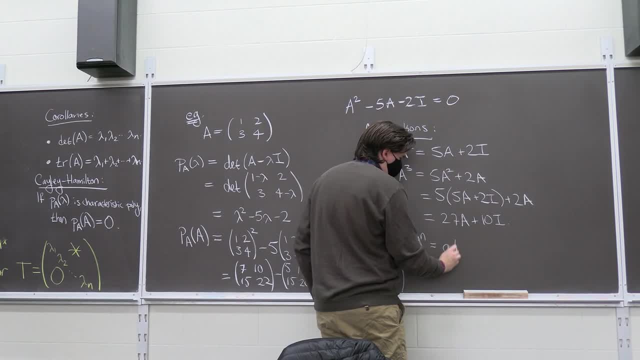 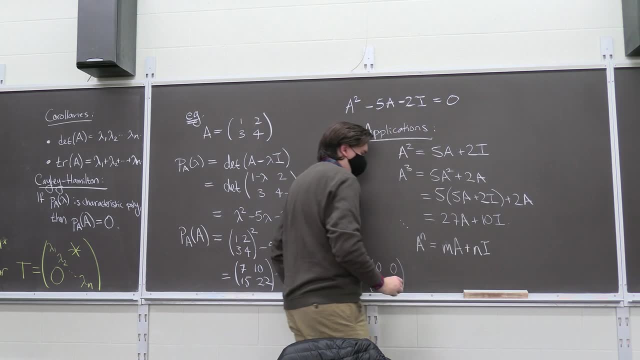 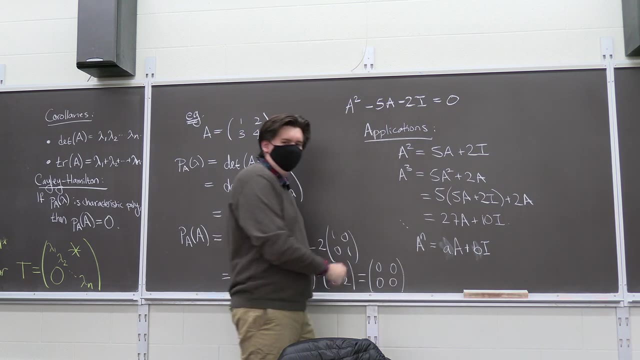 which of my coefficient names be Some number of copies of a. these are integers, so let's say some number of copies of a plus some number of copies of i. That should not be an n, let's just call these a and b, And I suppose you could think about a. 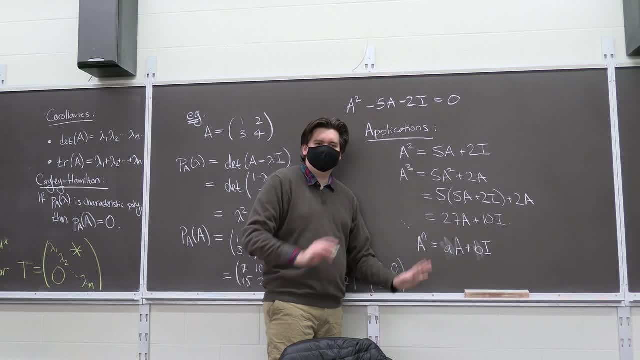 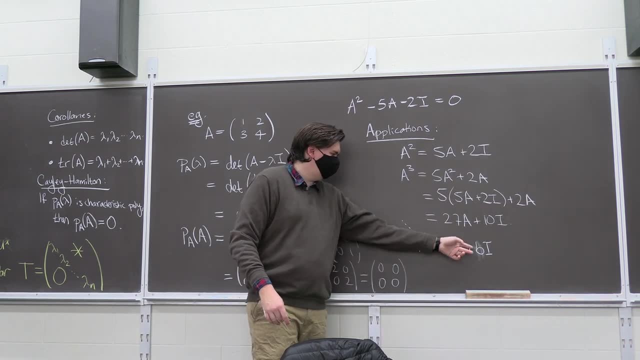 little bit and come up with a general formula. I'll tell you where your a and your b are right. So this wouldn't be too bad. You just kind of figure out what's going on each time And I think pretty quickly you can figure out. 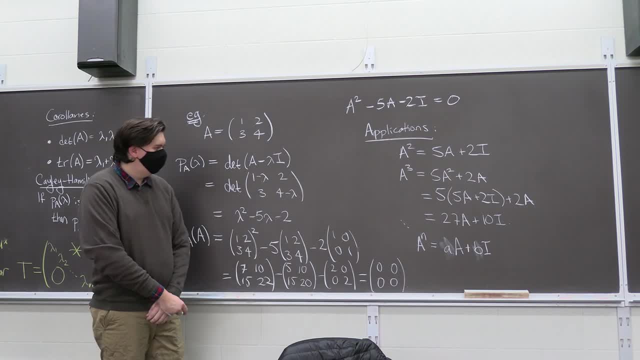 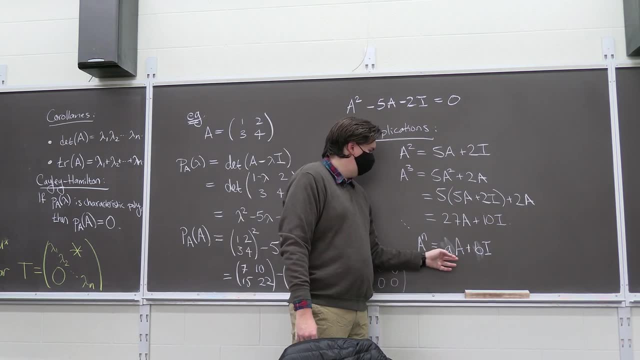 expressions for your a and your b in terms of n. And so, Cayley-Hamilton, lets us reduce finding powers of matrix to a much simpler operation of just scaling and adding matrices. The second application I'll mention is what if I want to calculate a inverse? 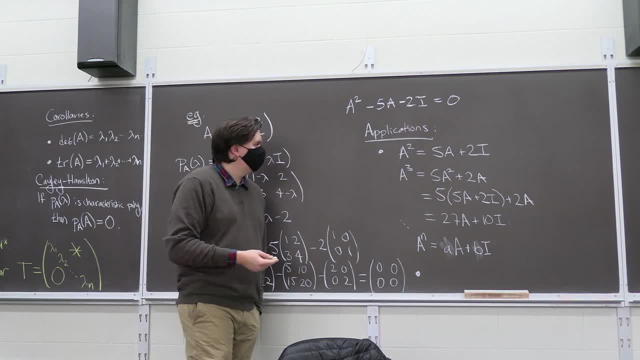 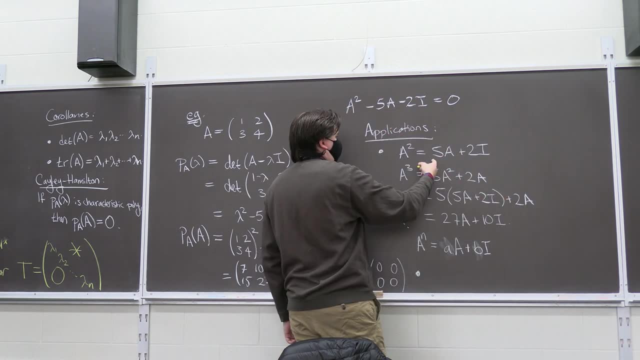 What is the inverse of a? Well, here, instead of solving for the a squared, like I did in this term, I'm gonna solve for the i. So what is the identity matrix equal to? It's going to be a squared minus five a. 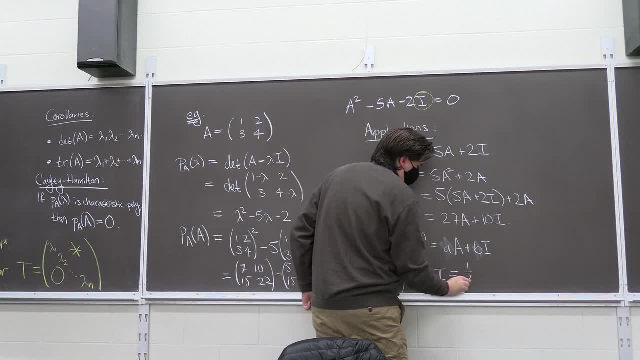 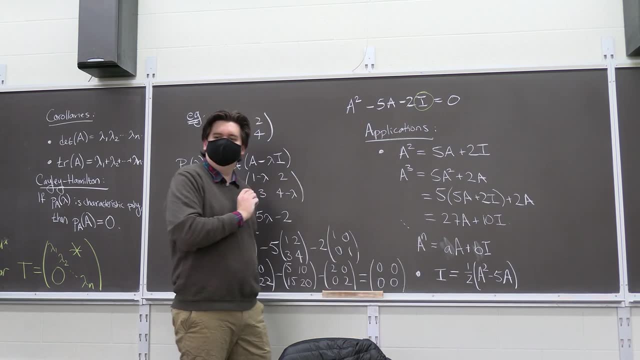 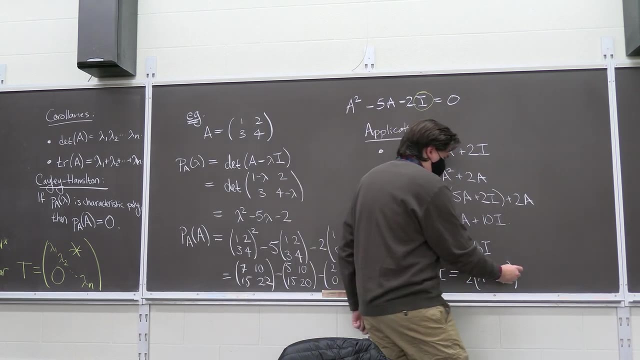 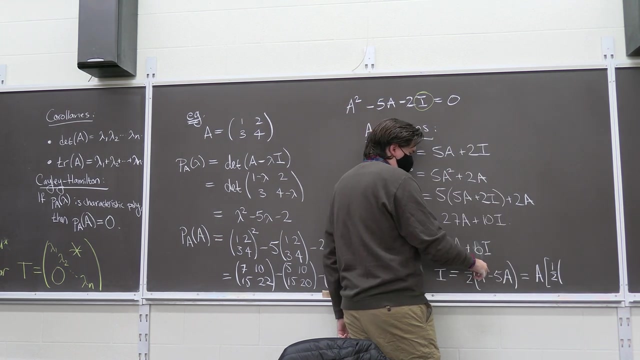 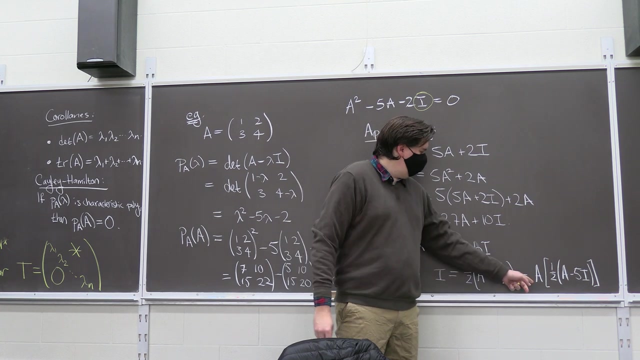 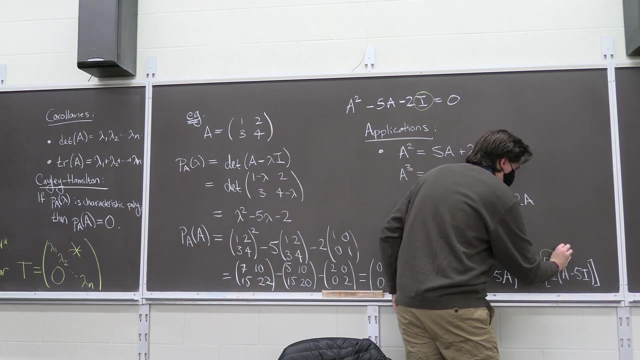 scaled by one, So one half of a squared minus five a. But then we can pull out an a, So it's a times one half of a minus five, times the identity. Now, a times this matrix is the identity. Ergo, this matrix must be equivalent to your inverse. 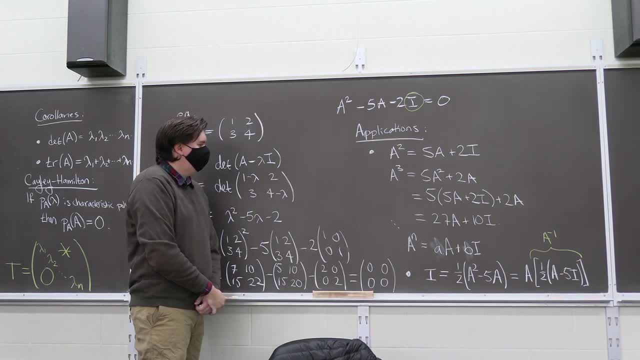 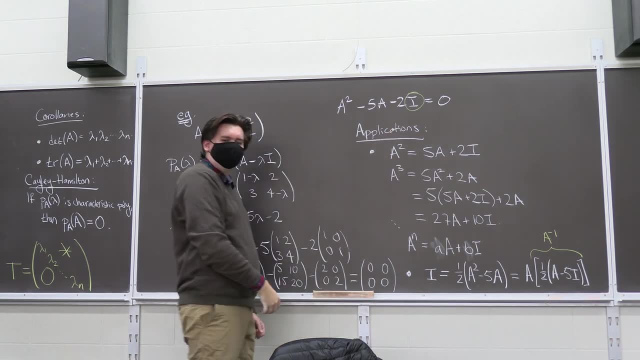 Okay, so we can keep chasing down examples like this, but hopefully it's beginning to show. once you have a relationship between some higher power of a and lower powers, it lets you do tricks like this very nicely, right? So this is one reason why we care about Cayley-Hamilton. 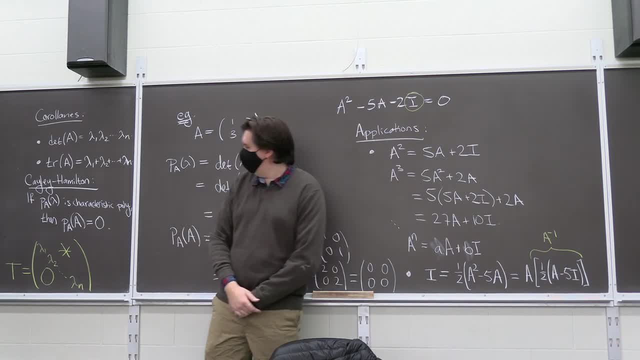 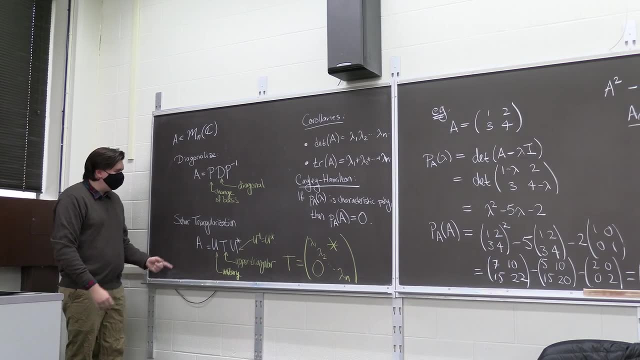 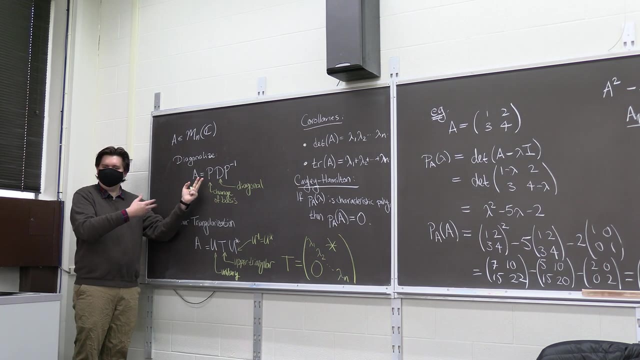 But I want to step back now and come back to a short triangulization, because it's like we gained something when we moved from here to here. We went from just some whatever that change of basis is. p is some basis right. 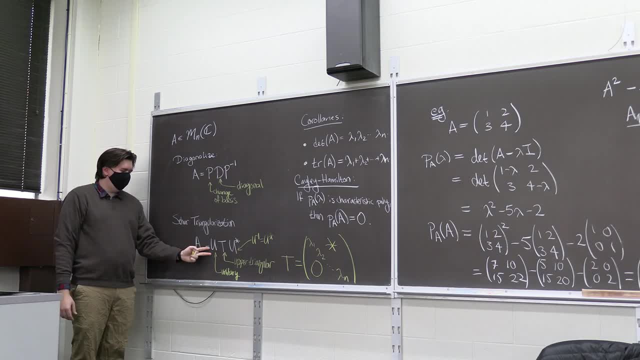 The columns of p comprise some basis to a unitary matrix. So now the columns are a orthonormal basis. So that was a gain, but we also lost something. We went from having a diagonal matrix, which is nice, which means that these vectors here 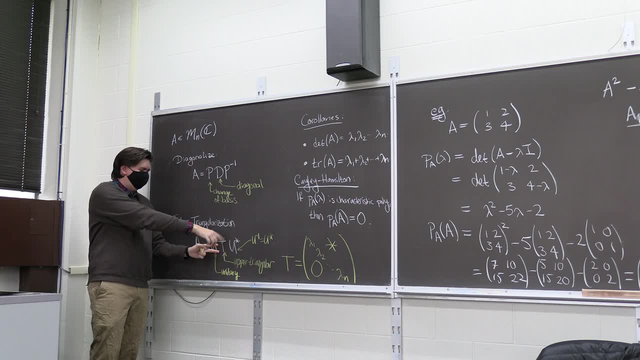 these columns are actually eigenvectors to now having some upper triangular matrix, And you might want to ask yourself: well, what if I want to have the best of both worlds right? It's like: when can I have this being both unitary? 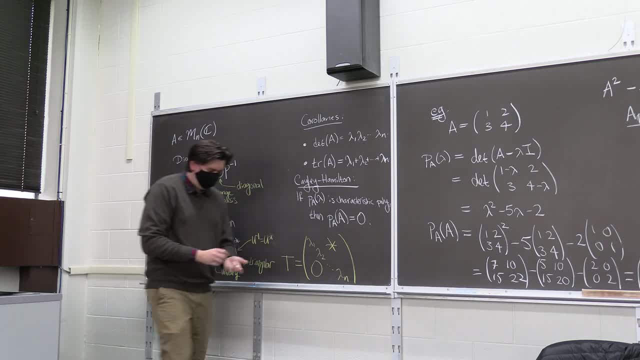 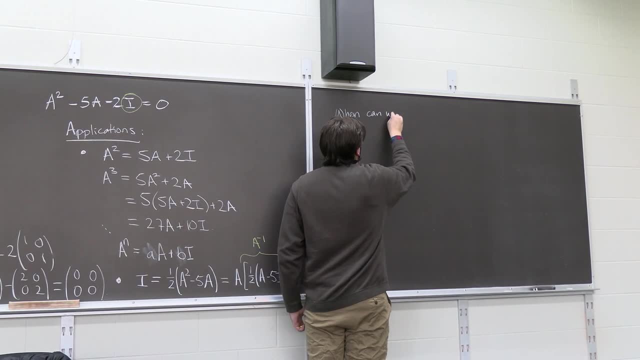 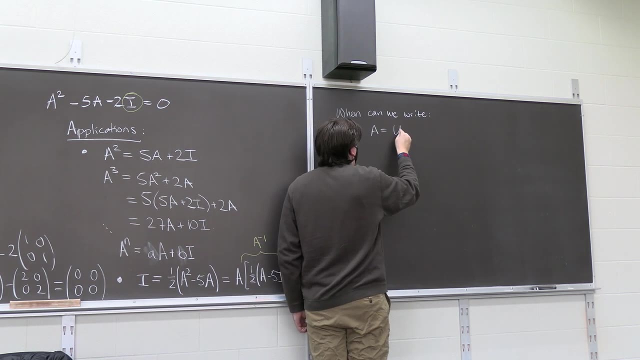 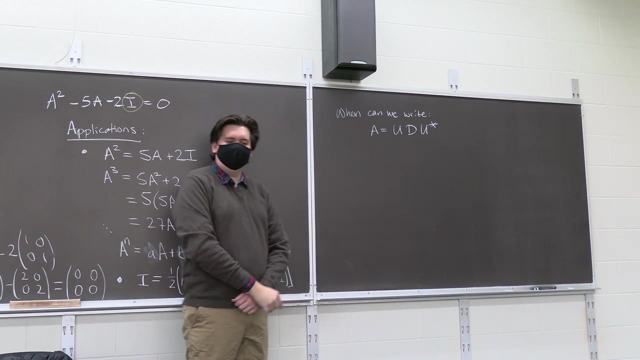 and t actually being a diagonal matrix. So the question I want to ask us is: when can we rewrite a as some unitary matrix? u times a diagonal matrix times the conjugate transpose of a unitary matrix, Because this is where you have lots of nice properties, right? 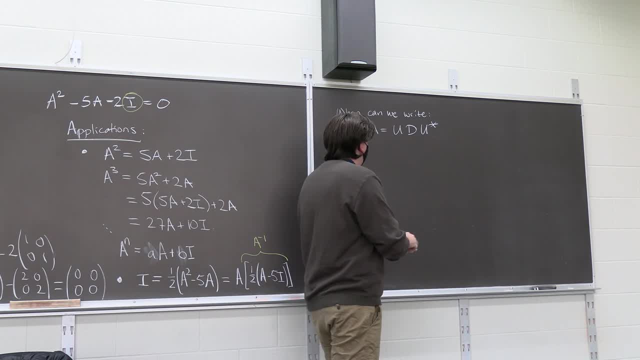 As I've been saying, this is diagonal. This should be your eigenvalues. So here d It's just my eigenvalues, lambda one through lambda n. Again, we're working over the complex numbers, so these might be complex. 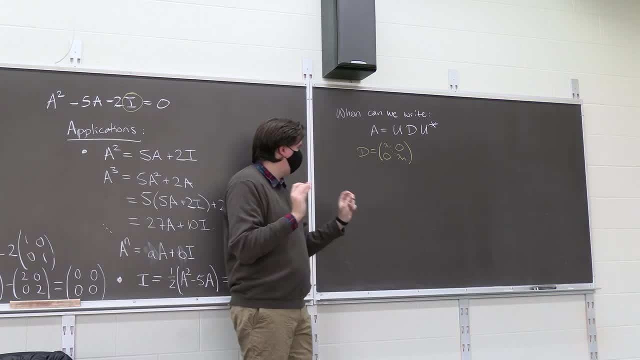 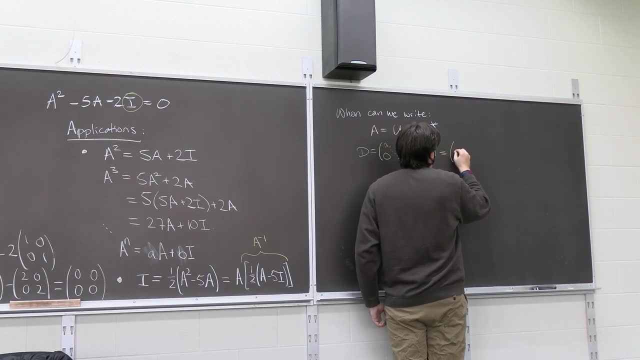 Next class we'll talk about: well, what if we want to make everything real? But today we're going to stay with the complex numbers. But, u you know, it'll have some column vectors: u one through u n And these: u one through u n. 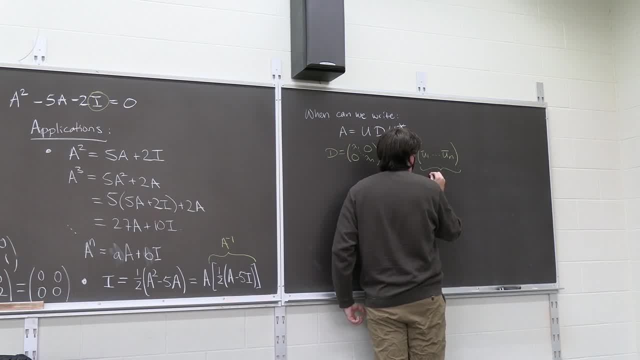 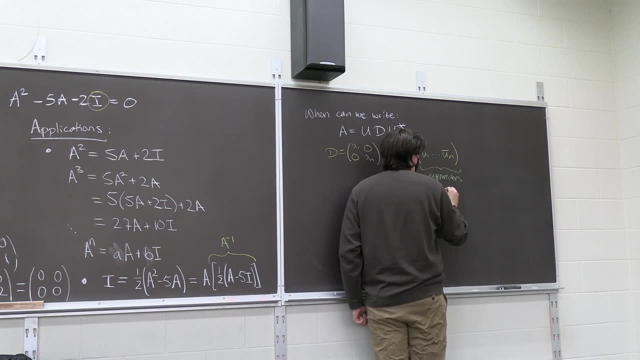 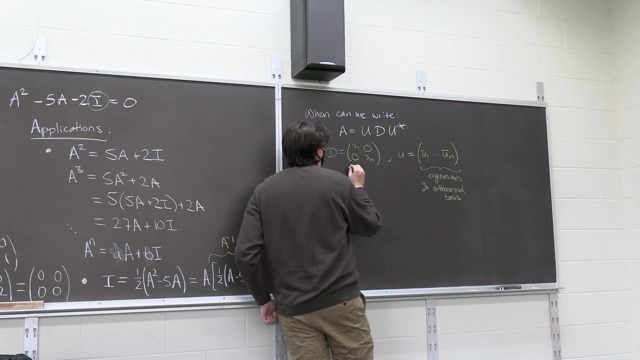 are the complex numbers. So what we've got here would be both eigenvectors and it would be an orthonormal basis. So my, that's all the good stuff, right? So requires investing. Here we have the eigenvalues. He, we have the eigenvalues. 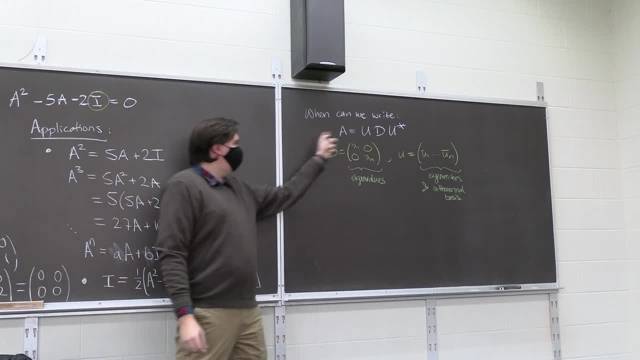 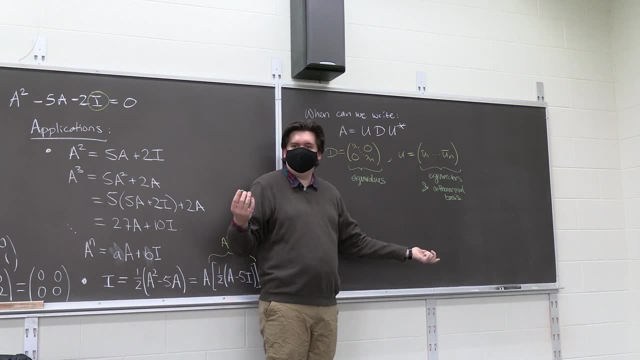 kind of matrices can you do this? And it's like, well, the answer is: I guess you can do this when there exist eigenvectors that form an orthonormal basis, right? That's the answer. It's like, well, when does that happen? right? When do you have eigenvectors that form an? 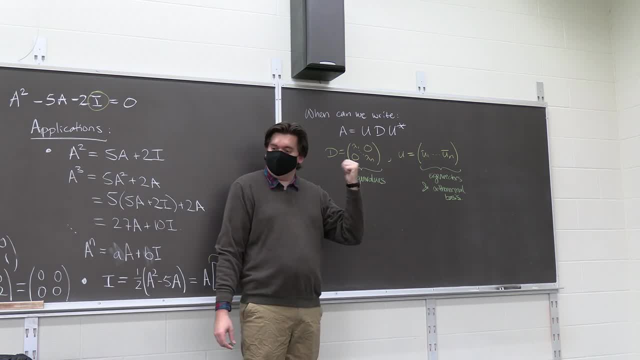 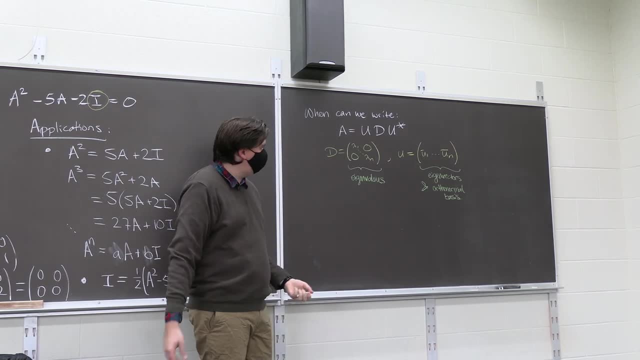 orthonormal basis. If you think back to the example I gave you last class, that actually was an example of this right And we actually did this process and it came out to be of this form. But in general, when do matrices have this property? that they have eigenvectors, that 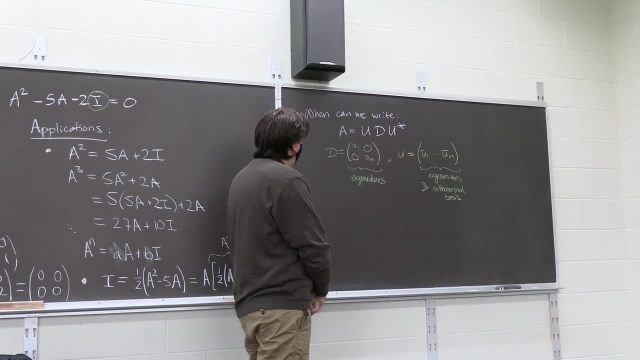 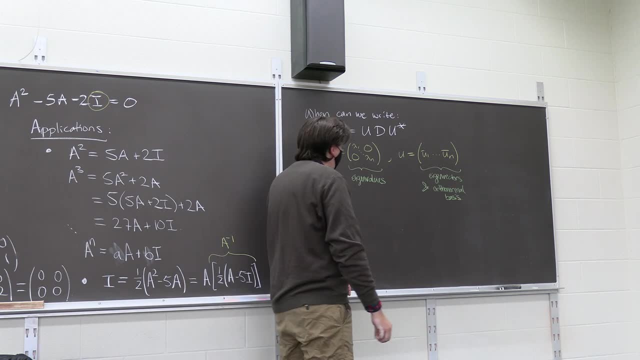 form an orthonormal basis, right? So that's what I want to think about for a minute, And so maybe what I'll do is just play around a little bit. I don't know like, should I give you the answer? Maybe I'll just give you the answer, then we prove it. 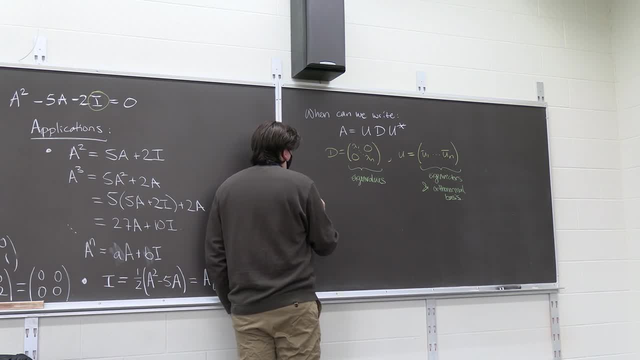 So here's the answer: Theorem. So we're given some matrix A with complex entries, square matrix And by n matrix. then I want to say we can write: a is a unitary matrix times a diagonal matrix times the conjugate. transpose of the unitary matrix: if, and only if, a times its conjugate. 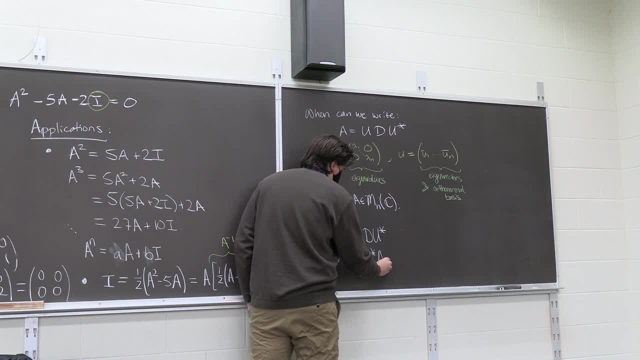 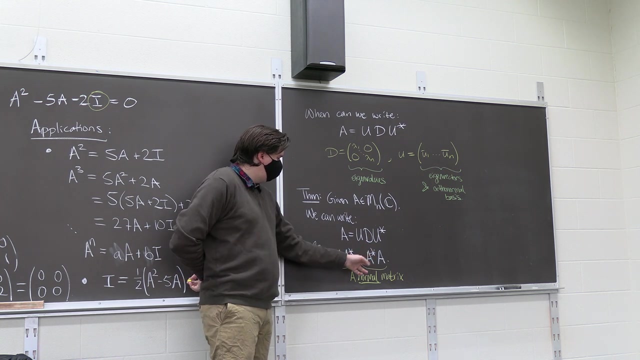 transpose is equal to a conjugate transpose times itself. This is called a is a normal. a is a normal matrix- Any matrix that satisfies the property that when you multiply by its conjugate transpose, you can commute. so it's a conjugate transpose times itself. 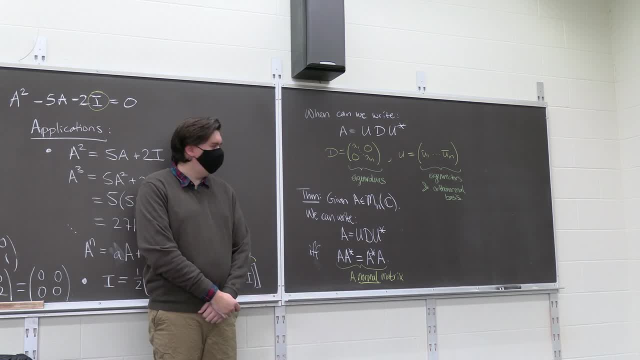 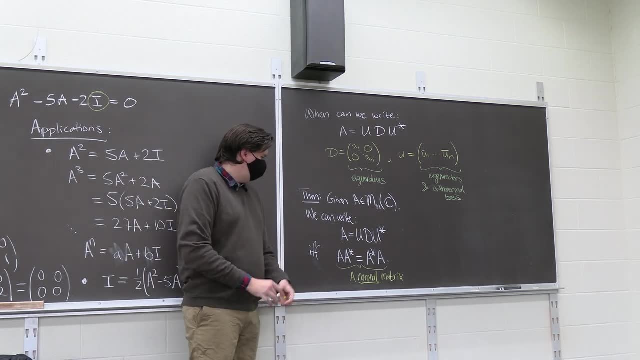 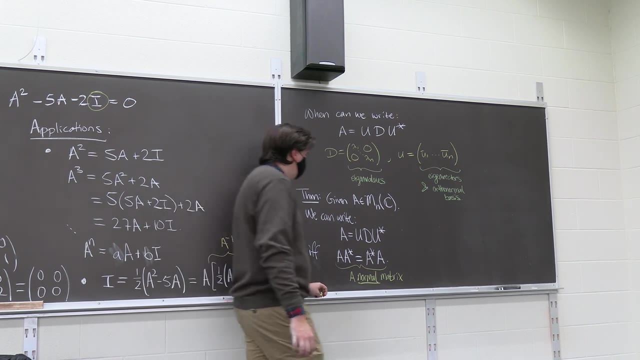 We call this matrices normal. Okay, So we'll prove this here in a minute, but maybe what I'll do is just spend a couple of minutes suggesting that this is not actually so uncommon, that there's a large number of matrices for which this works. 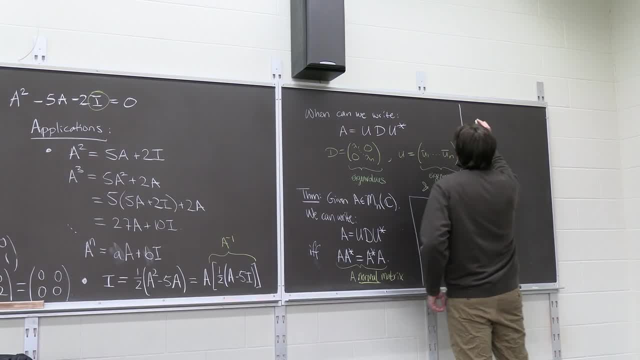 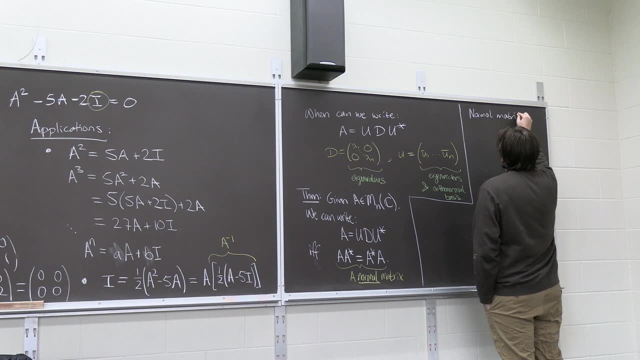 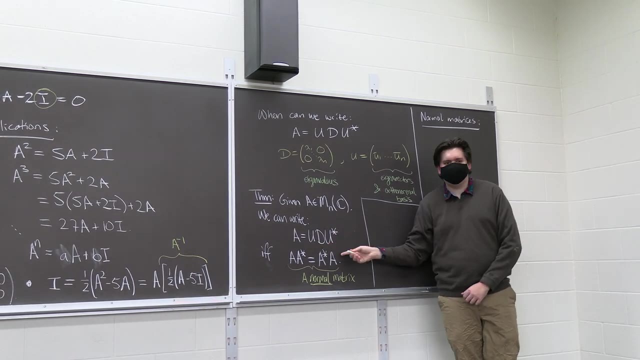 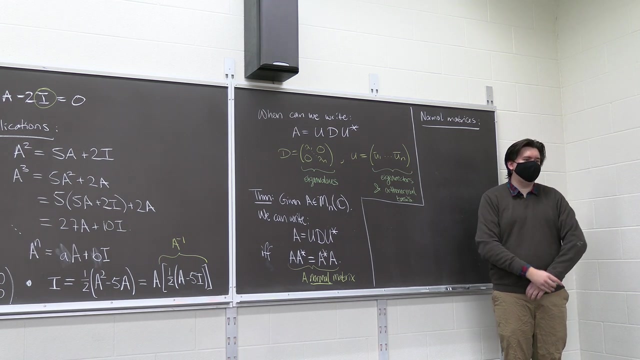 So let me just give you some examples of normal matrices. So we want to look at some normal matrices. Okay, Can you think of any kind of matrix that satisfies this property? Okay, Good, That does the matrix. satisfies the prop, so does zero. 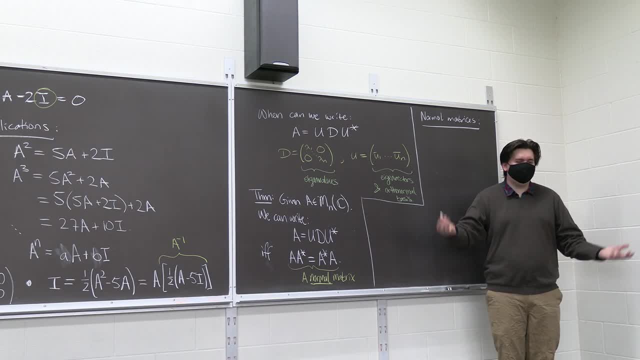 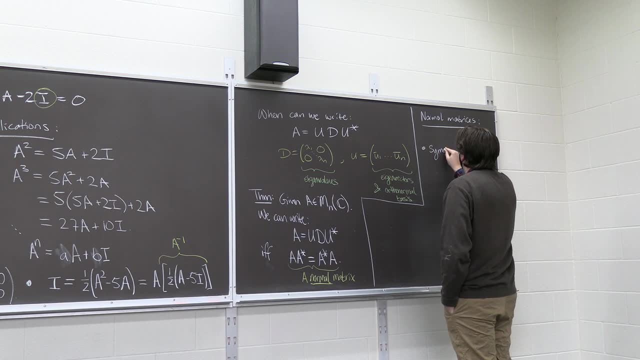 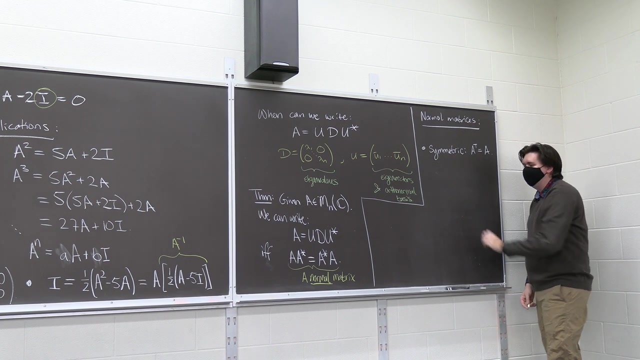 Okay, Got those out of the way. Can you think of any class of matrices? Symmetric matrices, Good. So recall what it means to be symmetric. Symmetric Just means that a transpose is a Okay, a right now. typically we call a matrix symmetric when you're working over real 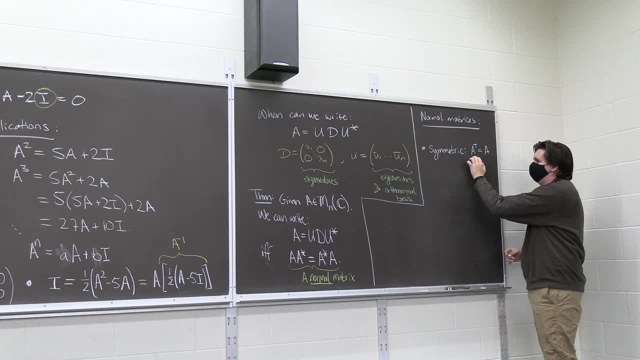 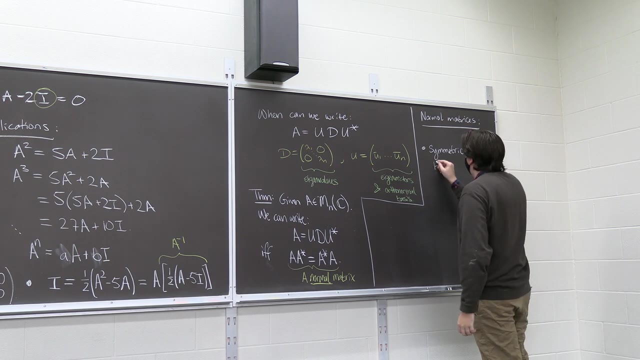 values. so so this is what we call it when working over real values. if you're working over complex values, we instead want to say: a conjugate transpose is equal to a, and you know what we call these matrices: permission, that's right, her nation. so if you're working over the reals, you call it symmetric. if you're, 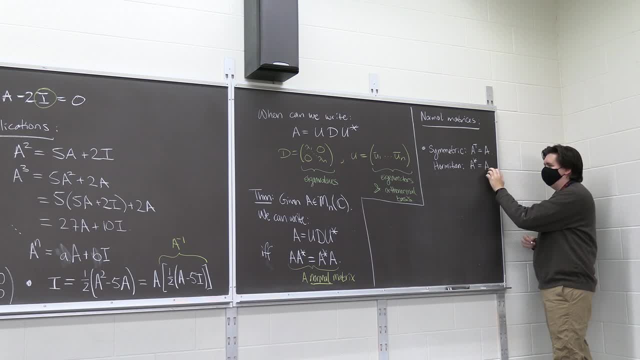 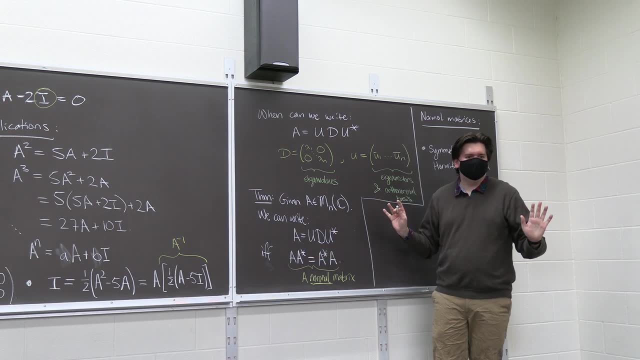 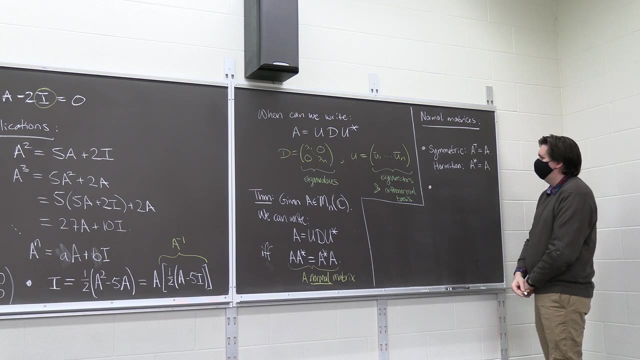 working over complex it's permission, where you have a conjugate transpose a and then clearly is this condition satisfied because a conjure transfer just is a. so both sides just a squared right. okay, give me another example. Oh, unitary matrices, great, and put this one down here. let's do one more here you. 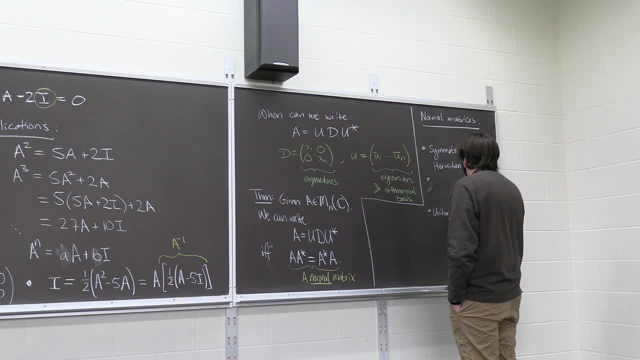 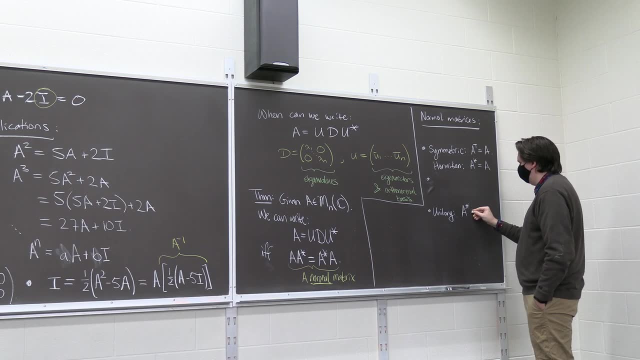 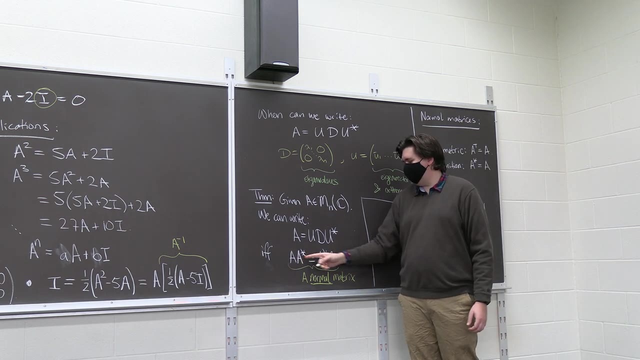 could have a unitary matrix, so a unit if a was unitary. it would satisfy that a conjugate transpose is a inverse right if a was unitary, which means both sides of this would just come out to be the identity. so that's certainly true, and 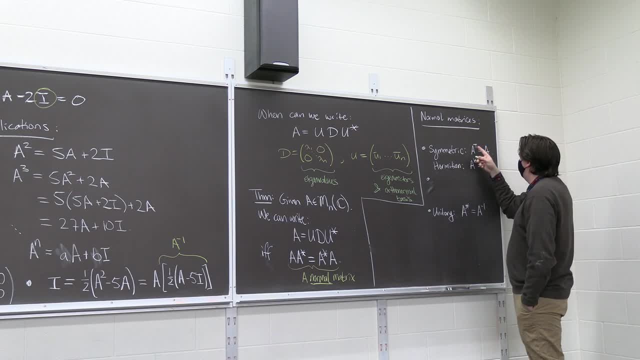 there's one more symmetric is it when a transpose equals a. if, instead, a transpose comes out to be negative a, we call it skew symmetric. so that word skew is just a noting that you're picking up a negative and you have an analogous example. and if you extend to the complex numbers which we're working in instead, 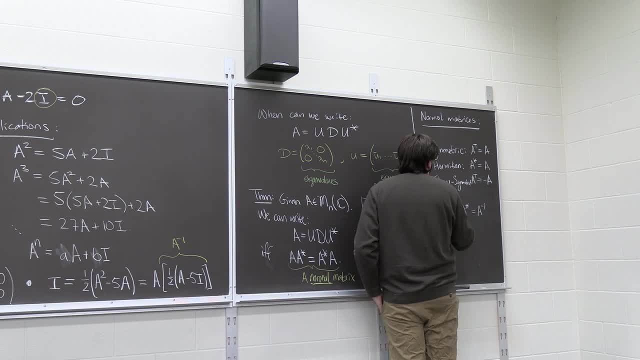 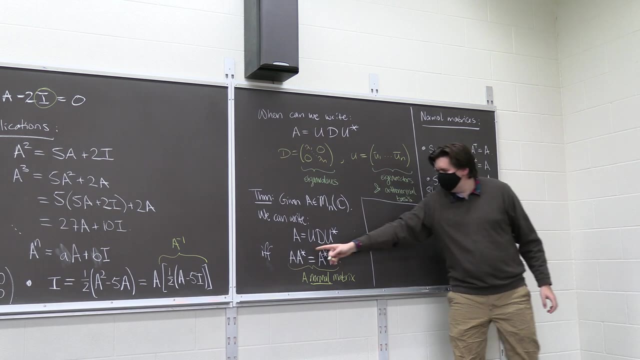 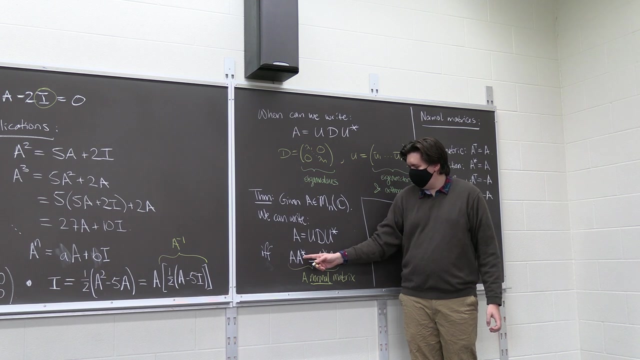 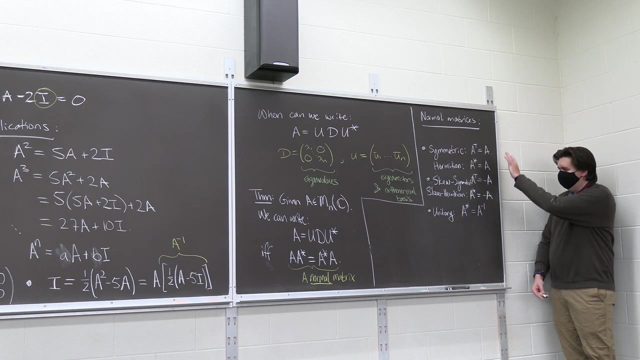 of symmetry, you call it skew. her mission, her mission. a conjugate transpose is negative, a right. if you're working over the real numbers, this is just the transpose. if you're working over the complex numbers, then the conjugate transpose becomes negative a. so that's negative, a squared. and same thing over here. so an important, few important. 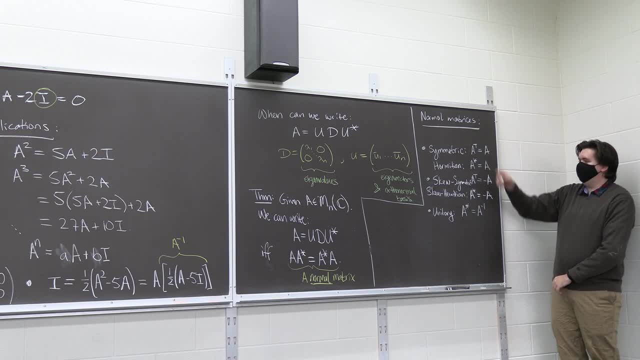 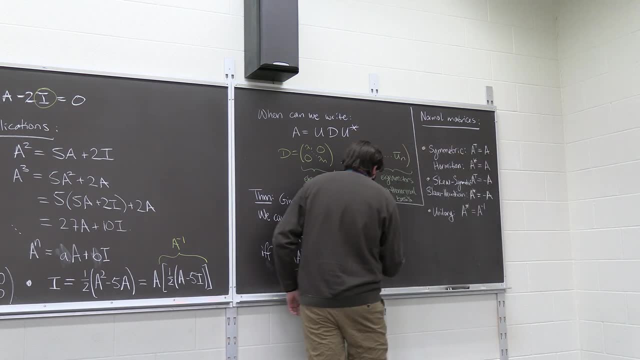 classes of matrices, all of which fall under this family of normal matrices, so it's a pretty broad family. if we were to make a make a picture like a Venn diagram, right here I have my family of normal matrices, so maybe I'll denote this by like a big 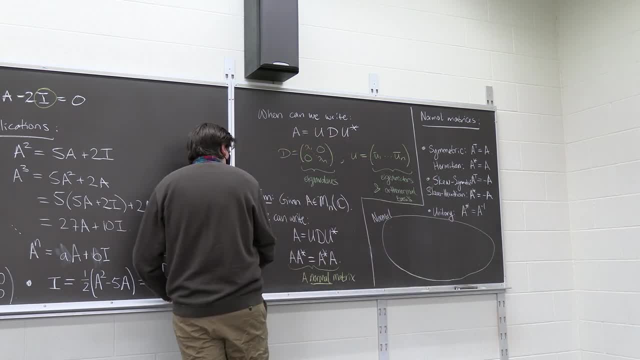 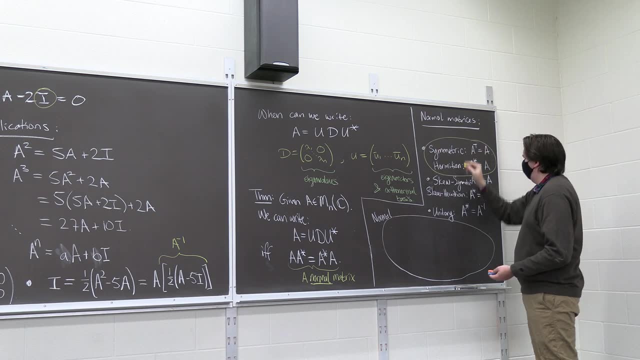 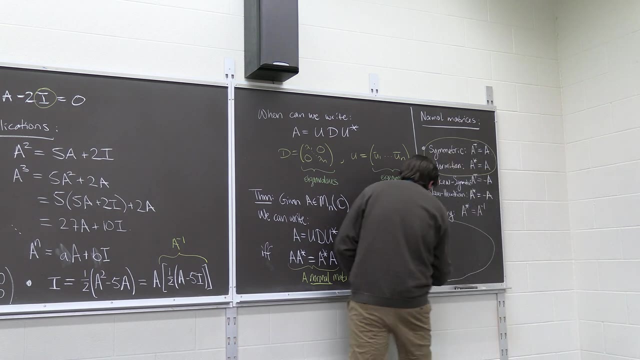 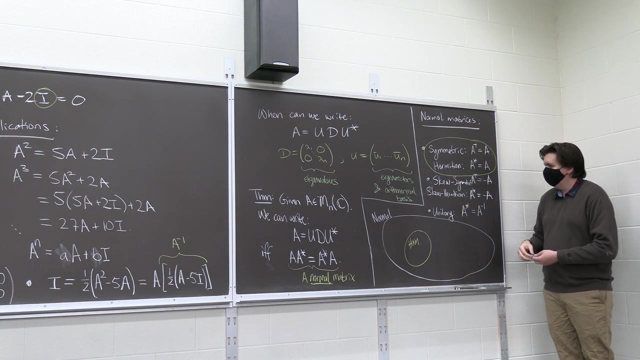 circle. we got a few colors. then in here you would have your family of either her mission or, if you work in for reels, symmetric. but I'm just going to call this a mission for now. when we move to the reals, remember this entails the symmetric ones, the other set, the, the symmetric matrices you would also have. 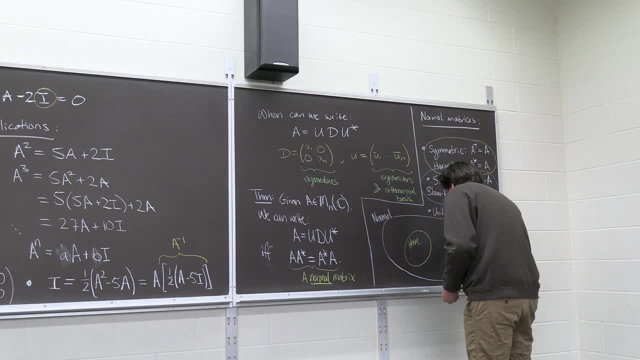 skews symmetric. so you would have skew symmetric or skew her mission and and skew her mission or skew herری, and this would be very, very similar to this one one matrix that sits at the intersection of those two. What is a matrix that satisfies both of these properties? 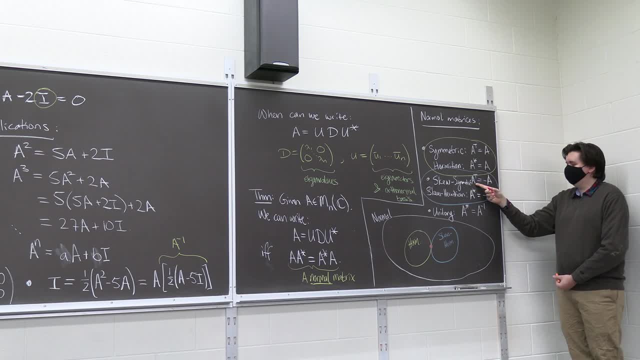 It's transpose is itself, but also it's transpose is negative itself. Only the zero matrix right. It's like you know you need both a to be equal to negative, a right, And that's only gonna happen if you have the zero matrix. 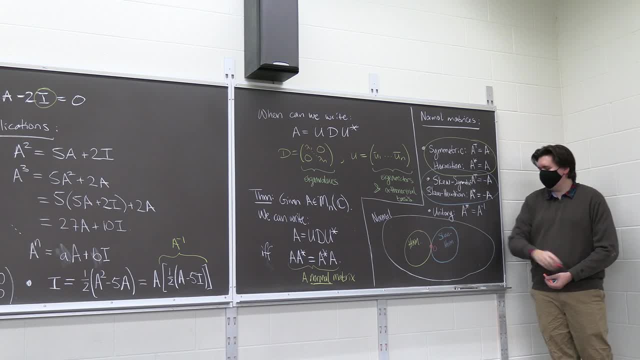 So the zero matrix sits right there at the intersection of them. It's the only matrix at the intersection, It's the only time a equals negative a, And then finally you have this class of unitary matrices. Well, now let's think. 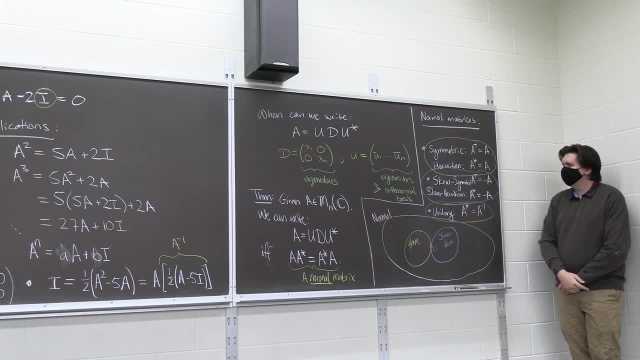 Can you be both unitary and Hermitian? Yeah, some matrices will be. You just need a to be equal to its n and a to be inverse, And there are matrices where a equals its inverse. Those are the matrices where you have a squared is one right. 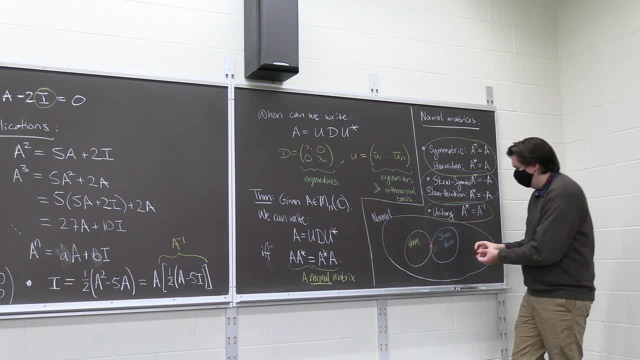 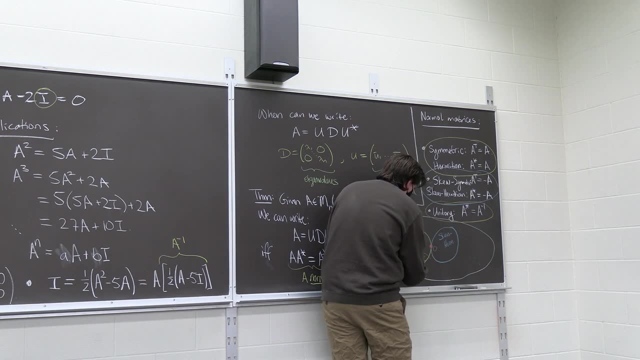 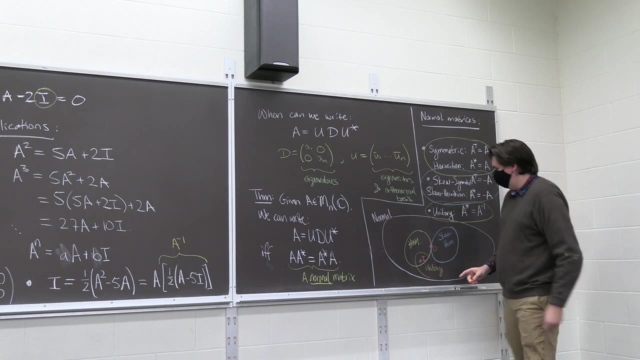 Or a squared is identity matrix And so there'll be some matrix that do that, in particular the identity matrix. So the identity matrix here i is gonna sit at the intersection of Hermitian and unitary matrices. Can you be both a unitary matrix and skew Hermitian? 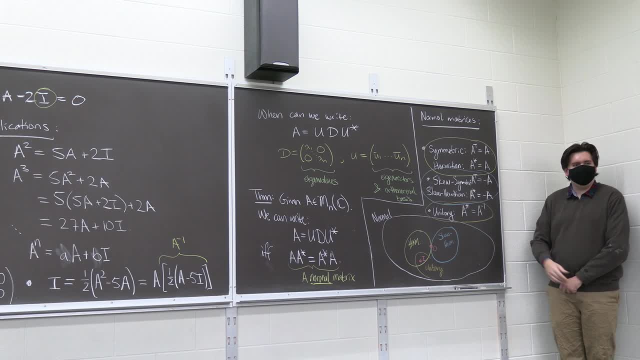 Well, now it's like you want the inverse to be negative a Can that happen? Yeah, this might take a little bit of thought, But if you think about, like for two by two matrices, how you find the inverse if you just have, like, maybe zeros on the diagonal. 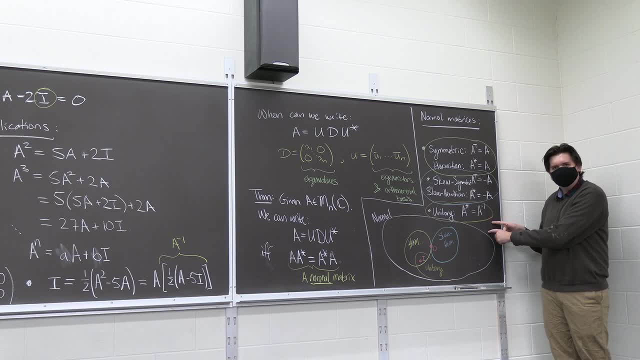 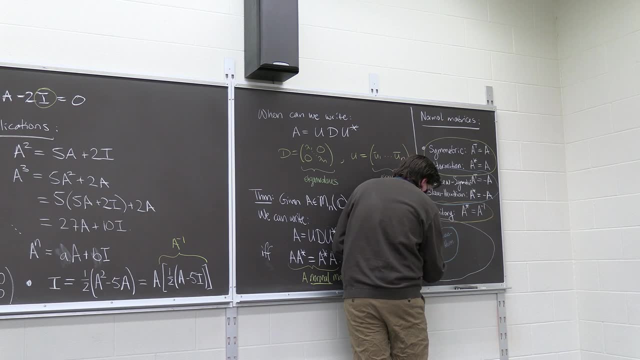 and maybe something like one and negative one down here. I think that'll work, Because then the inverse just flips those, which is just finding the negative. So there's some. it can work. You can have some overlap, You can have some overlap. 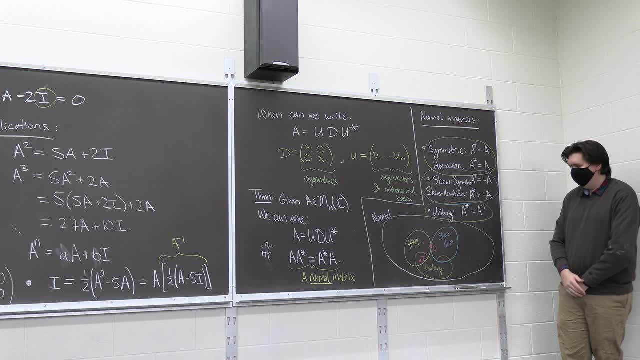 And then you'll have some normal matrices that are none of these right. So you have these three classes that intersect with each other. Here the intersection's pretty trivial, but they intersect and they're all examples of normal matrices. So we'll continue to talk about these classes. 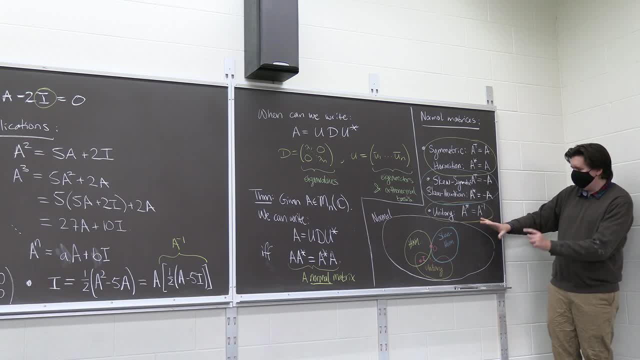 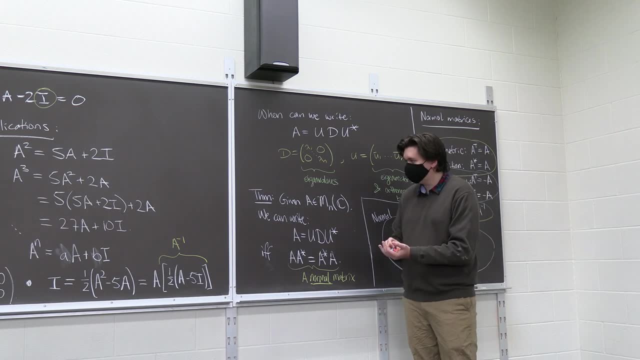 of matrices quite often, And so I just want to have a good sense in your mind- any of these classes, of what we're talking about when talking about a matrix being normal. Okay, we happy with this. So I guess I should prove this claim right. 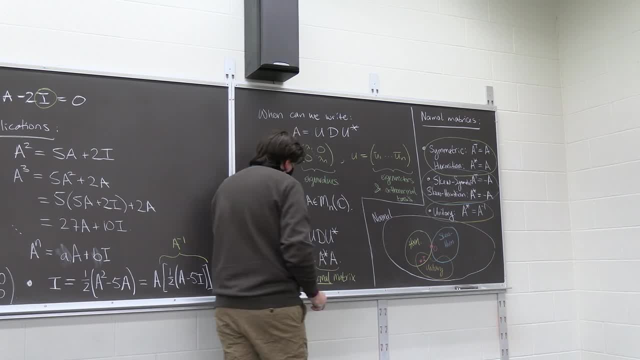 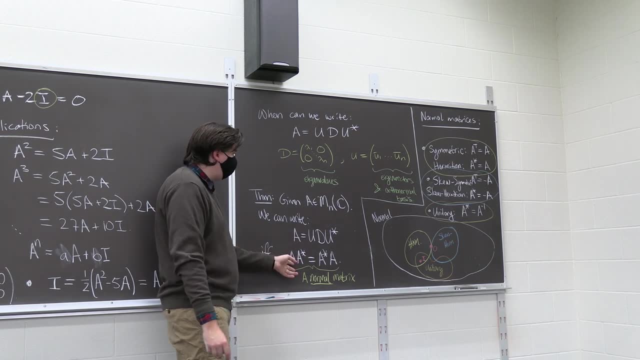 Why did normal matrices allow us to diagonalize in this way to find a? so this is really saying: if you're a normal matrix, if you have this property, you have a orthonormal basis of eigenvectors, right? So that's the big claim. 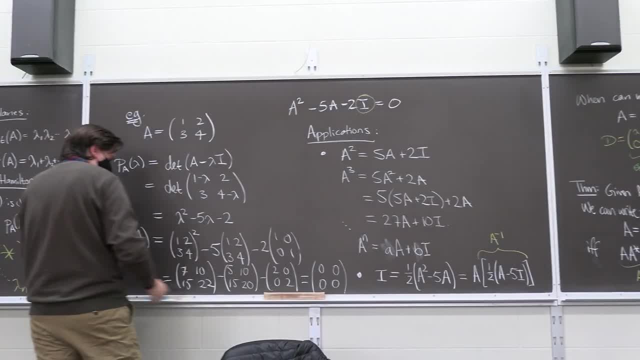 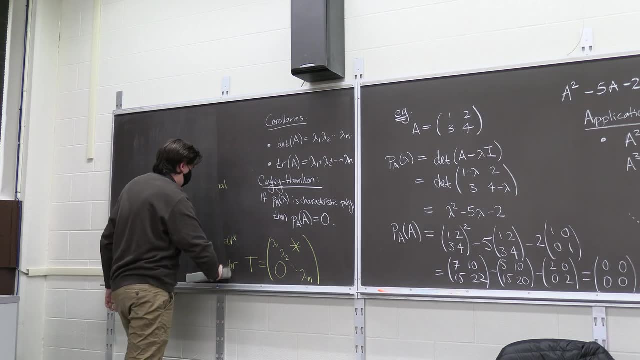 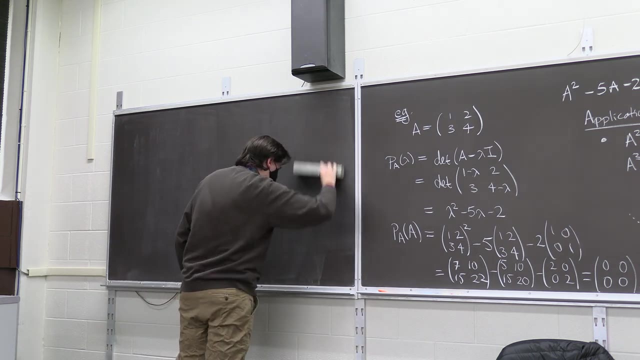 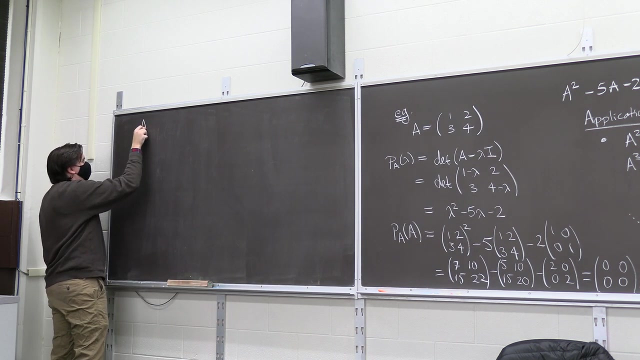 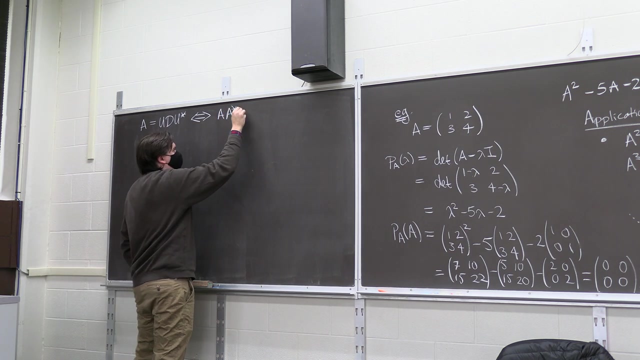 So let's try and prove it. So we're trying to show that you can write a as a unitary matrix times the diagonal matrix, times the inverse of the unitary matrix, its conjugate transpose. if, and only if, a is normal, A conjugate transpose is equal to a conjugate transpose a. 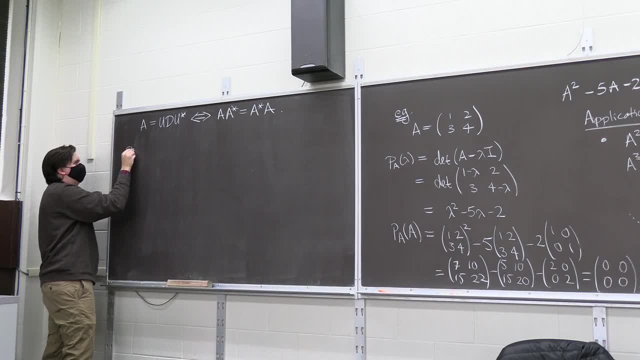 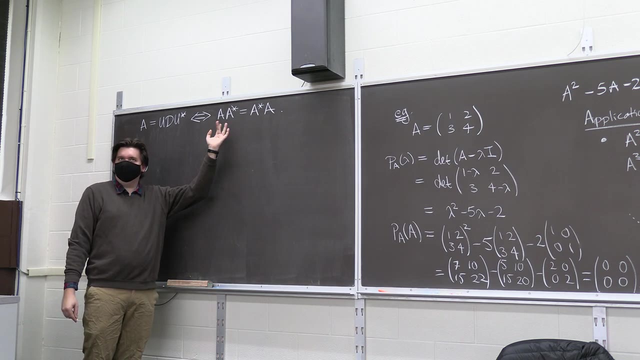 That's what we're trying to prove, So let's give a proof of it. Okay, we got to go both directions, So first of all, we want to prove that A is normal. First let me go the left direction. Suppose your matrix: A is normal. 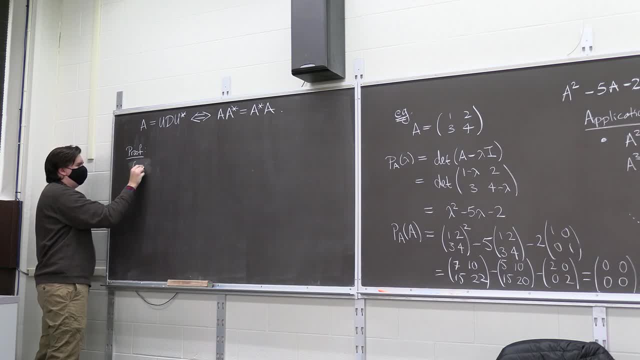 Actually this direction's going to take a little bit longer. So for a quick reward, let's go the forward direction and then we'll go the left direction. Let's suppose you can decompose in this way. I want to argue if you can decompose your matrix. 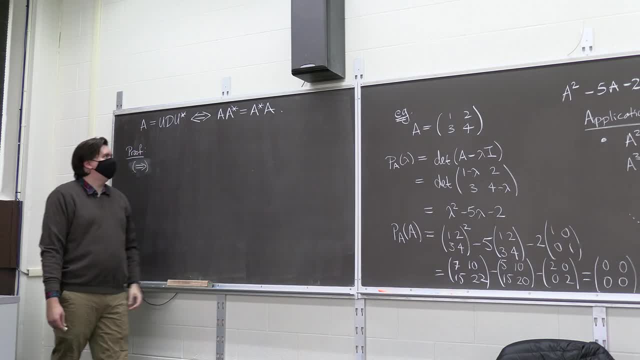 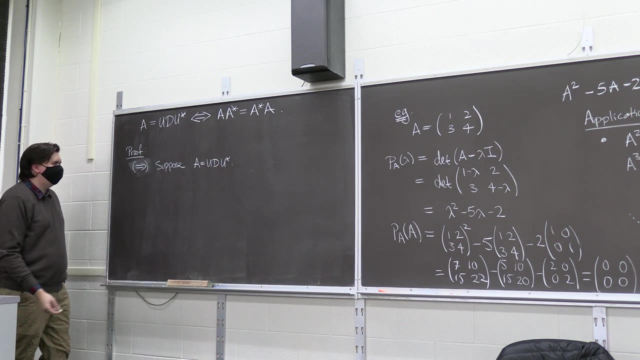 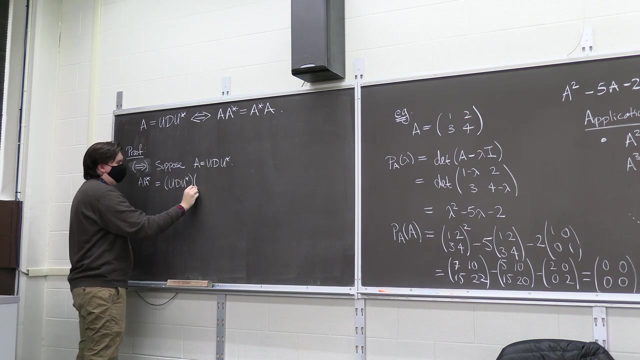 like this, then your matrix is necessarily normal. So suppose A is UD U inverse, Now all we have to do is just calculate what is A A transpose, And so here we go. It'll be UD U conjugate transpose times UD U conjugate. 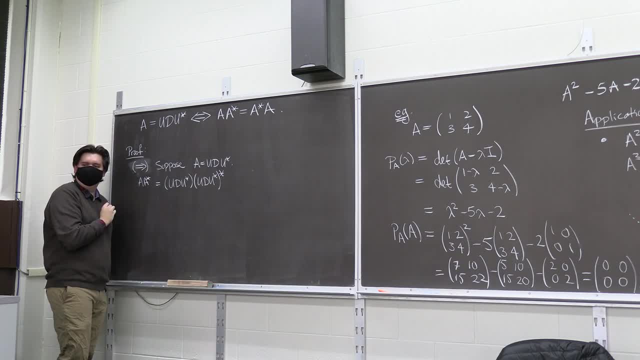 transpose, Conjugate transpose. let's remember how conjugate transpose of a product works. It's just like inverses, right or transposes. You flip the order and then you do the transpose of each one. So we get UD U conjugate transpose. 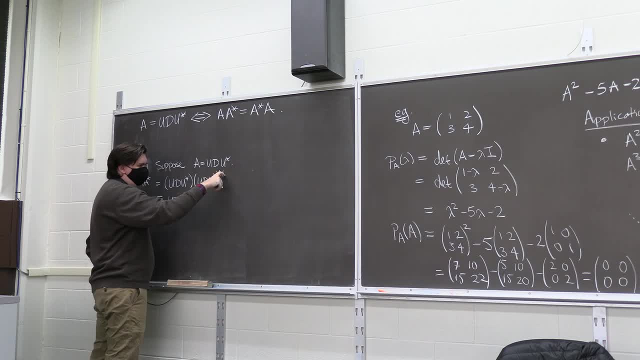 Here the last guy becomes first, So it's U conjugate transpose- conjugate transpose, which takes you back to U. D becomes D conjugate transpose and U becomes U conjugate transpose. But since U is a unitary matrix, U times U conjugate transpose. 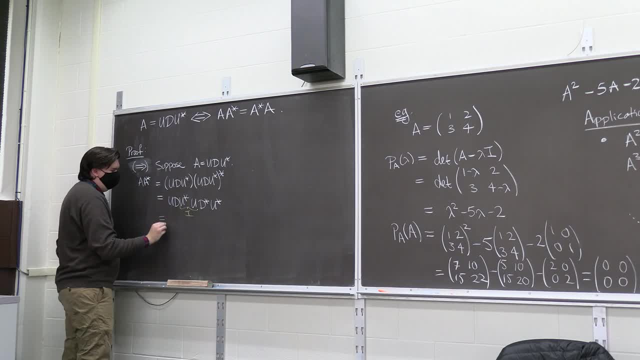 is just the identity. So here we've covered U times D, D conjugate transpose times U conjugate transpose. Now I don't think there's any more simplification we can do. But D is diagonal right And this other D is also diagonal. 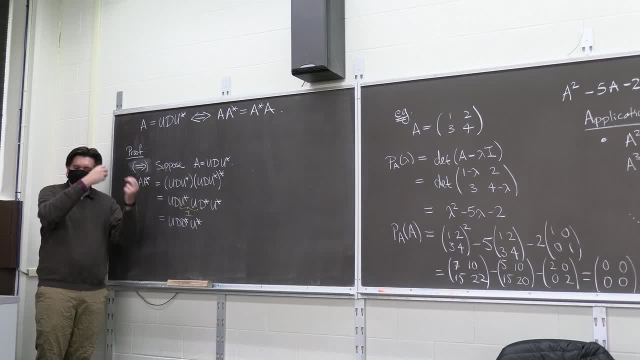 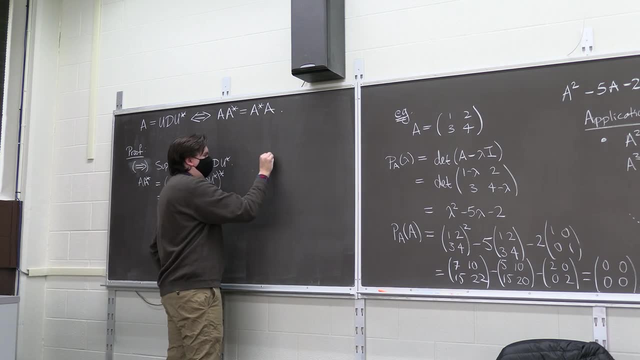 So how do you multiply two diagonal matrices? OK, Well, it's just going to end up being the product of these will just be the matrix that, if we can write it out right here, my D times D conjugate transpose is just: 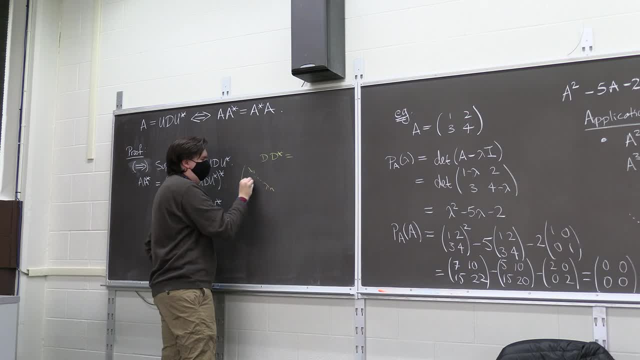 going to be the sky of lambda 1 through lambda n times lambda 1 conjugate transpose. So it's just the transpose of lambda 1, sorry, just the complex conjugate of lambda 1 through the complex conjugate of lambda n. 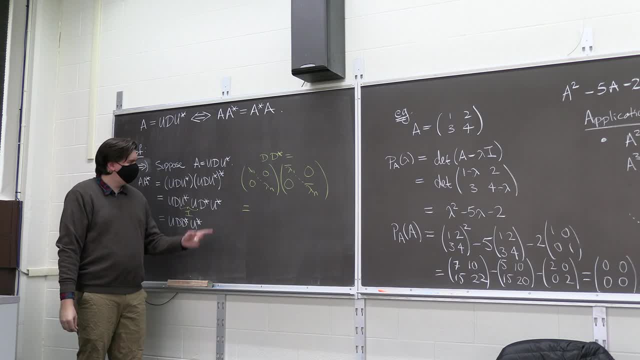 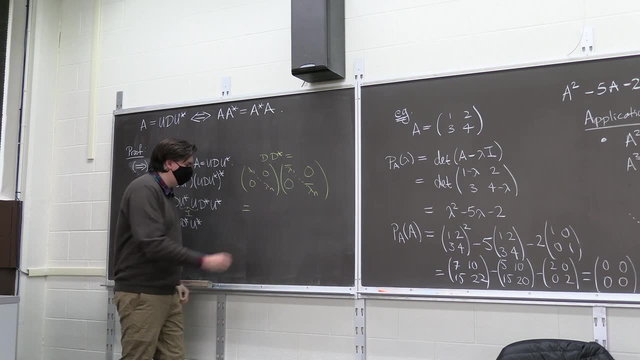 And so what is that? Well, you just multiply row and column and you just get the first diagonal matching with the second diagonal. So it's just lambda 1 times conjugate transpose. It's just lambda 1 times its conjugate transpose. 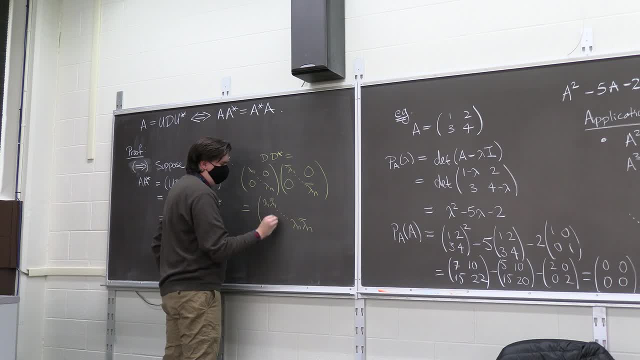 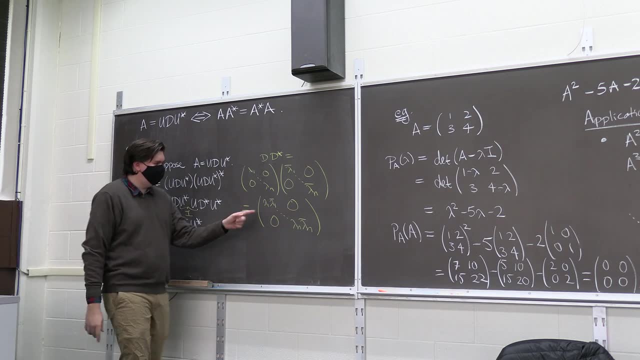 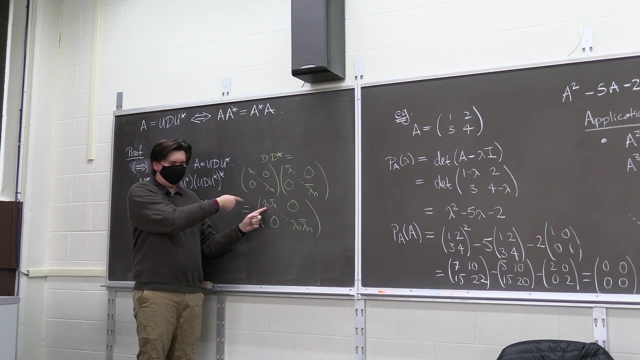 all the way through lambda n times its conjugate transpose. By the way, this would just be like the norm of lambda 1 squared Right. If lambda 1 is a plus bi, this is a squared plus b squared. But here's the point. 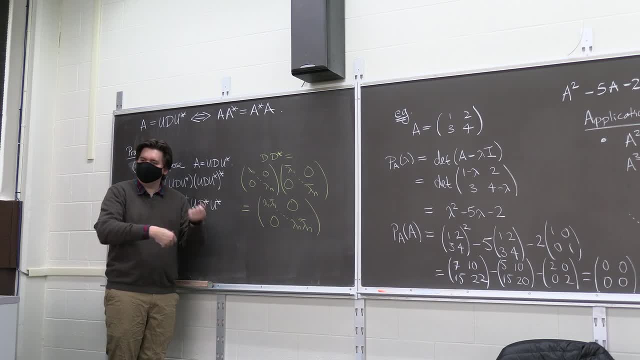 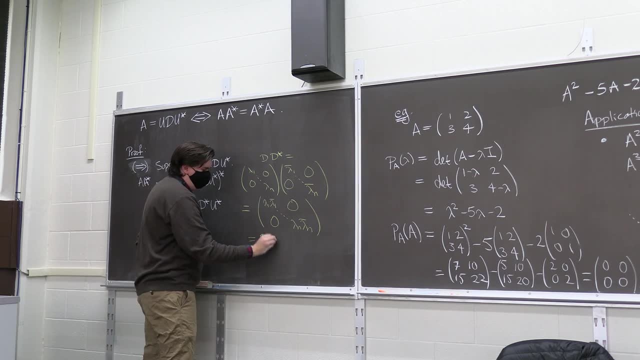 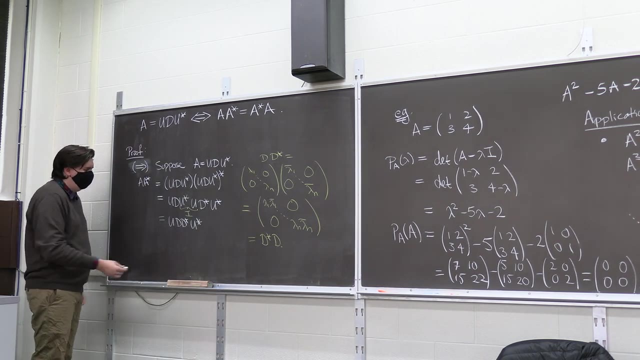 These are just complex numbers. Complex numbers commute, And so you can just flip it And then you can pull it back apart And you end up with d star d. In general, if you have two diagonal matrices, they'll just commute with each other. for this reason, 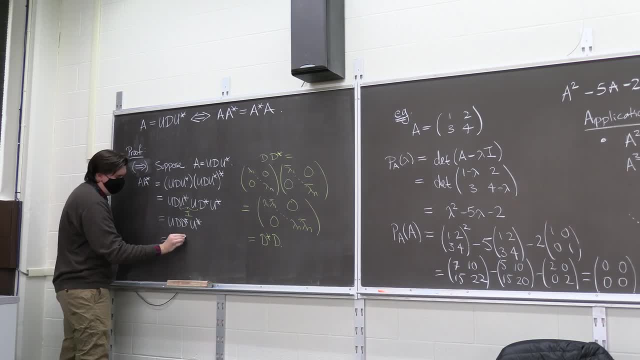 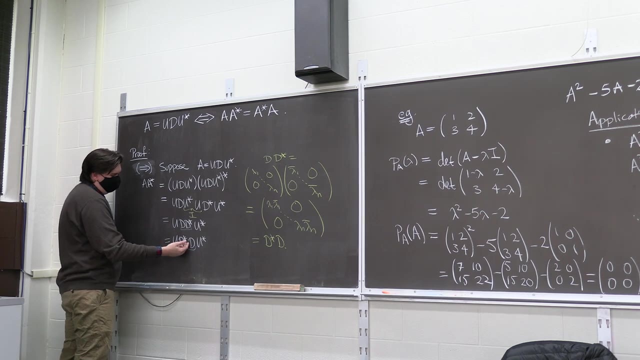 So we can commute. This is just u d star, d u star. I just commuted these two matrices, But then I do all the steps I had done before, but in reverse Right. It's like I can introduce in the middle here these two. 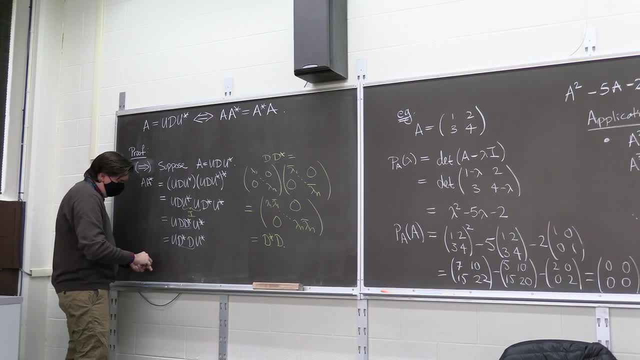 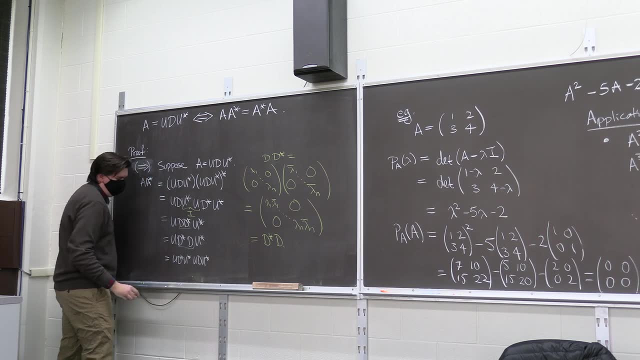 There's like a density matrix there, So you can just slip in u d star, u star, u d u star And like: oh, that guy on the left is just the conjugate transpose of u d u star, Right, Right, Right. 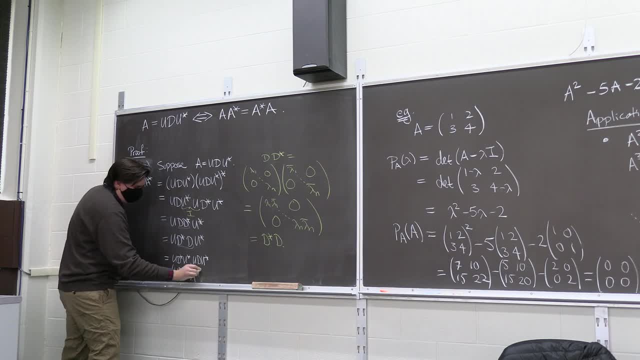 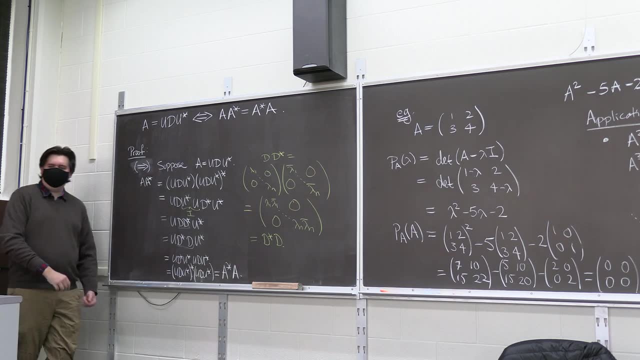 Right, Right, Right. The guy on the right is just u d u star. So that's exactly the conjugate transpose of A times A. So if you want to be able to decompose this way, your matrix has to be normal. 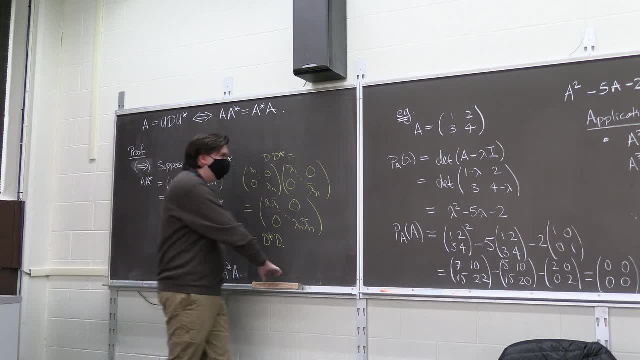 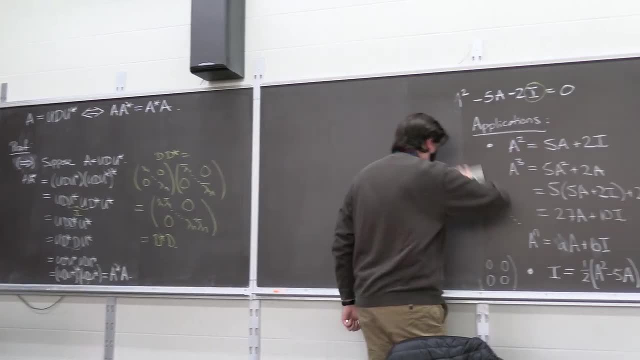 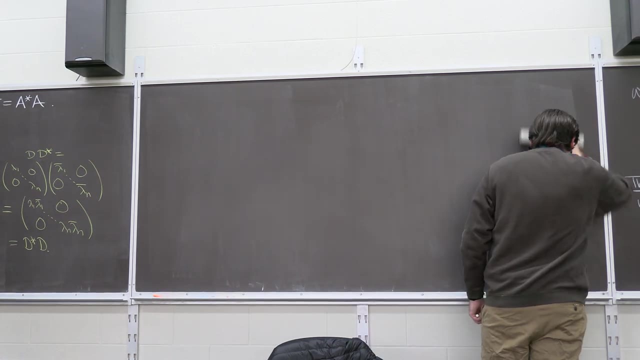 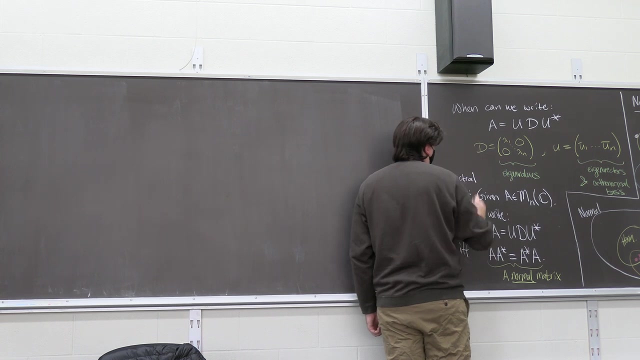 Good, What if we want to go the other way? Let's try and prove the other direction. By the way, this is such an important theorem. it has a special name. This is called the spectral theorem. Sometimes we'll call it the complex spectral theorem, because next class we'll see a version. 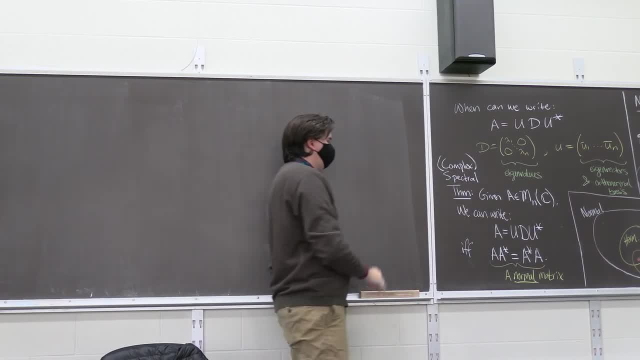 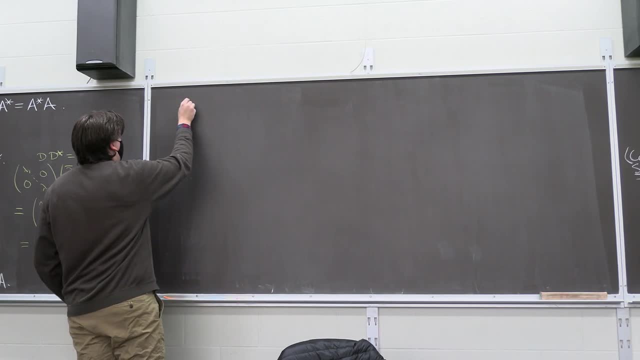 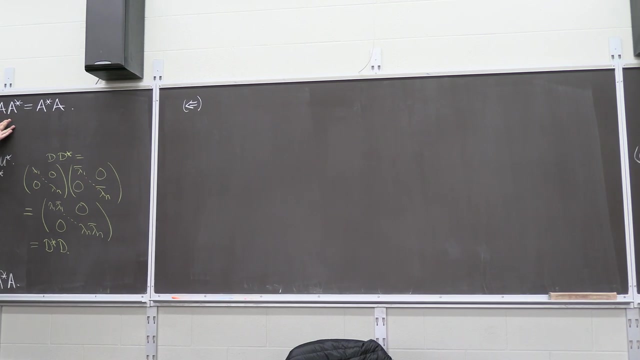 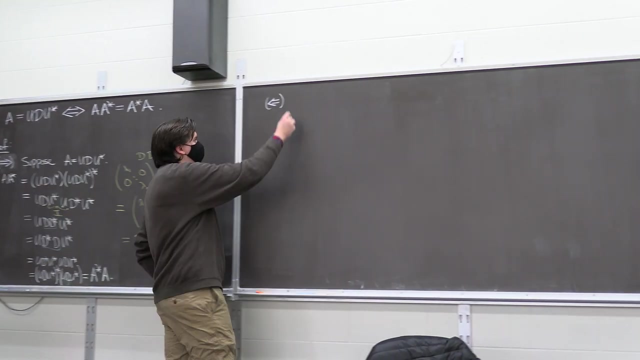 for real numbers. right, I'll just call it the spectral theorem for now. So let's finish our proof a bit. Now we want to prove the other direction. We're assuming our matrix is normal. We want to show that we can write it this way. 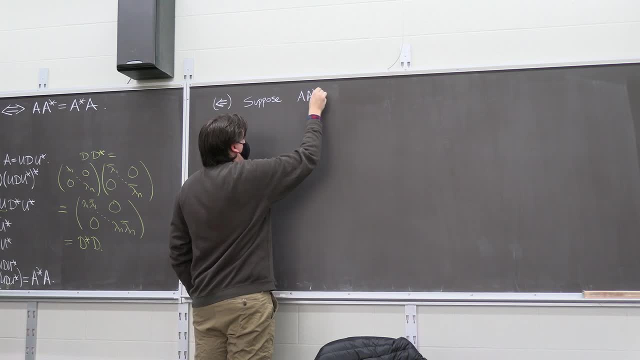 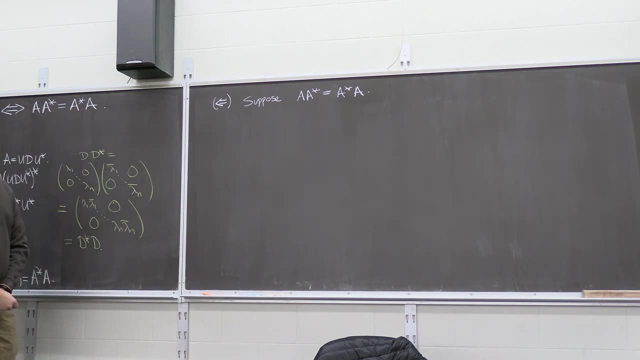 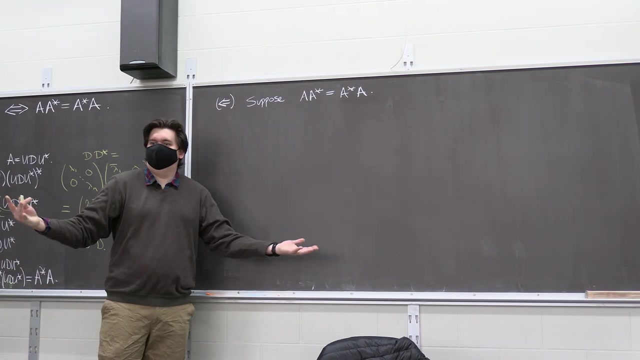 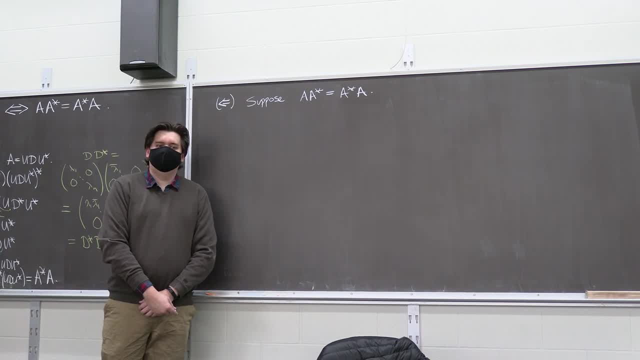 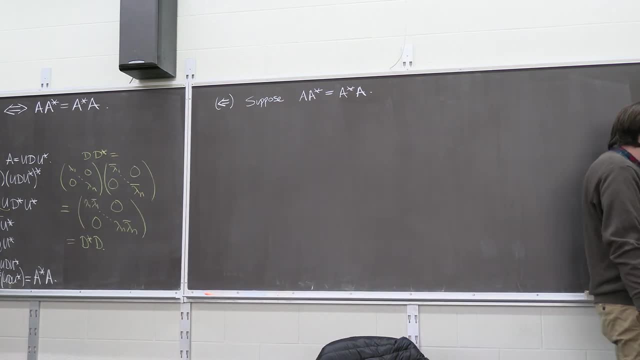 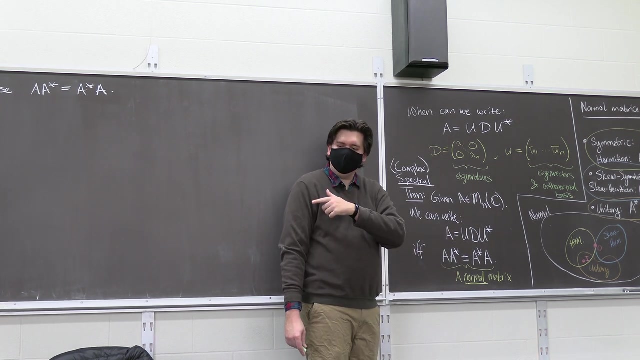 What can we unpack here? What can we unpack here? I don't have much to work with. I'm trying to show what comes out to be of the special form, Ah, but I know it's a complex matrix, so I know our results from last time still hold. 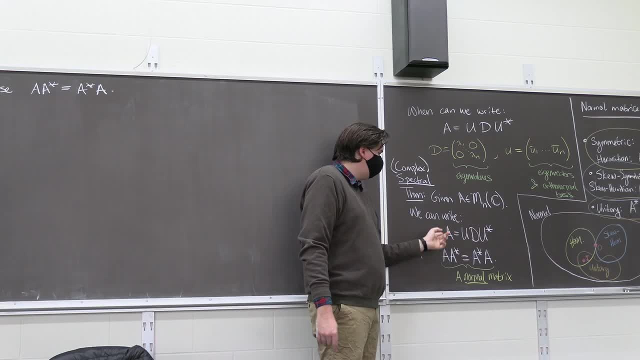 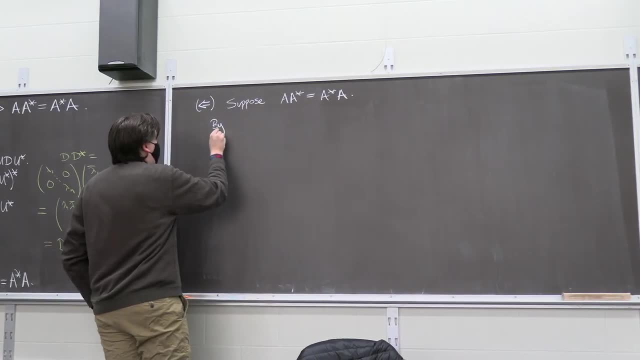 I can still do sure, triumphalization: I may not know what comes out to be of this form, but I know it comes out to be a former, at least the middle guy's triangular right. Bye, Bye, Bye, Bye, Bye. 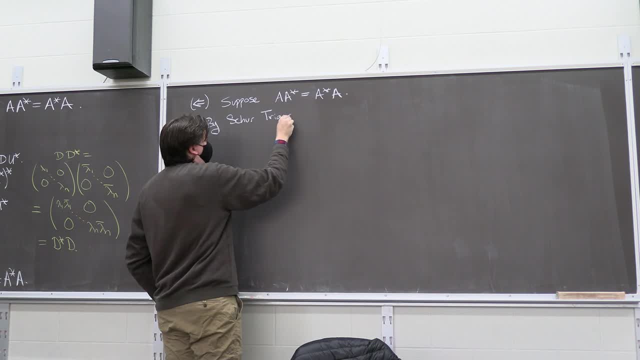 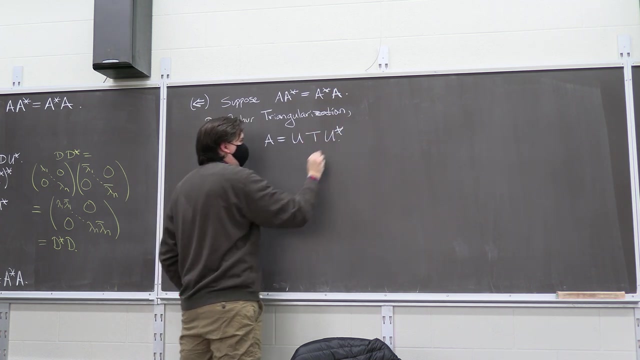 Bye, sure triangulation. really, what we're doing here, that's just a special case of sure triangulation, triangularization. but we prove this for all complex matrices A. we can write A as some unitary matrix times an upper triangular matrix, times u star. And so now what we just need: 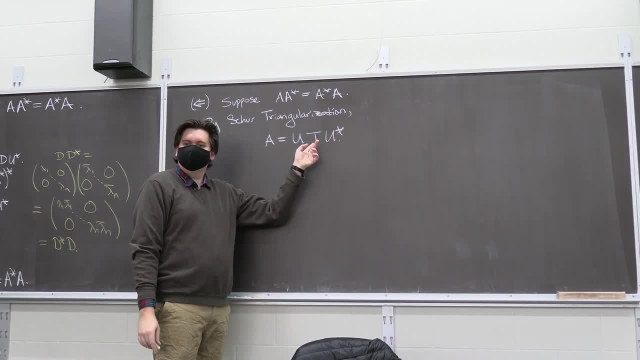 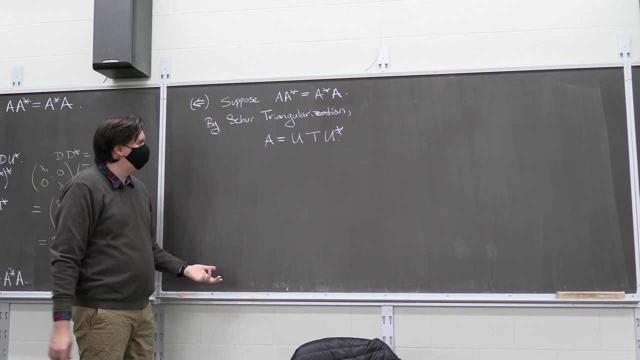 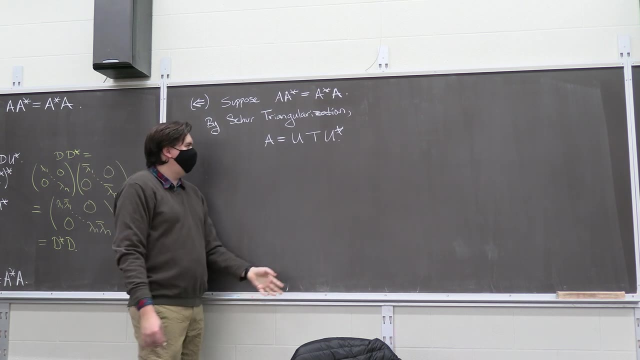 to argue is that that T is sequelae diagonal matrix right Now. this condition is going to force T to be diagonal. But now the proof's just going to write itself. It's like: well, A looks like this, so let's plug that in and see what we can get out, and we'll try and argue that we end. 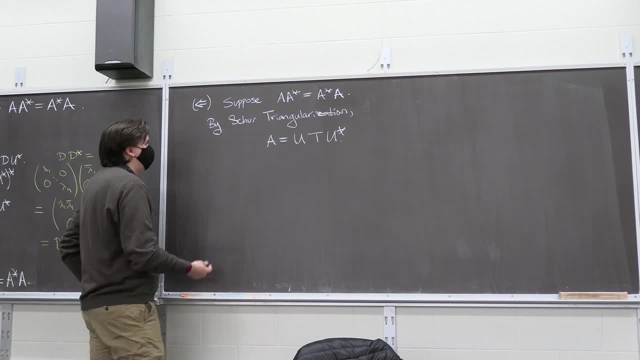 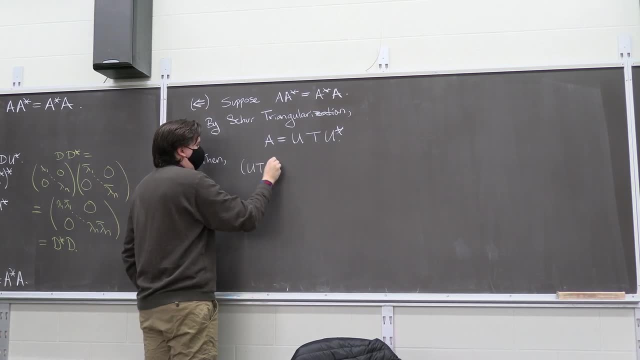 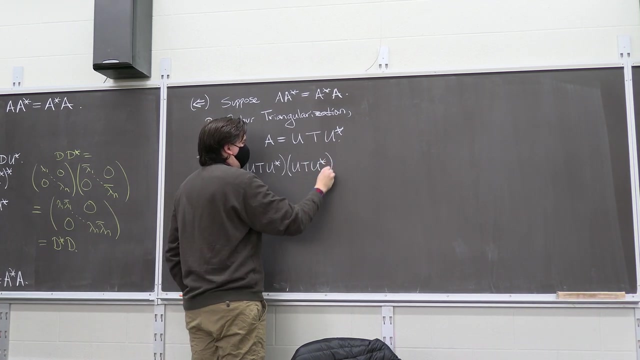 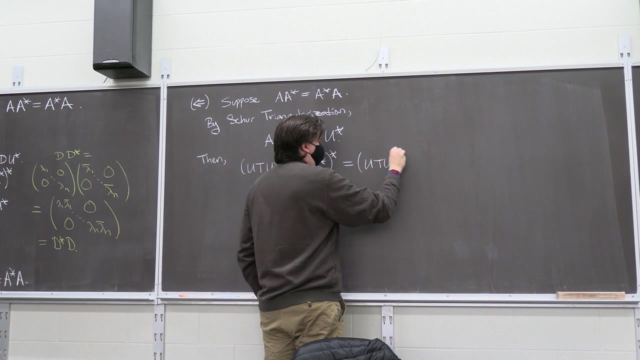 up with T having to be diagonal. So here we go, Then. A, which is u T u star times A conjugate transpose. so u T u star conjugate transpose will come out to equal A star u T? u conjugate transpose, conjugate transpose. 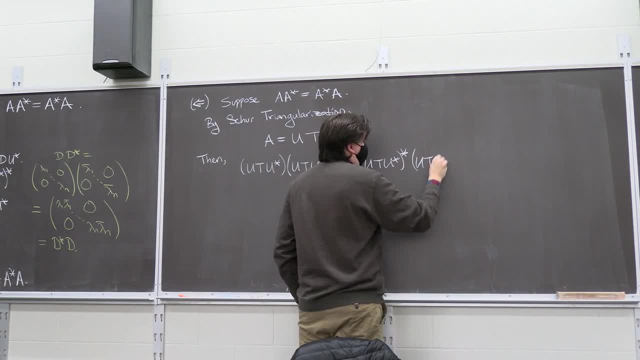 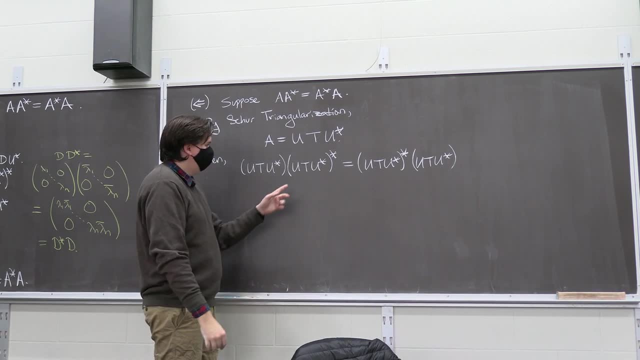 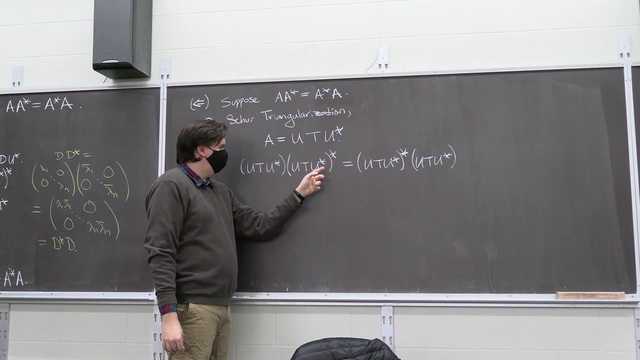 times A u, T, u conjugate transpose. Let's just begin simplifying, just like we did to the left. I mean, we already know how this is going to work. right? This is going to become a u, T, star, u conjugate. transpose The u and the u star. cancel. giving you here just a u. 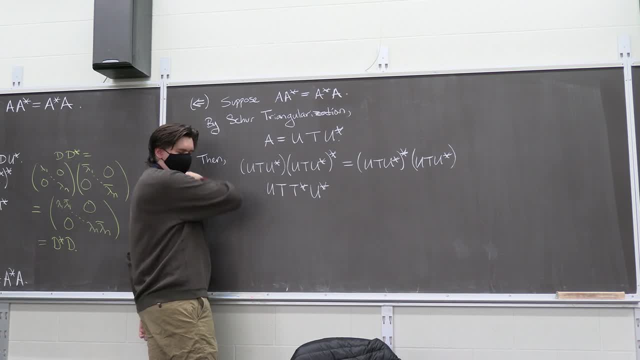 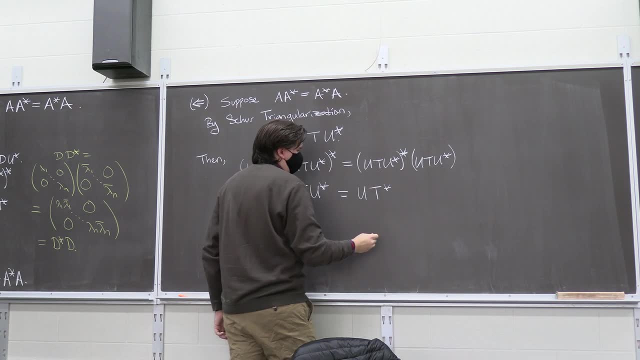 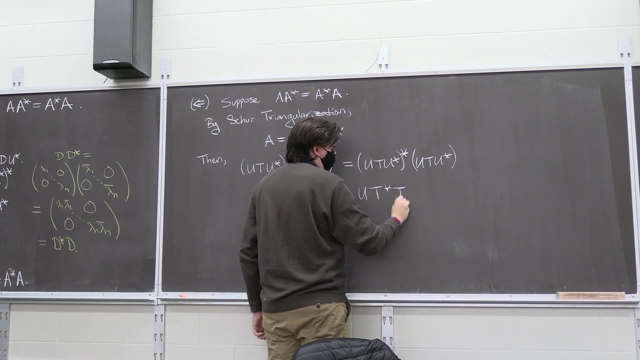 T, T conjugate transpose. u conjugate transpose, just like we had on the left And here it's somewhat similar, except we have u T conjugate transpose. That u will cancel with that u. That u conjugate transpose cancels with the u. So times T times u conjugate transpose. 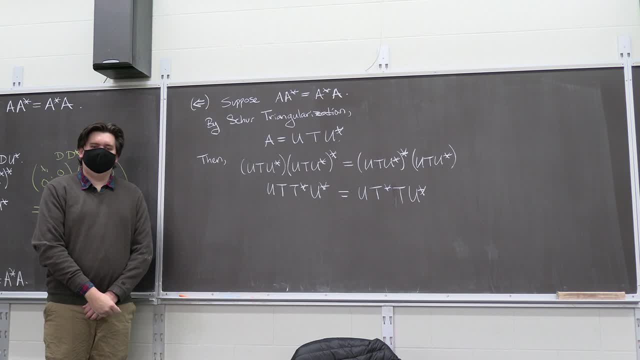 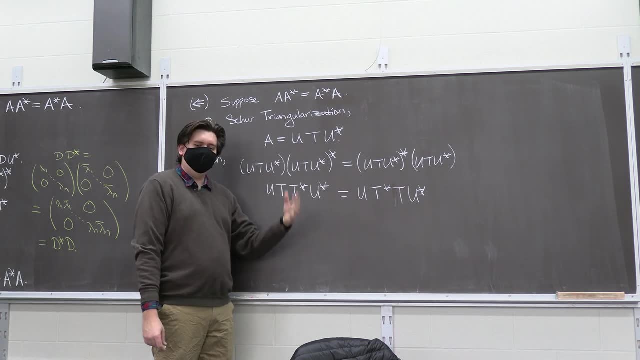 Then multiply both sides on the left by u conjugate transpose to cancel that u. So u T? u conjugate transpose. That's just the way those two things work: The? u and the? u star. that's the way those two cancel that U and multiply both guys on the right by U. 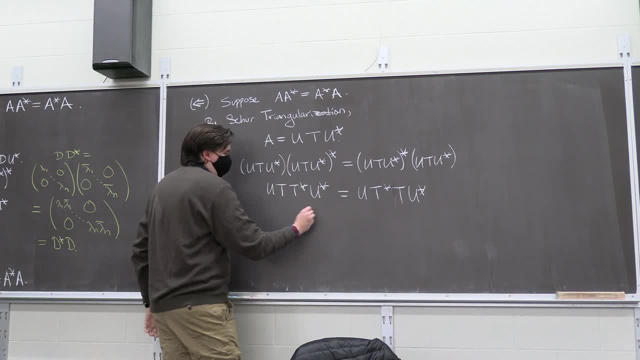 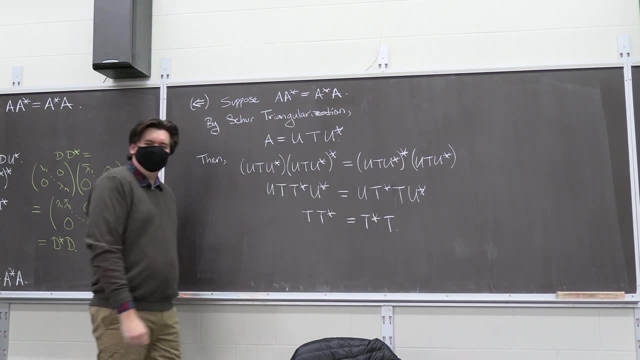 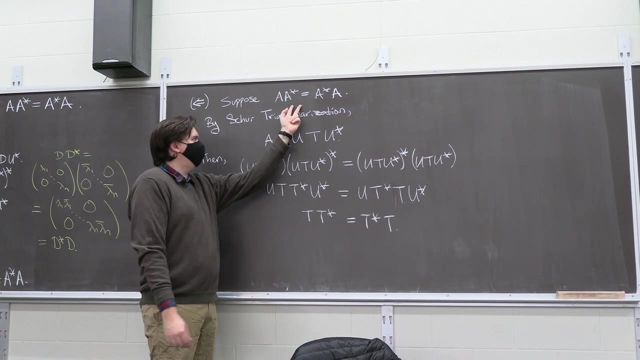 to get rid of the U inverse, the U conjugate, transpose and you have that T T star is T, star T. So, once again, the power of short-triangulization is it. lets us move from some fact about matrices to some fact about triangular matrices. 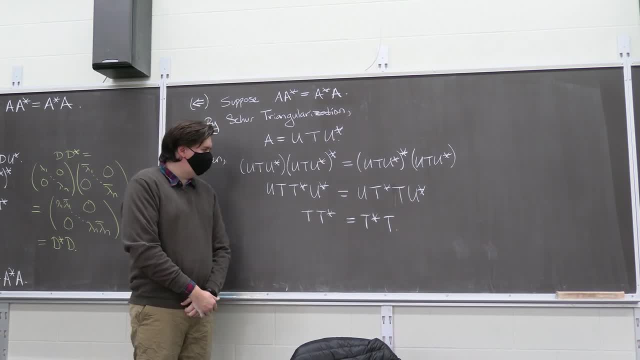 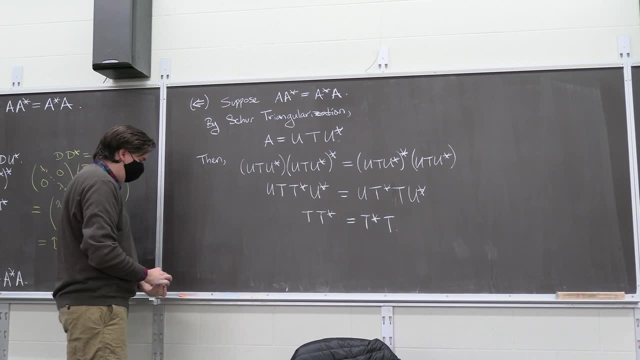 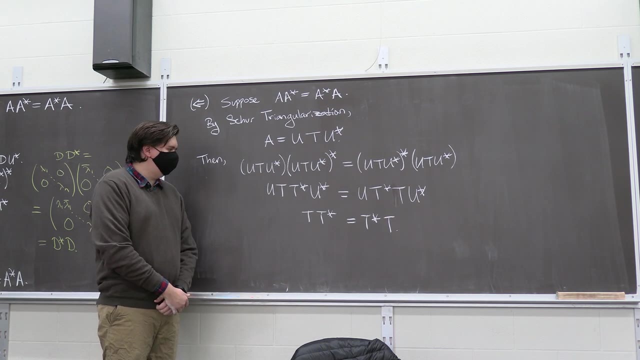 Upper triangular matrices. And now let's take a second to think what this is really saying. So I need to maybe draw a picture of what T looks like. So I can do this in general and that would be fine, but I think what I'm gonna do is just do. 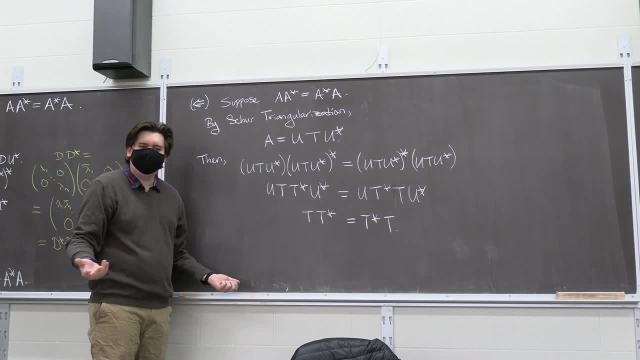 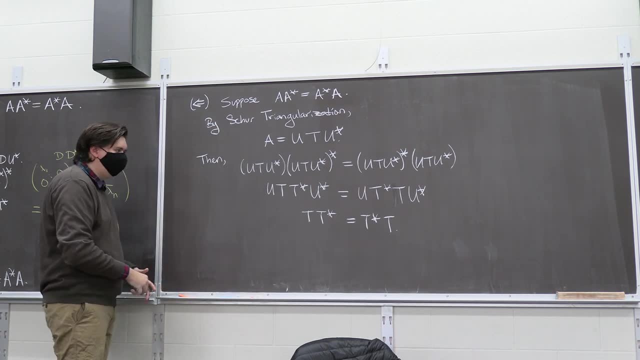 with a three-by-three matrix and you'll see how the proof works with a three-by-three matrix. and then, if you wanna do it in general, you just add a few dots and change the three to an N right? But I think for concreteness I'm just gonna do this. 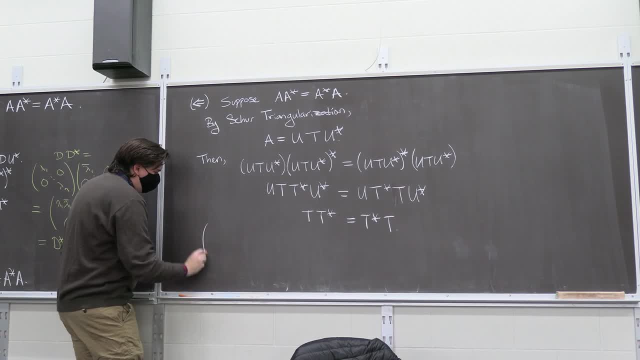 with a three-by-three matrix, So T just looks like some guy. well, maybe I'll give him some indexing that makes sense, like I'll call it T one one, T one, two. T one three, zero T two, two, T two, three zero, zero. T three three. 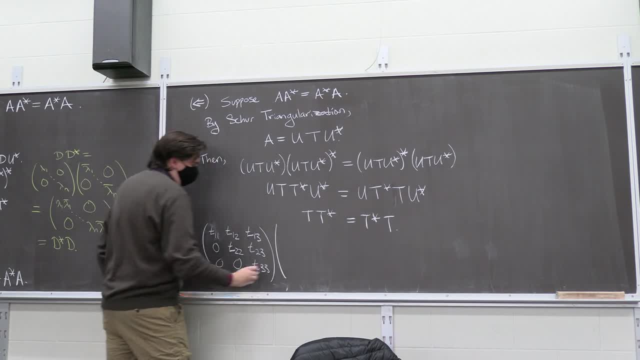 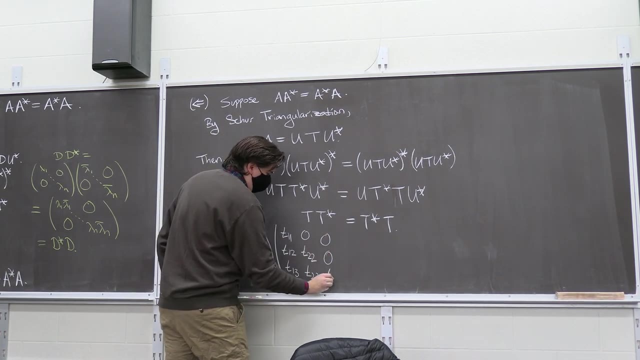 That's T. so T conjugate transpose is: the transpose is: T one one, T one two, T one three, zero, T two, two, T two, three, zero, zero, T three, three. But also I need to take the complex conjugate. 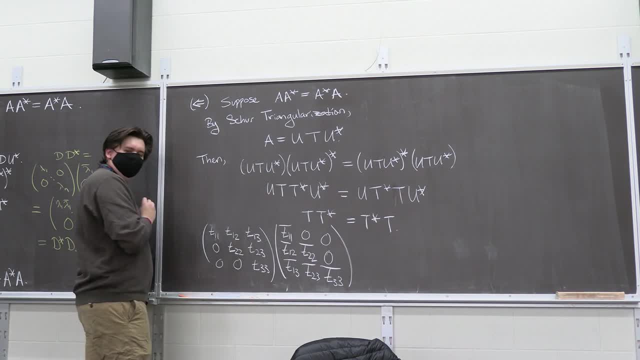 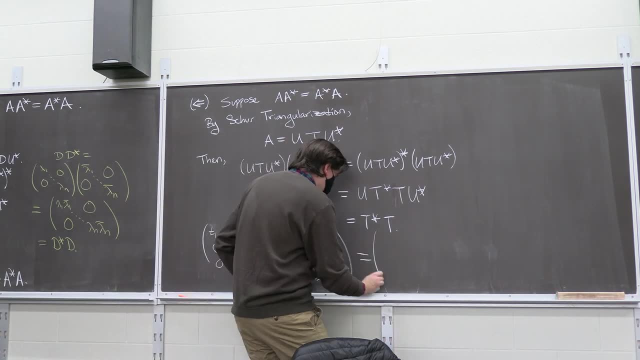 so these may be complex numbers. we're taking the complex conjugates And then on the right it's the same thing, but in opposite order. I wish there was a copy and paste option for blackboards, But here we go. One one, zero, zero. 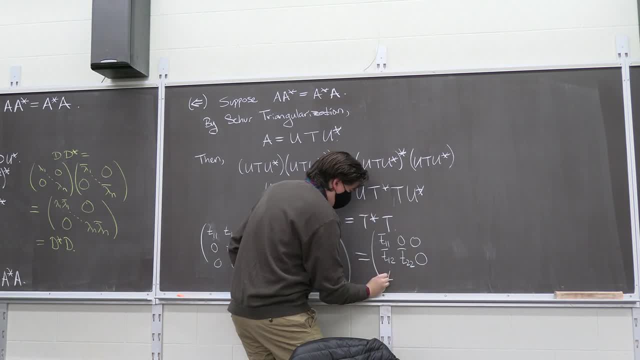 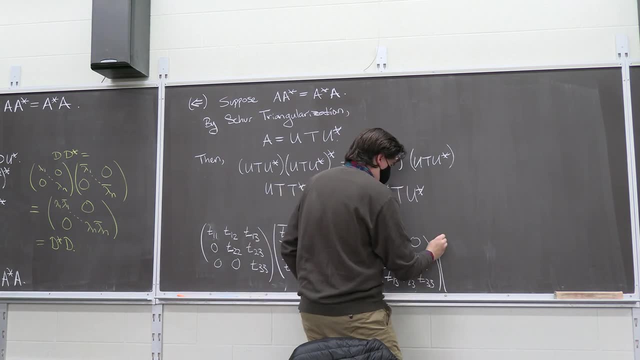 T one, two, T two, two, zero, T one, three, T two, three, T three, three times T one. one. T one, two, T one, three, zero T two, two, two, two, three, zero, zero, T three, three. 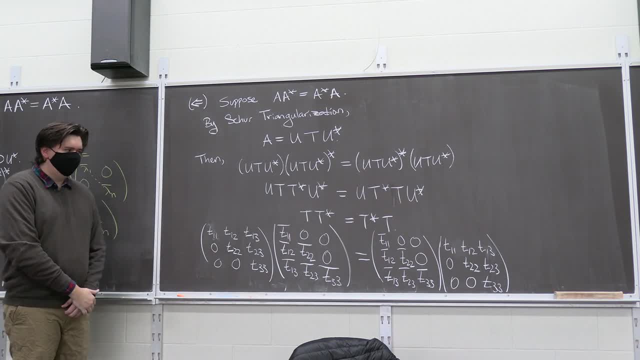 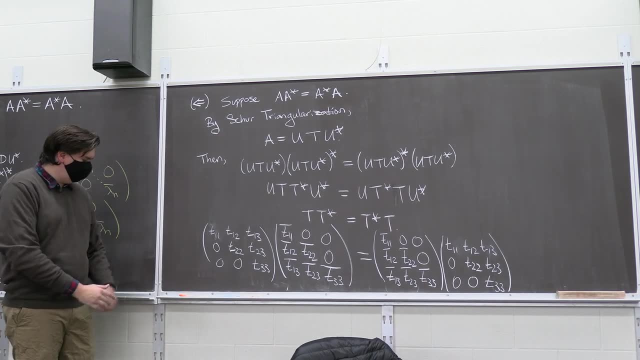 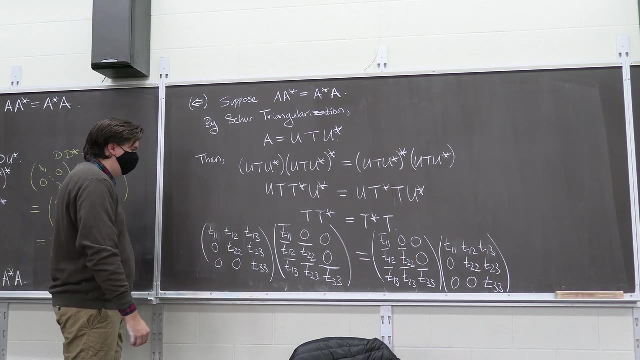 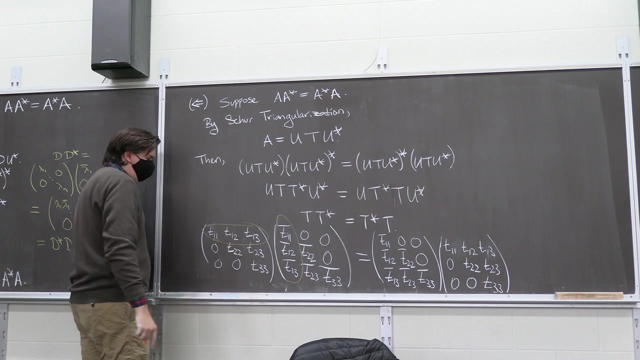 Whoo, I think I got it right. Okay, let's start digging into this guy. What is the upper leftmost entry of this guy on the left when we multiply this out? Well, it's gonna be row times column, So the upper leftmost entry will be T11. 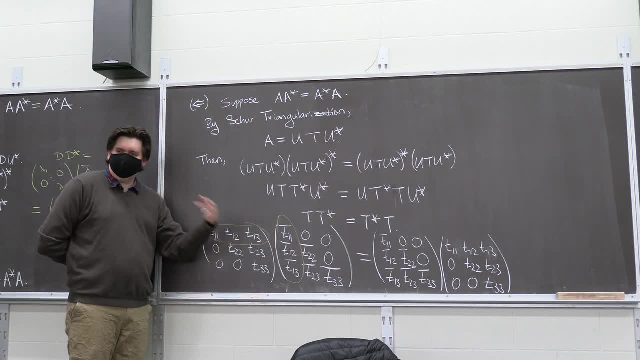 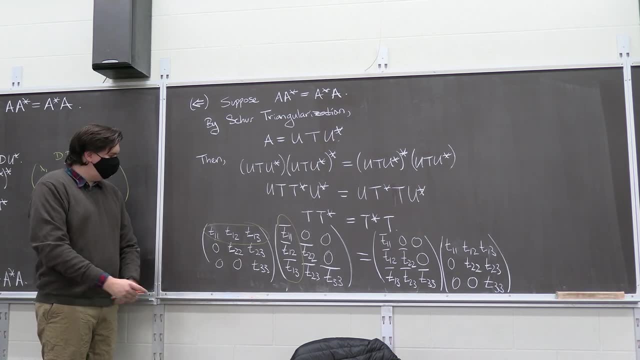 times its conjugate transpose, plus T12 times its conjugate transpose, so on. If there were N of these, those would be N right. You can do this in general, But remember a complex number times its conjugate transpose is just the norm. 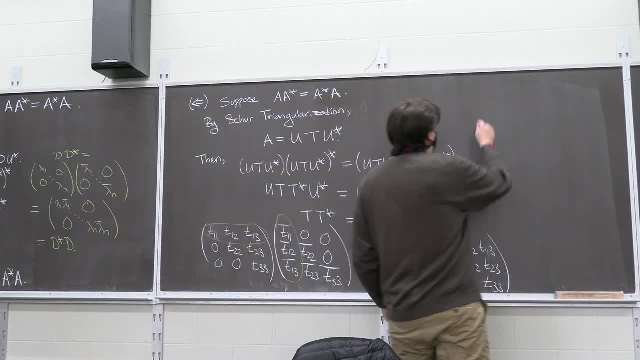 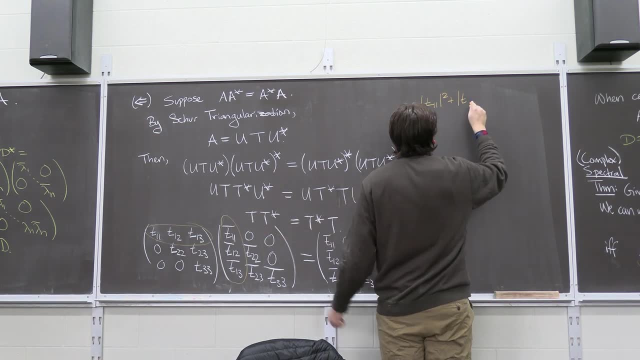 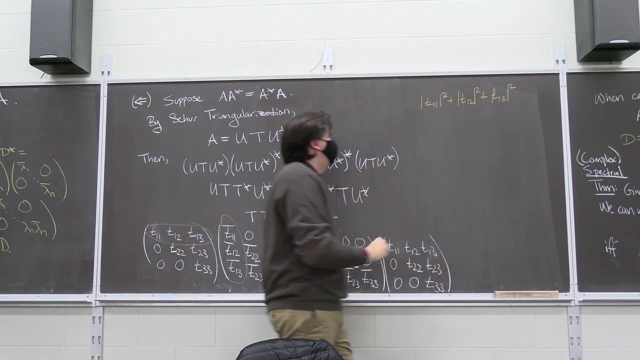 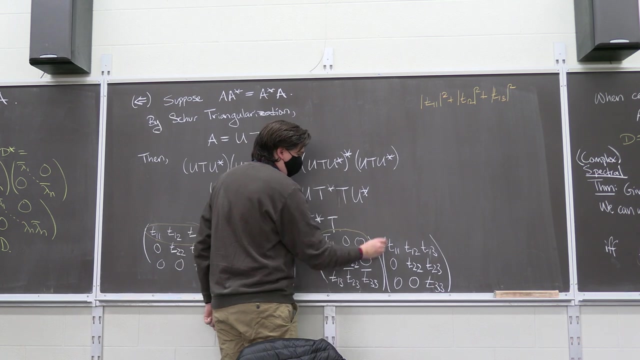 of that complex number squared. So this will just come out to be T11 norm squared plus T12 norm squared plus T13 norm squared, Whereas here on the right, when we do row times column, all we have is T11 norm squared. 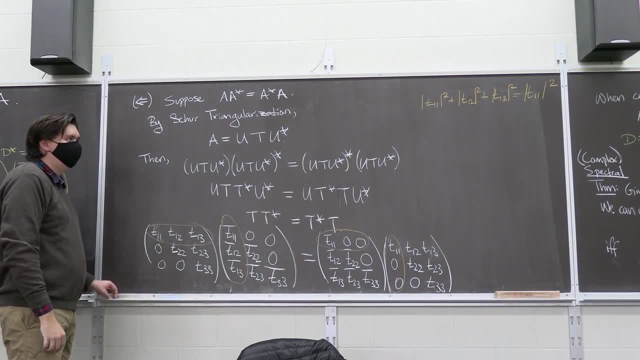 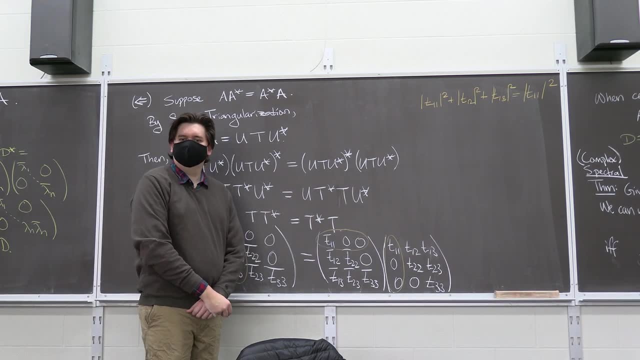 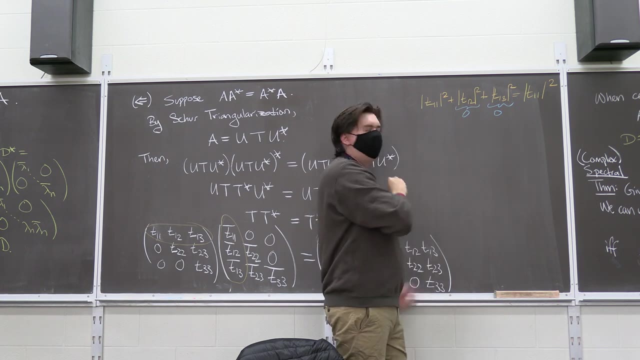 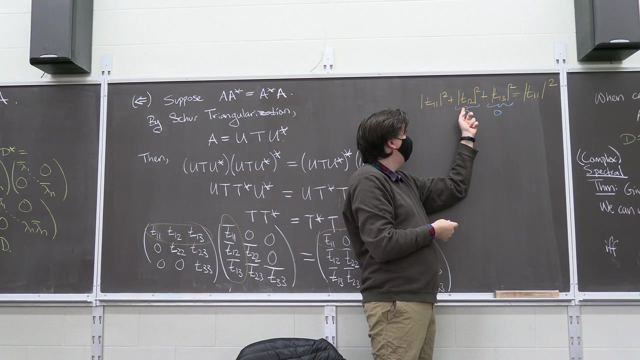 What does that tell you? These both must be zero, Right? These are equal, So these values have to be zero. They're not negative, right? Because it's something of the form of A squared plus B squared, So it's not negative. 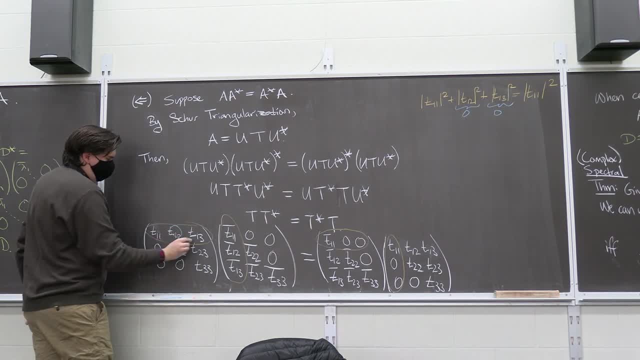 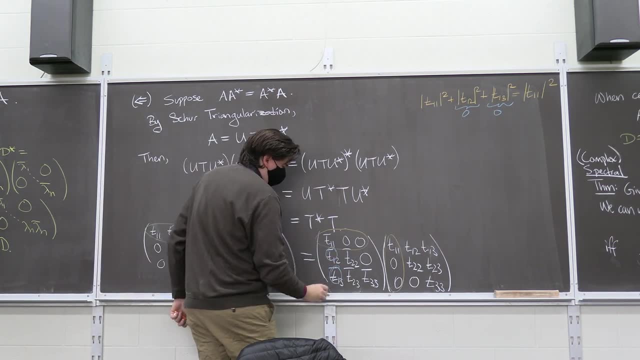 So they must be zero. So we just showed: actually this guy is zero, this guy is zero and hence also his complex conjugate is zero. So we just showed all those values as zero. And then you know, like in the general, 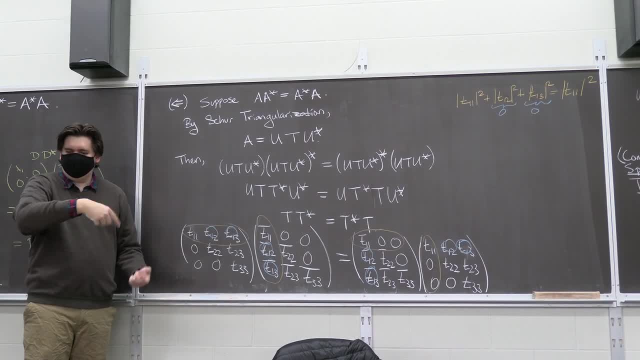 if it's like an M by N matrix, you just keep going through this And you just see the rest will fall out. I mean, we'll do one more row. We only have to do one more row here. We only have one value left to show that it's zero. 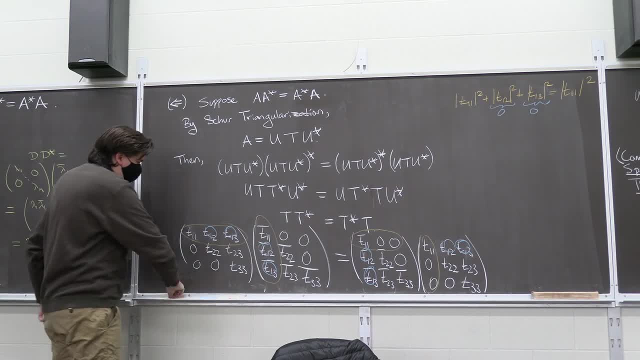 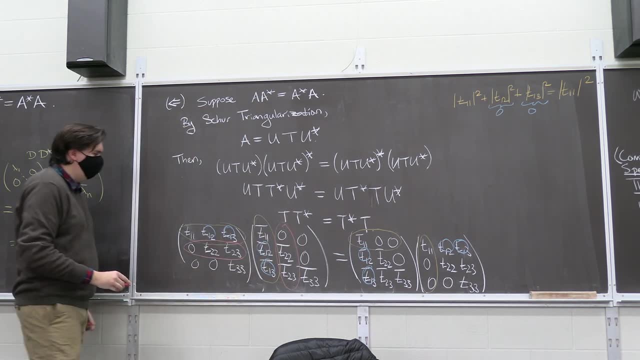 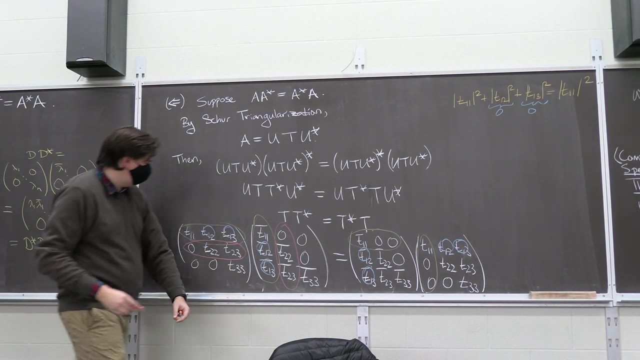 But in general you just keep going. So let's go ahead and do the next one now. Second row times, second column. What does that give us? Zero and zero, T22, T22, and T23 and its complex conjugate. 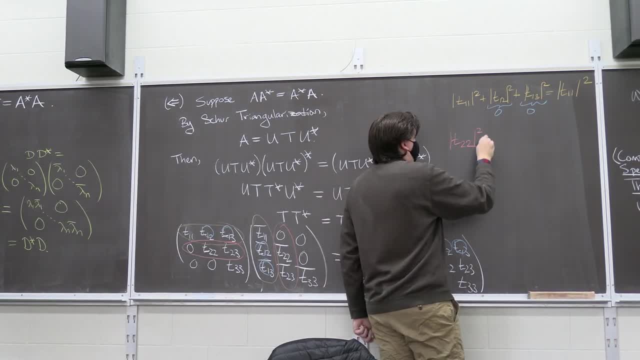 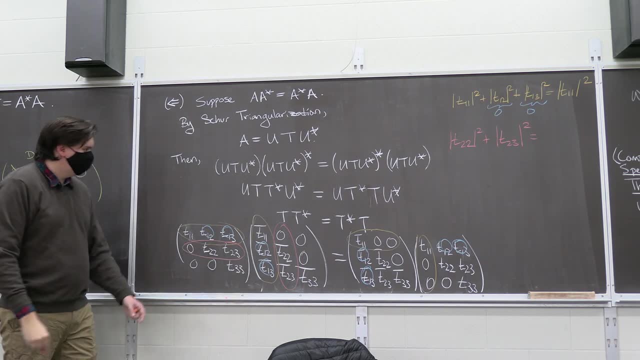 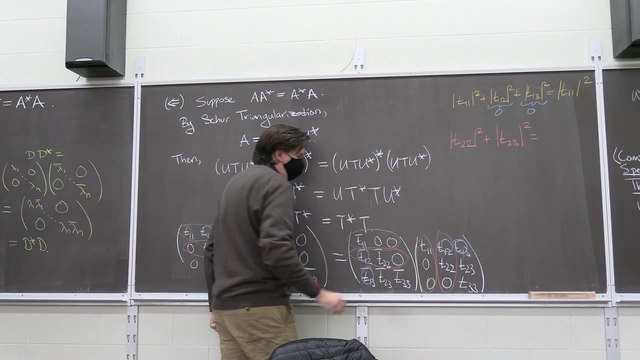 So we get T22 and T22.. And then what do we get on the right? Here's where the previous step's going to help us. This row times this column: Ah, since we now know this value is zero, you end up with just T22 times its conjugate transpose. 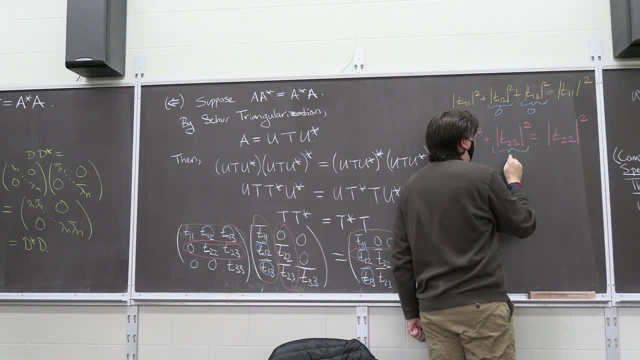 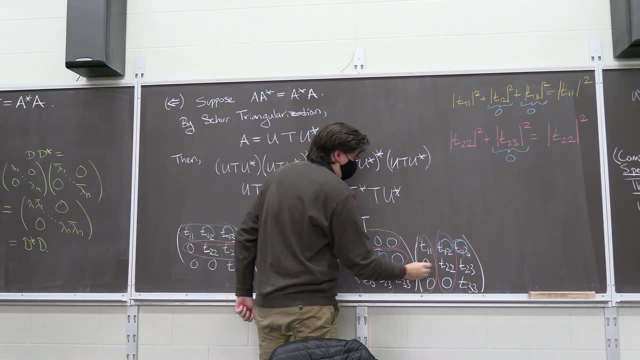 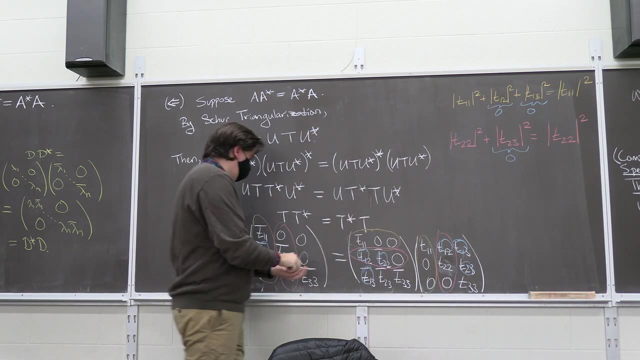 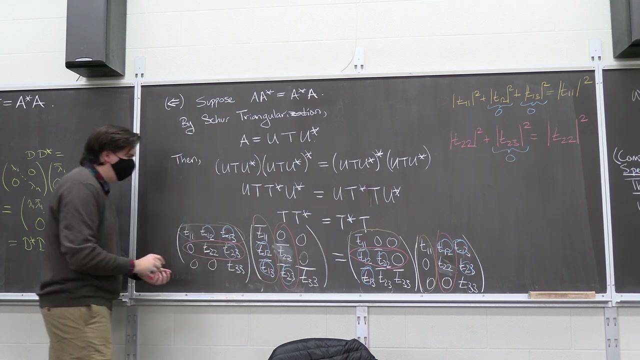 And thus you conclude, just like before, that T23 must be zero. And so you get: the T23 is zero. Oh, no, That's not zero, that's T22.. Oh, Made the same mistake twice, Almost made it thrice, okay. 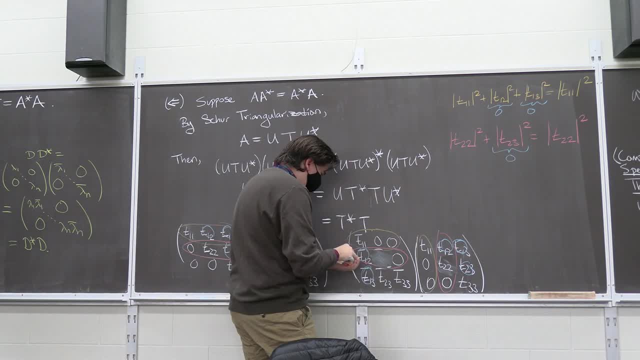 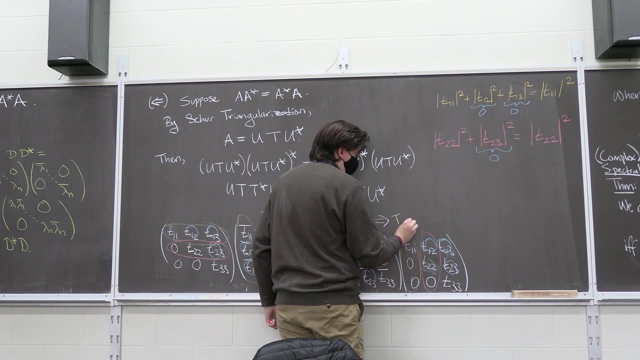 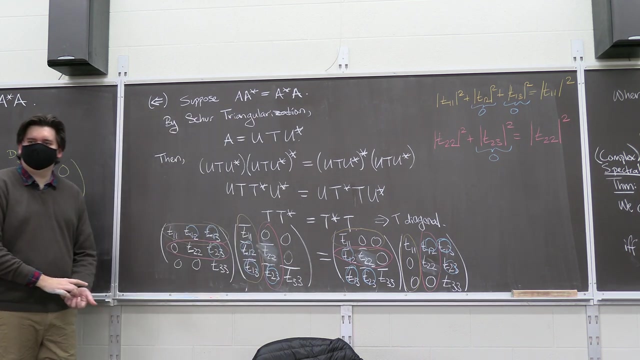 Oh, It's T23, that's zero. It's just so easy to get this wrong. Okay, And so you left that T is actually a diagonal matrix, Right. hence this gives you T is diagonal. Okay, like I said, you can do this in case. 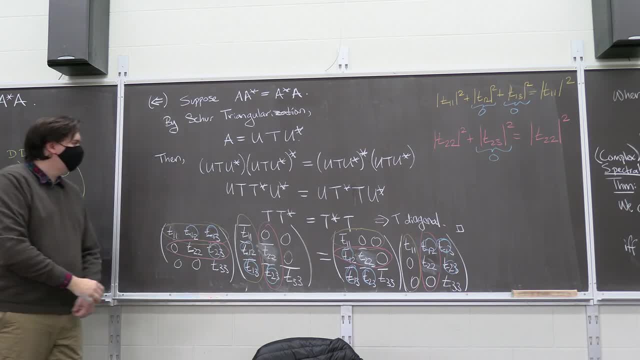 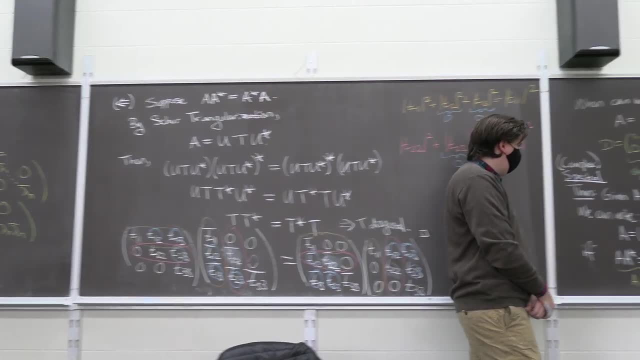 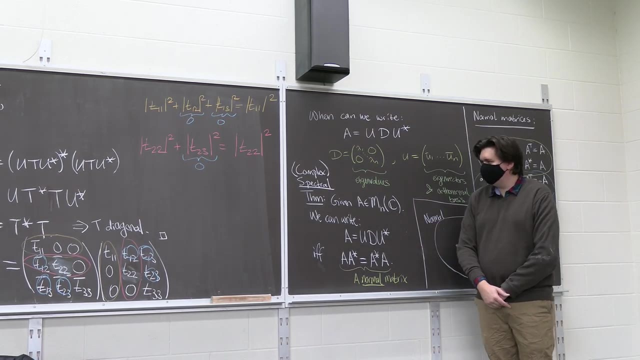 It's just a little bit keeping track of your indexes, which is a little bit messy, Okay, So maybe we should wrap up today by actually looking at an example of calculating this Right. We'll see it has lots of nice properties. 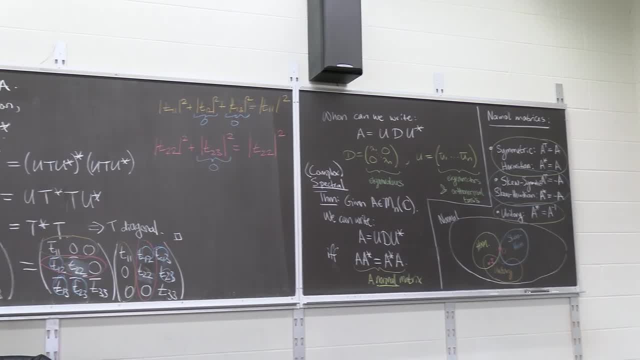 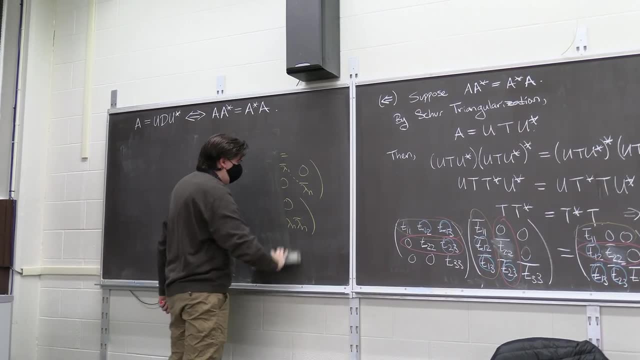 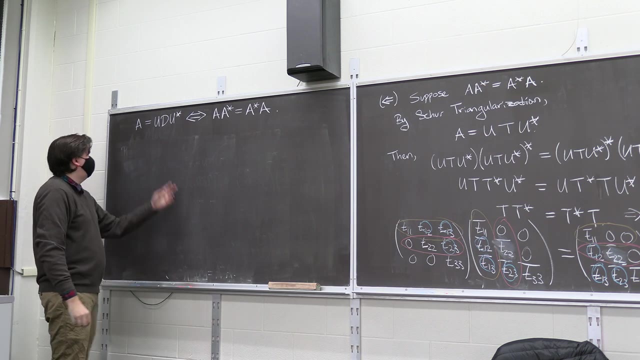 but let's just get a very concrete example. So I need to begin by picking some matrix that's normal, so then you can be confident that in fact there exists such a decomposition. Well, how do I find a normal matrix? I could try and manufacture one. 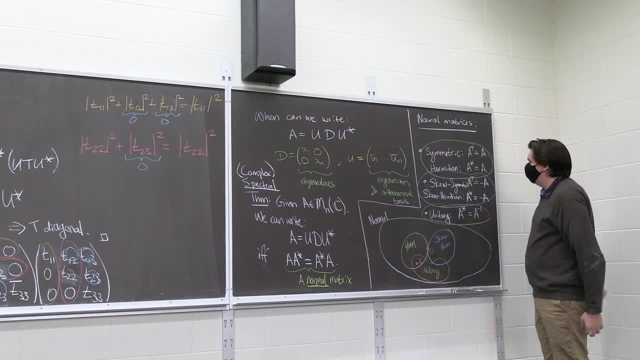 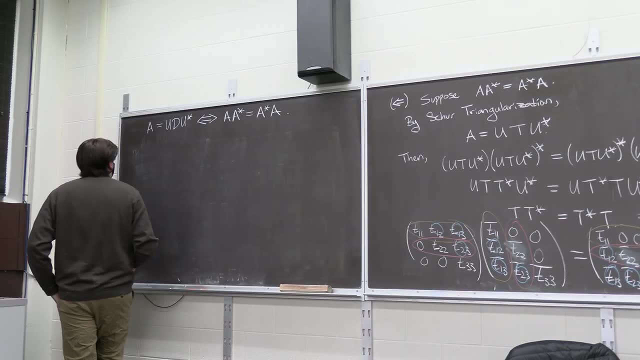 but I can just pick any of these kinds of matrices in particular, and I'll know it's normal. So let me just pick a symmetric matrix. Let me just do it with real numbers, right? I'll just keep it really simple. So, for example, let's just do something like: A is. 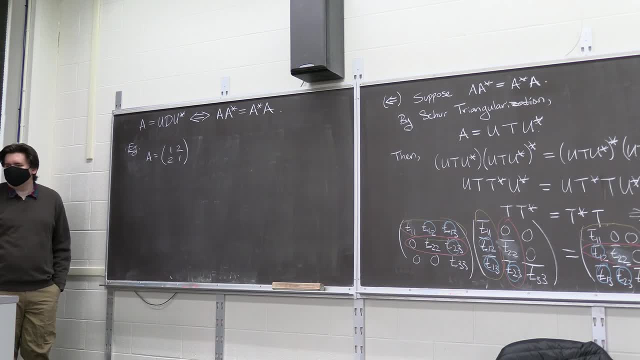 one, two, two, one Symmetric matrix. hence it's a normal matrix And you can verify that this times its transpose is equal to its transpose times itself. So how is this going to work? Well, maybe we should stop and think a little bit. 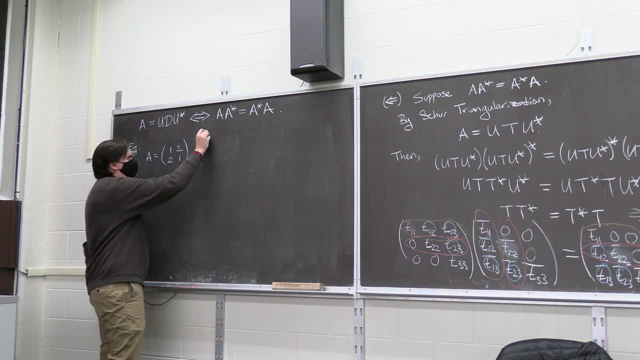 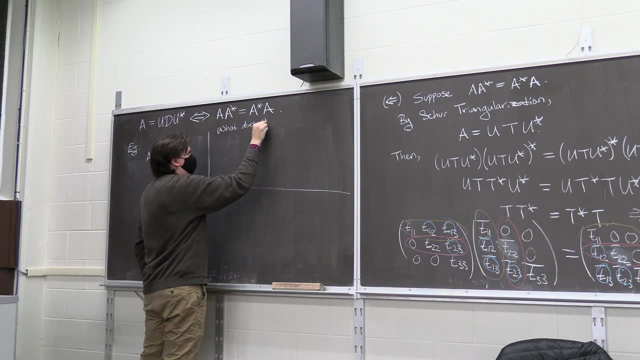 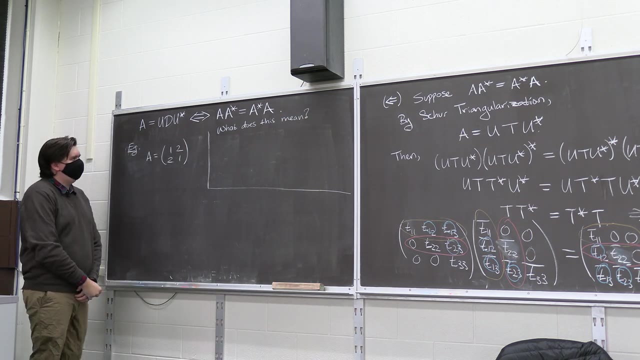 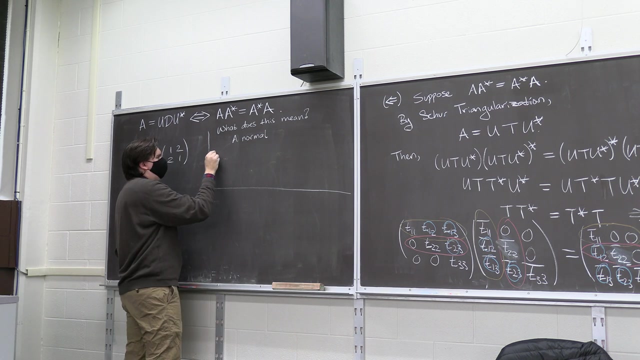 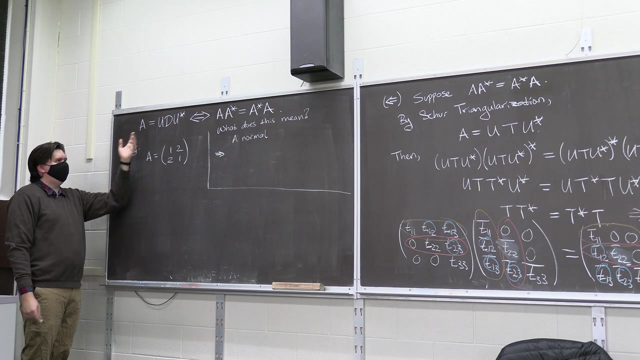 about what this theorem is really telling us. So, like, what is this saying? Well, one thing it means is that if A is normal, then that means there exists some collection of eigenvectors that forms an orthonormal basis. Alright, so that's one way to think about it. 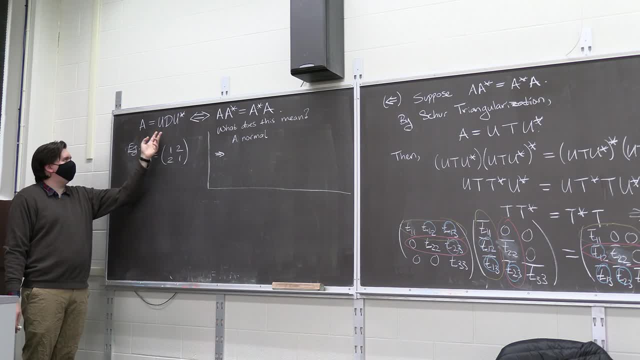 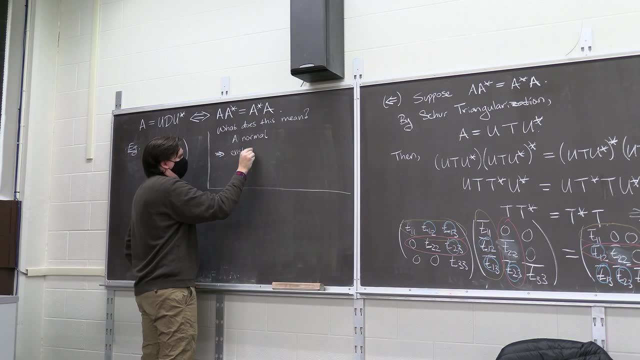 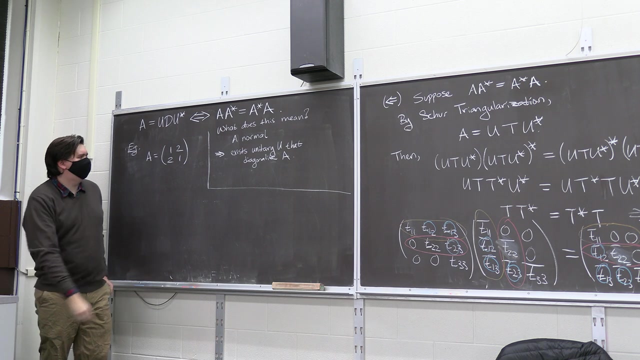 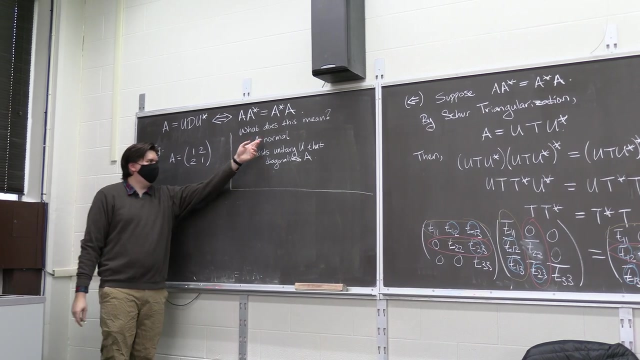 Another way to think about it is that you can diagonalize A using a unitary matrix. So you can. there exists a unitary U that diagonalizes A, But since the theorem goes both directions, it's not just that this is a one-way implication. 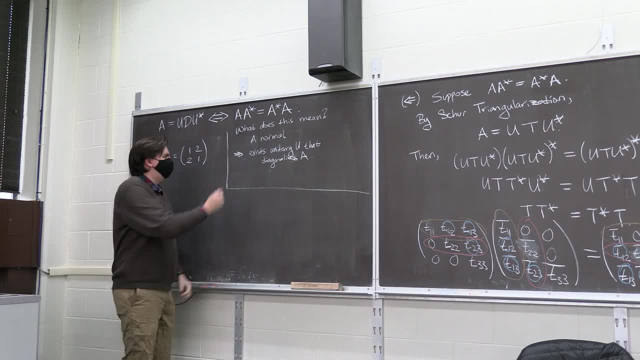 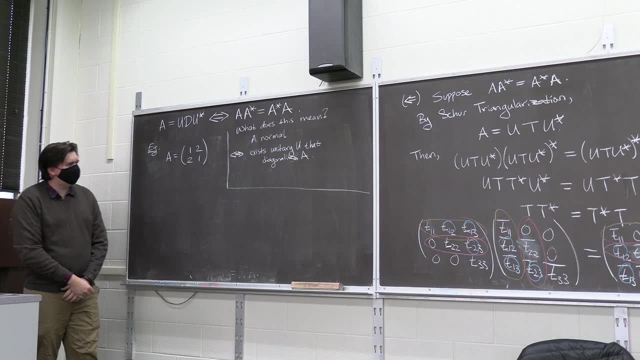 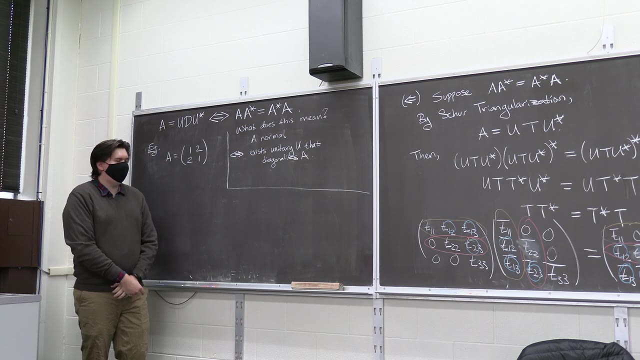 because if there exists some unitary U that diagonalizes A, the other direction of the theorem tells you that A is normal. But you look at this statement and it's their exist statement, And so you might wonder: like well, can you still diagonalize A? 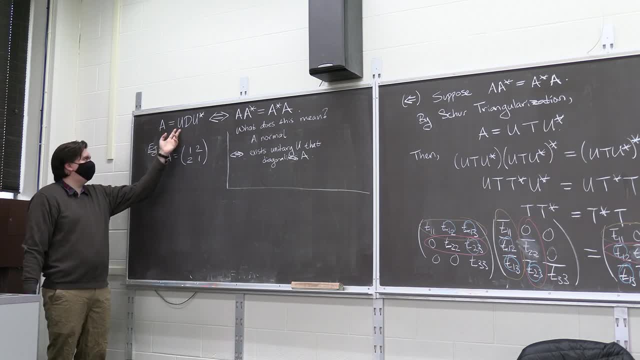 and end up with something that's not unitary, right, Like maybe some choices of like, a change of basis give you like a diagonal guy here. But you know what, if can you diagonalize using something other than something other than a unitary matrix? 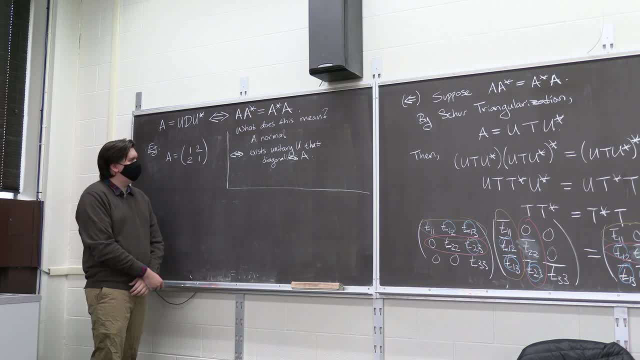 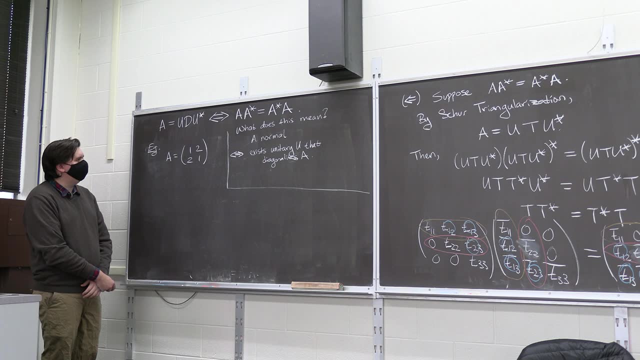 And the answer is no. So let's chase through the logic of this. Well, I guess it just falls out of the proof, right, That once you have your orthonormal, once you have your D is just your eigenvalues. 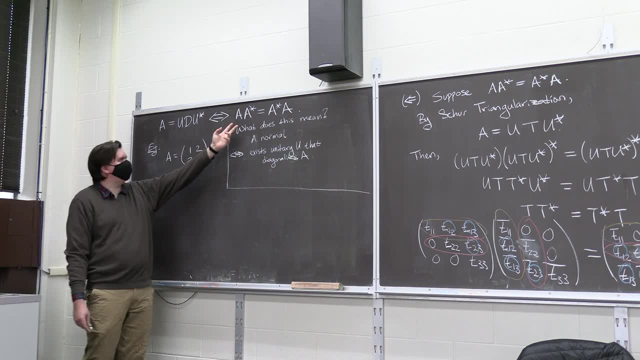 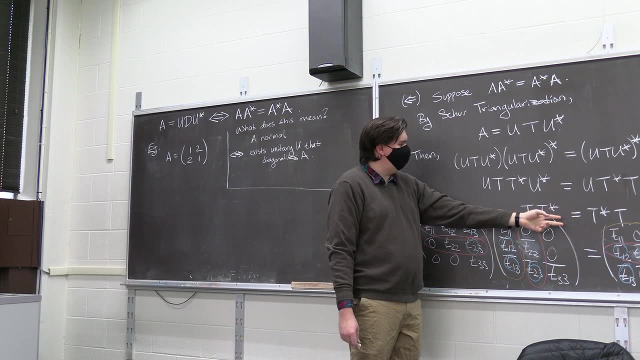 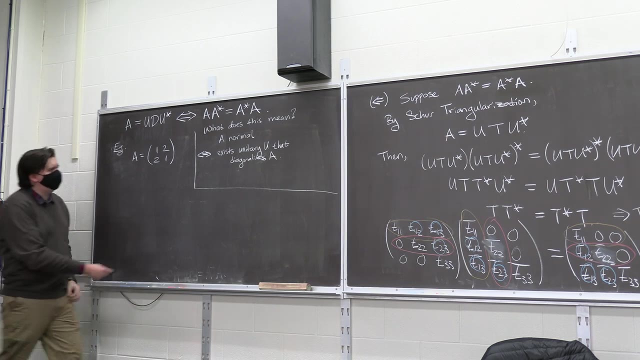 And so you just have from here that if A is normal- I mean, this is exactly where we showed here- If A is normal, that in fact this is gonna be diagonal, And so you actually get for free that, your orthonormal basis. 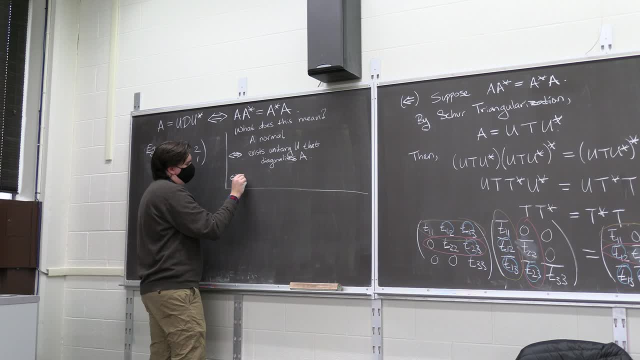 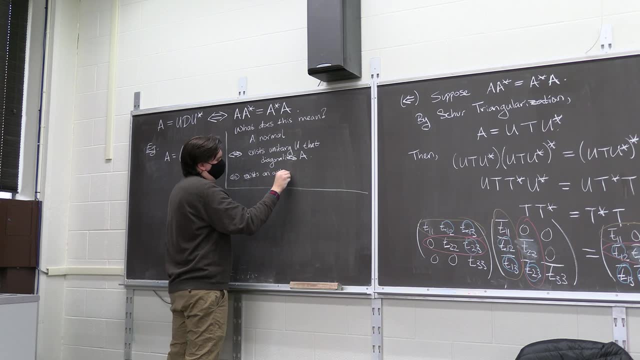 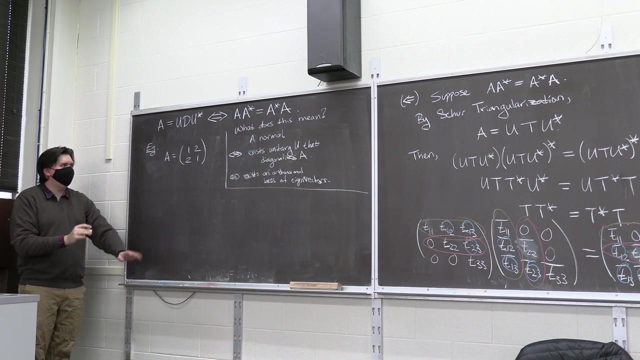 so another way of thinking about this is that your there exists an orthonormal basis of eigenvectors. So let me show you, like what this means, Like in practice. I'm just saying, if you wanna find U, you just find your eigenbasis. 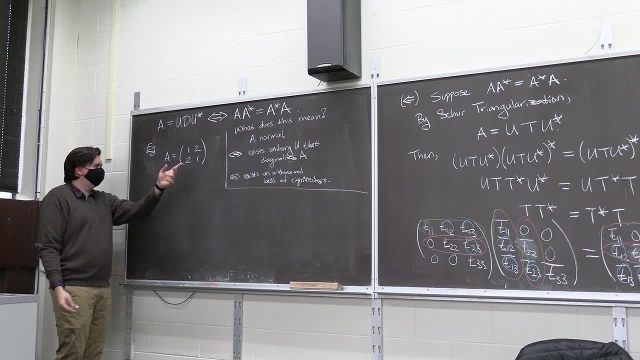 And you'll just fall out that it's orthonormal. So as long as you scale properly. So like here we go, Let's just find our eigenbasis, We're just gonna find. well, let's first find our eigenvalues. 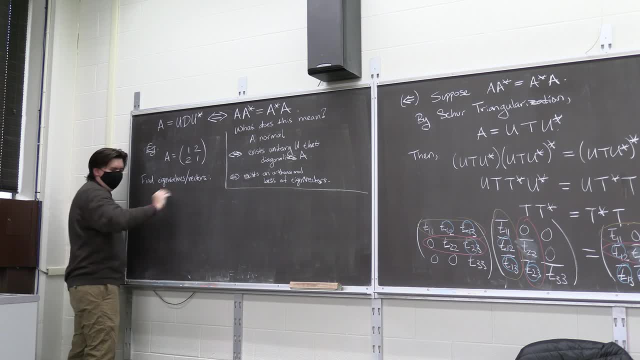 And then we'll find our eigenvectors And we're just gonna see that they just come out to be orthonormal, That this is really what this theorem is telling us. So you know, first we need to find the characteristic polynomial. 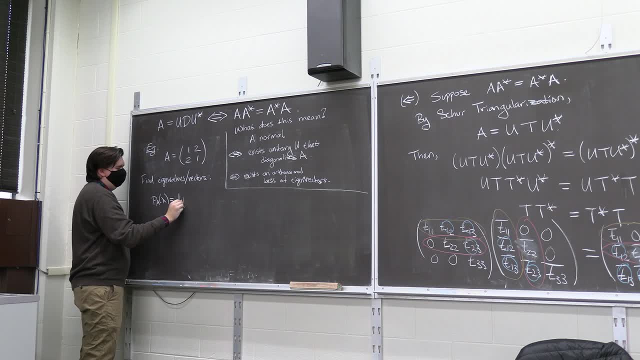 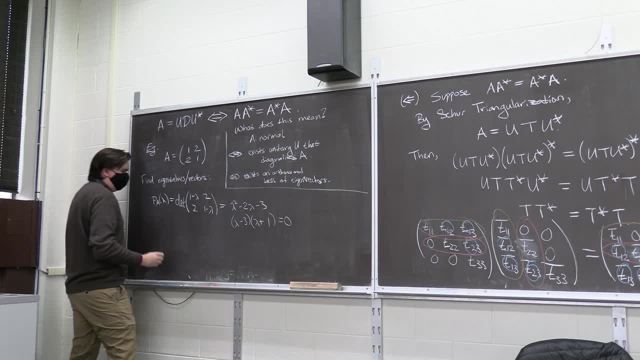 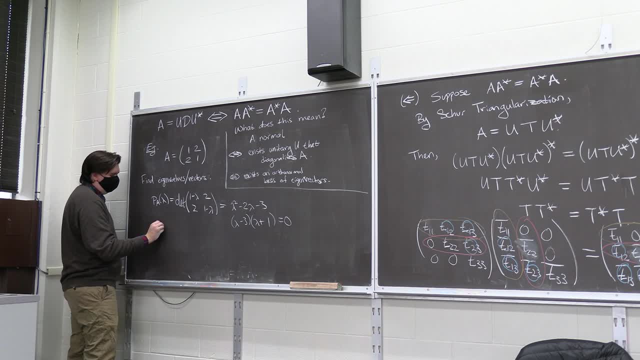 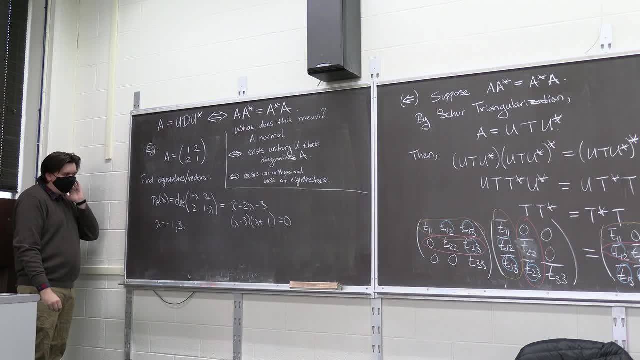 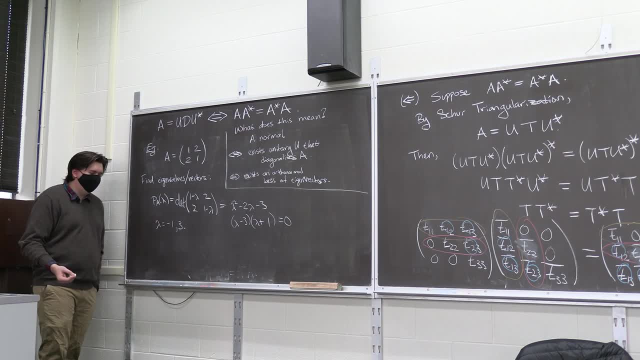 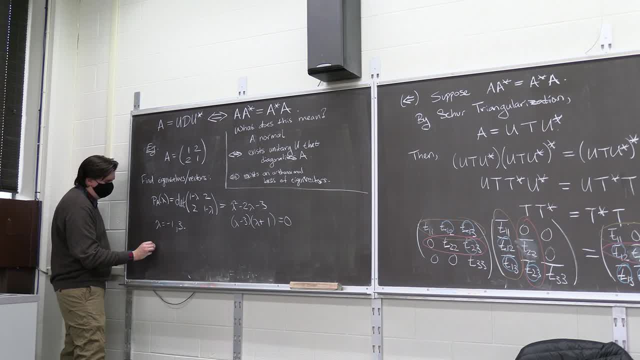 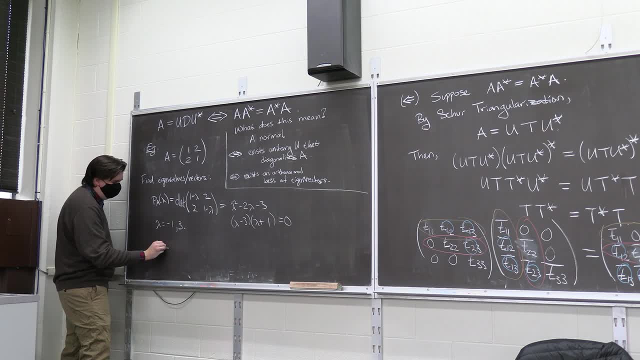 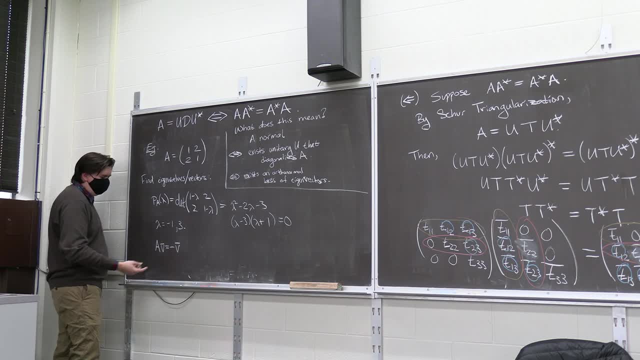 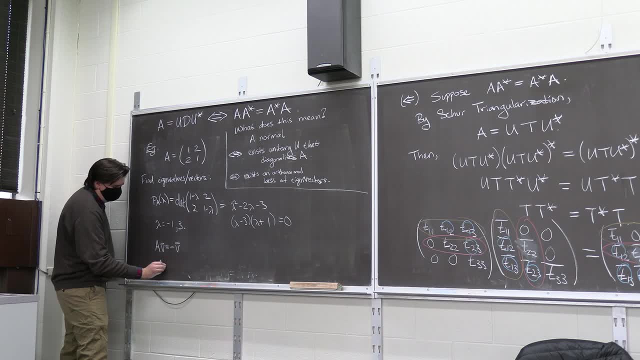 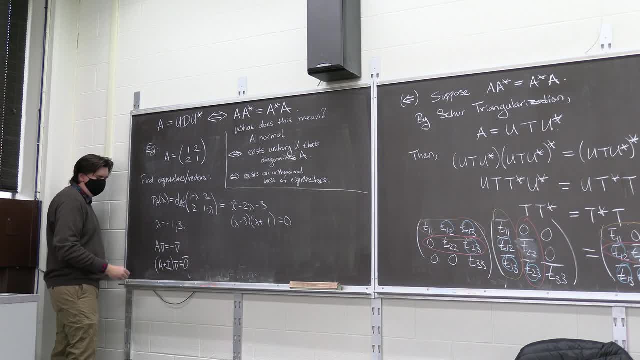 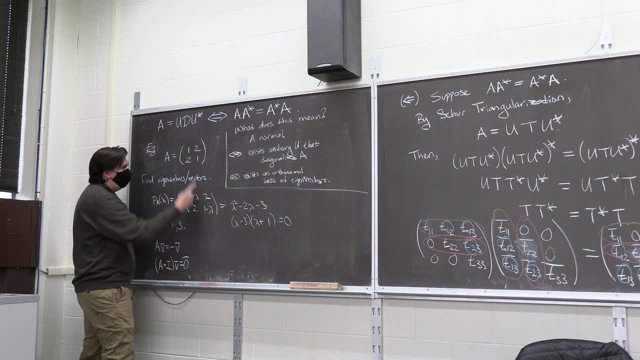 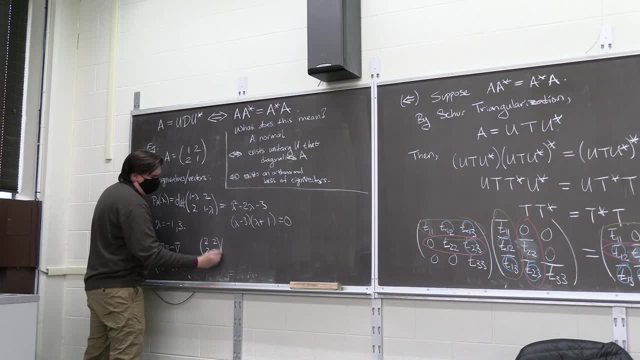 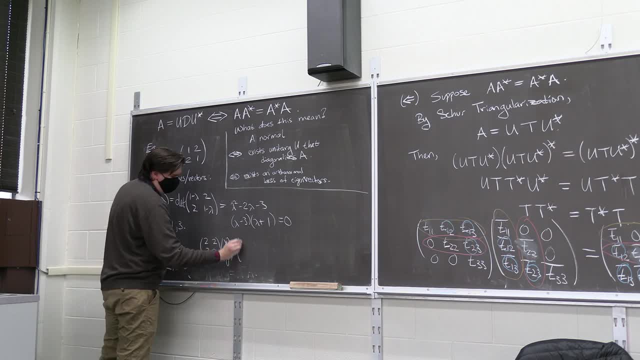 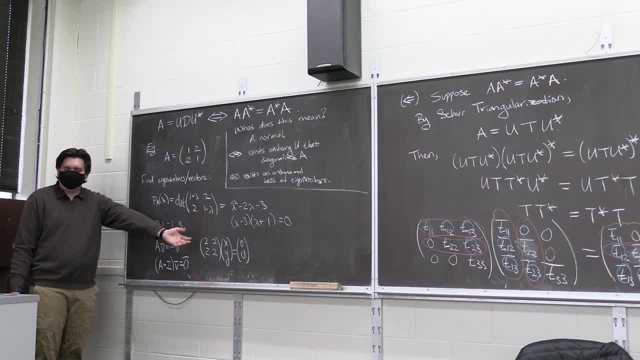 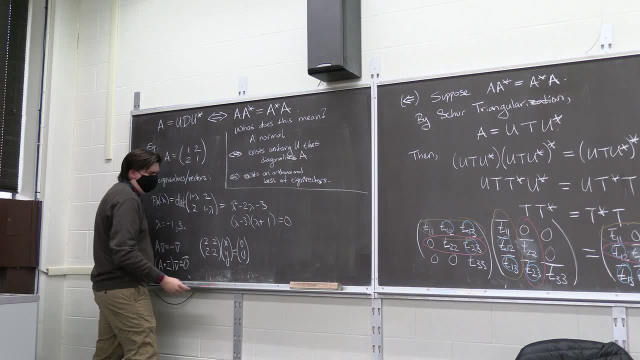 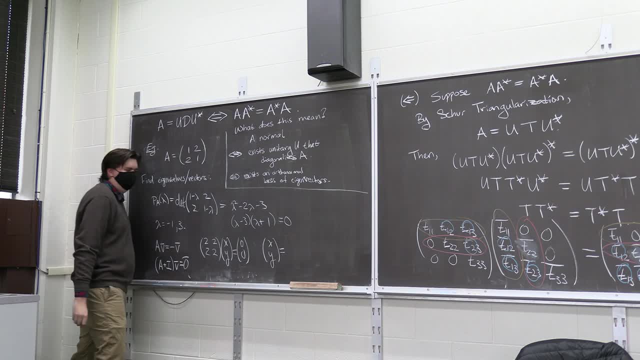 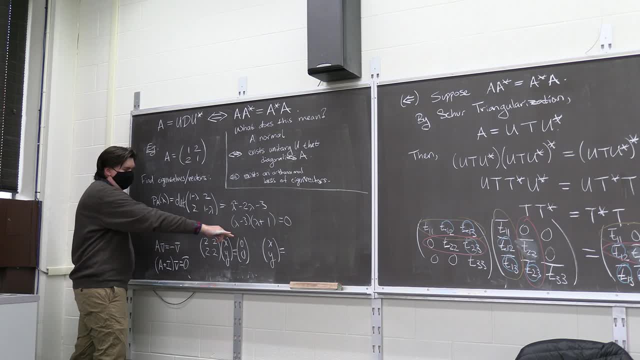 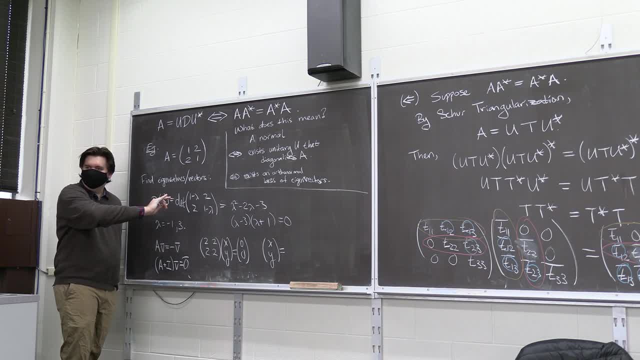 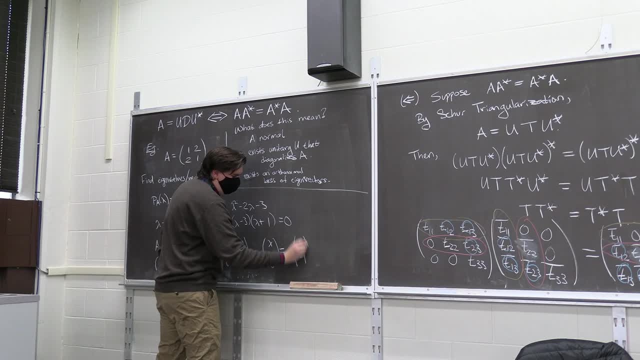 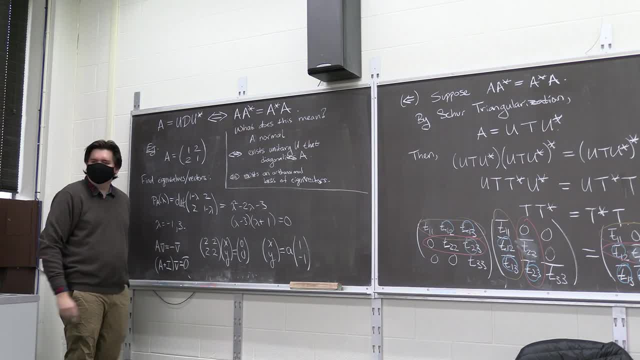 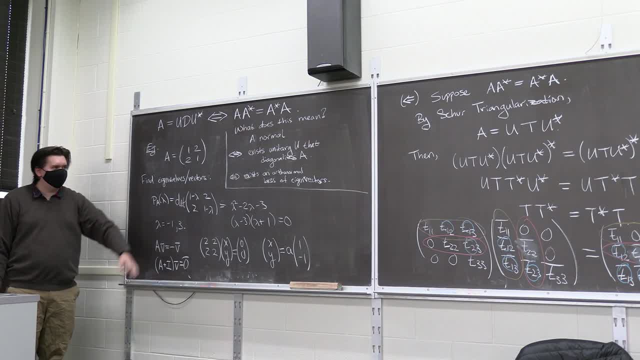 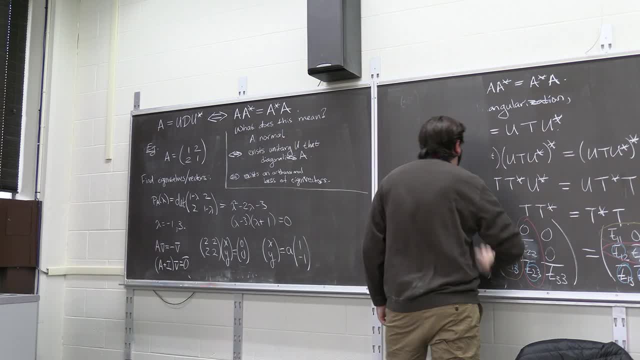 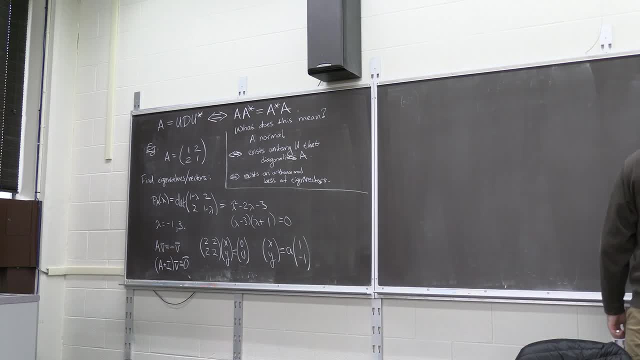 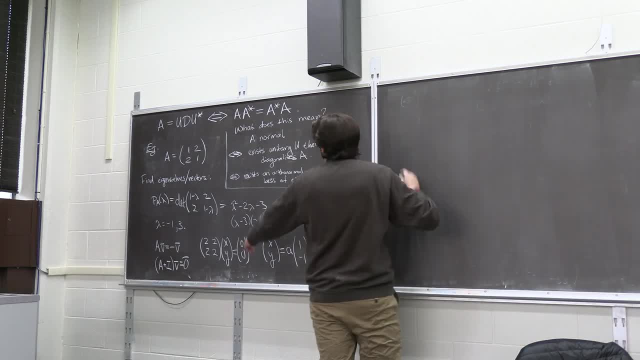 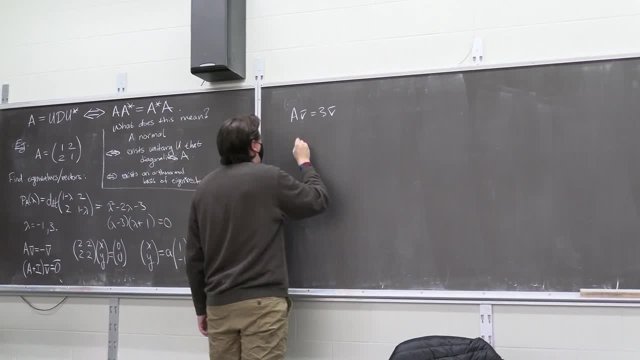 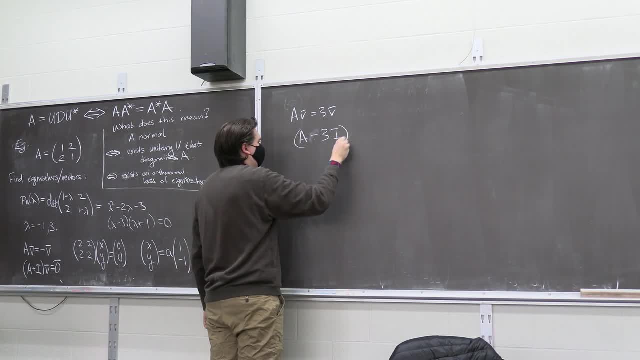 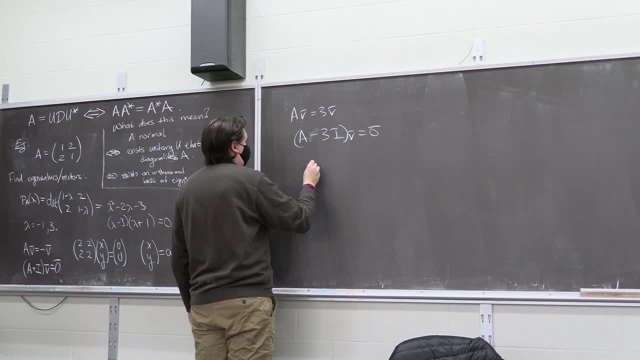 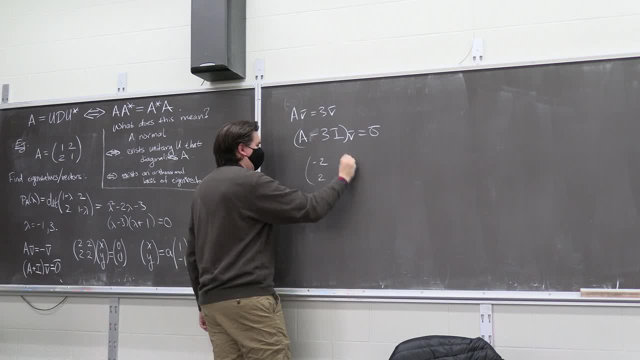 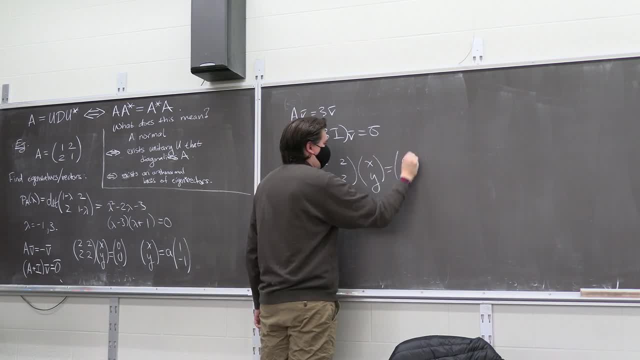 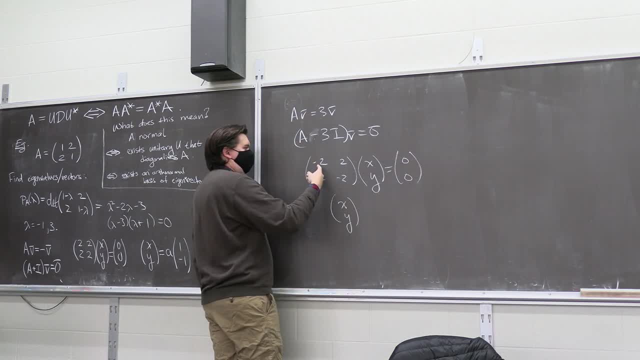 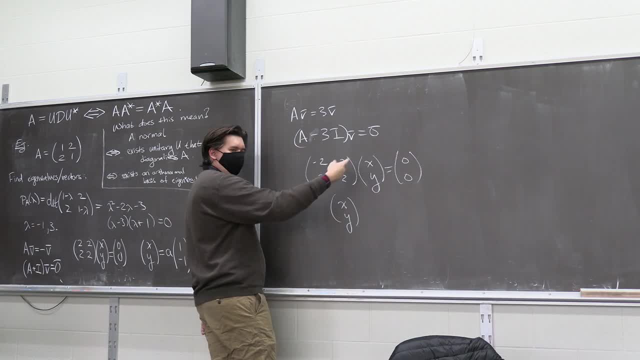 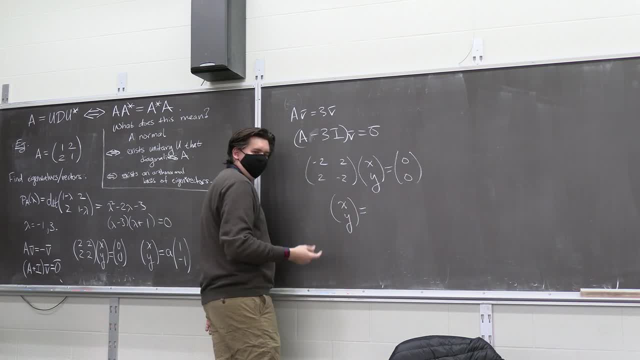 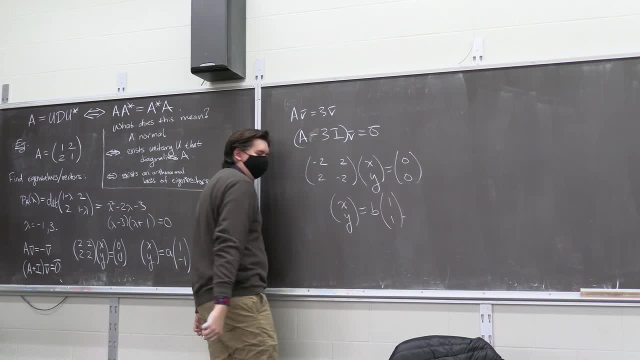 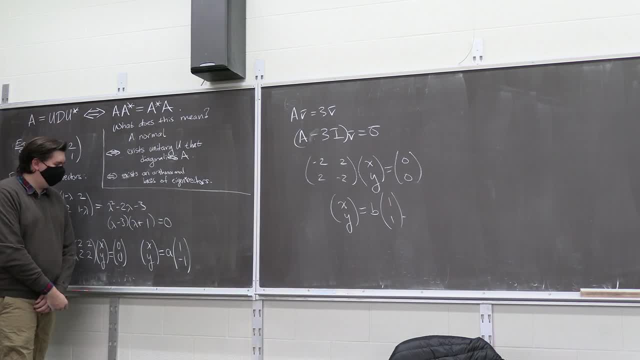 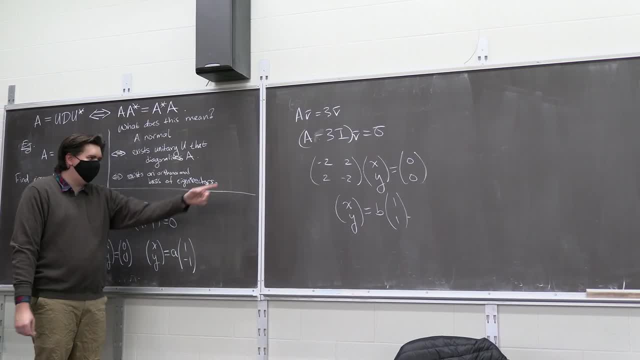 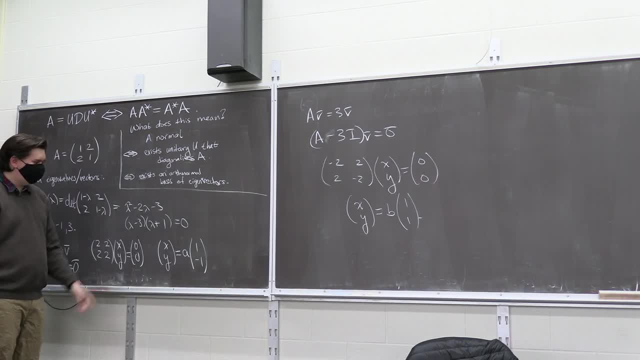 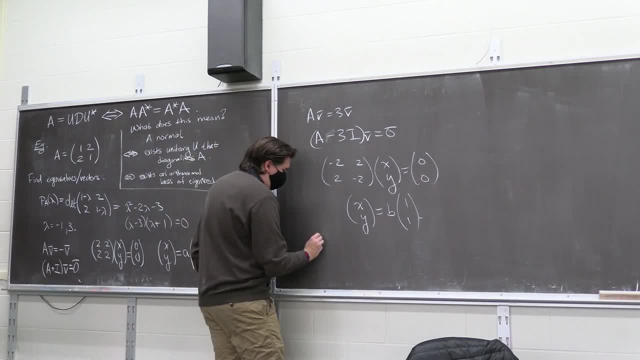 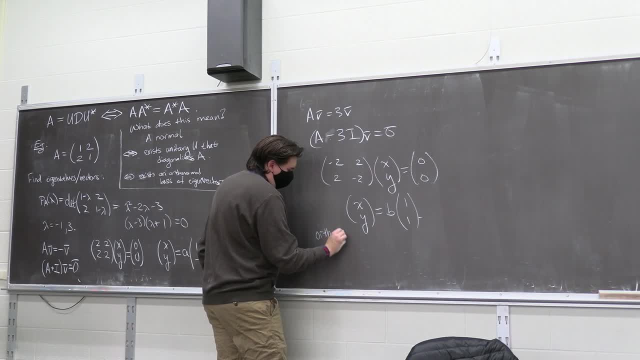 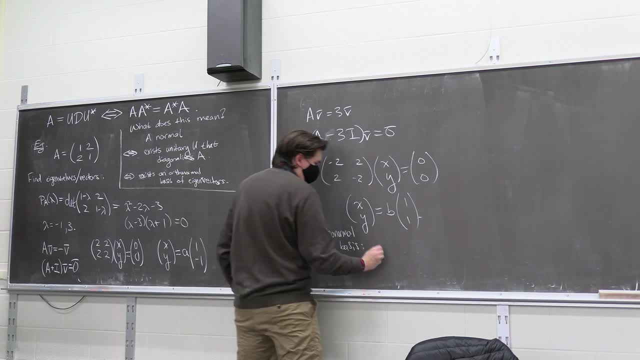 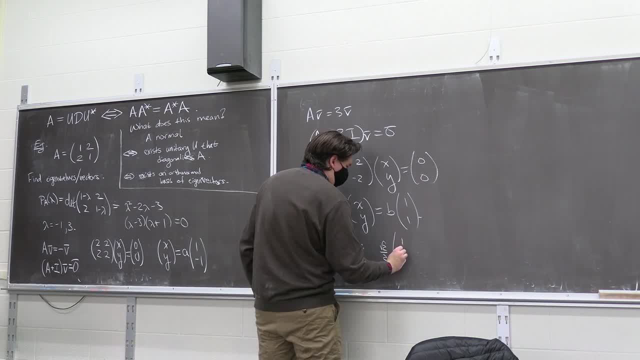 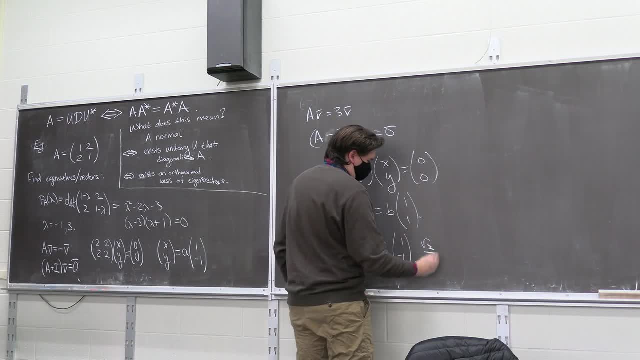 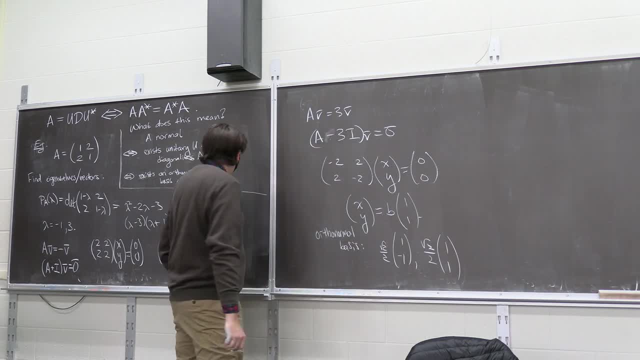 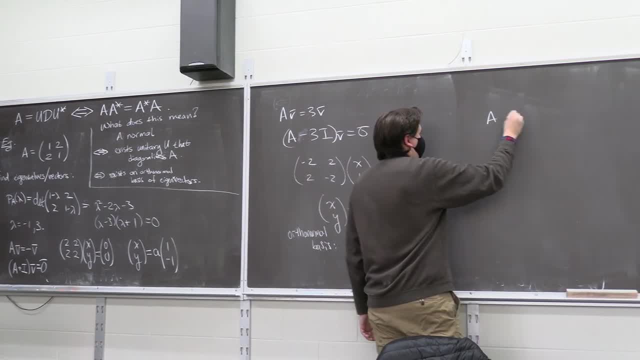 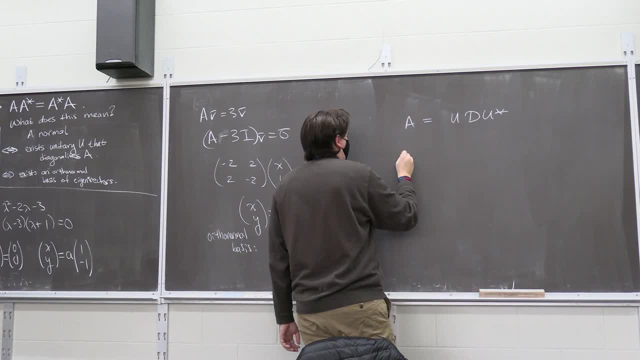 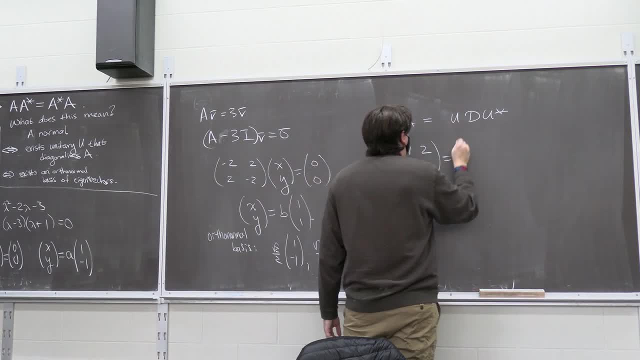 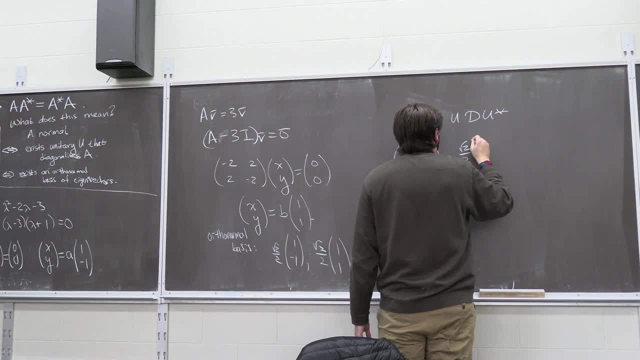 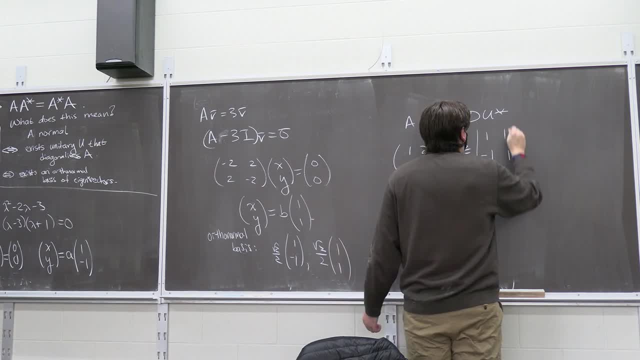 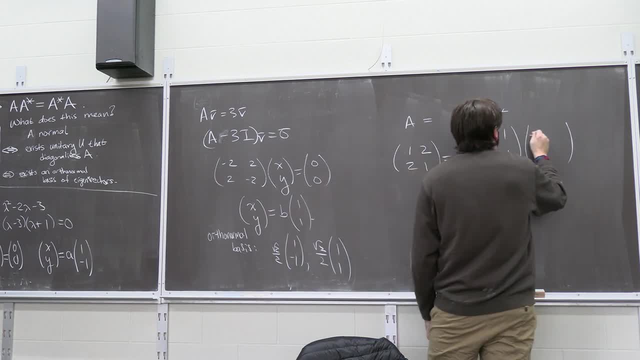 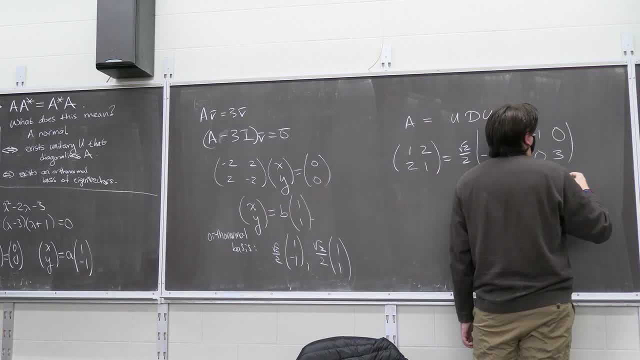 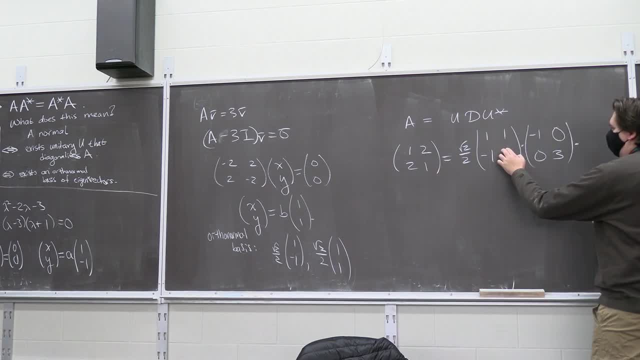 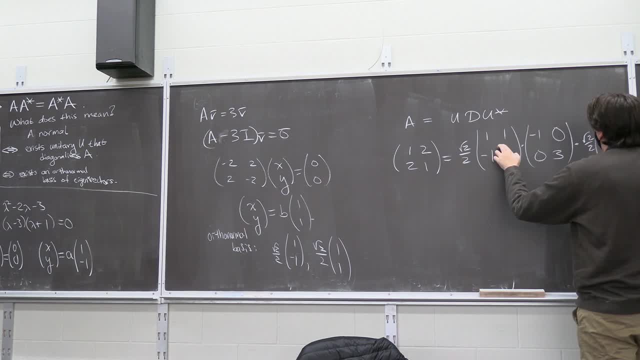 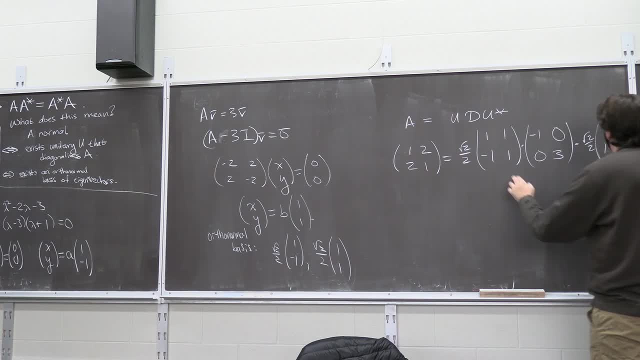 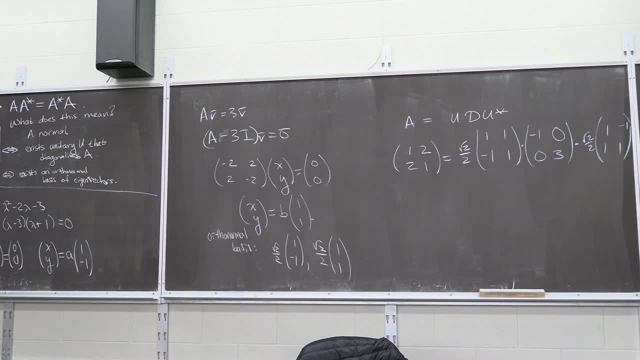